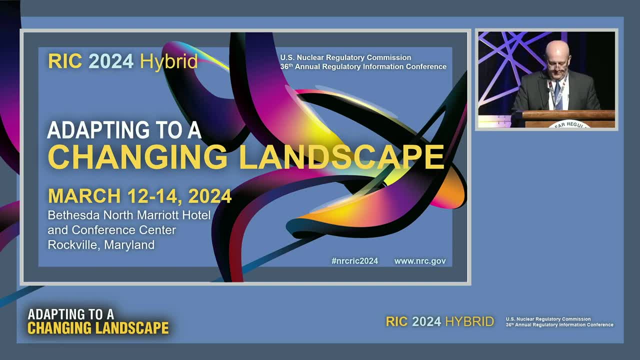 What I'd like to do is just do a quick introduction of our five panelists by name and organization, and I'll give a little more details. I introduce each one of them for our talk. So, from the Nuclear Regulatory Commission, we have Jason Piotr, who will speak first. We have Jorge Varnaes from the 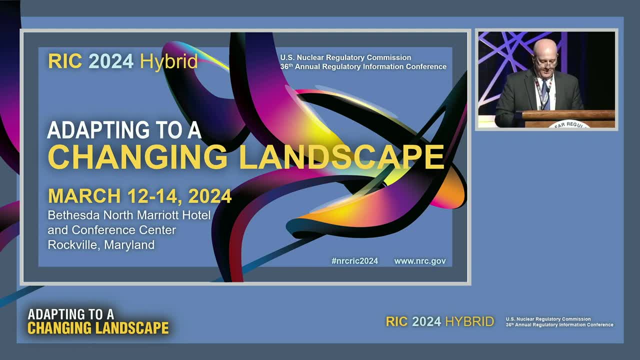 Department of Energy. We have Victoria Huckabay from the NRC, We have John Donaldson from Centris and we have Jean-Luc Luchon from our ASN, our French regulator, and he's one of our commissioners. I appreciate that. So let me start the presentation, as I said, with 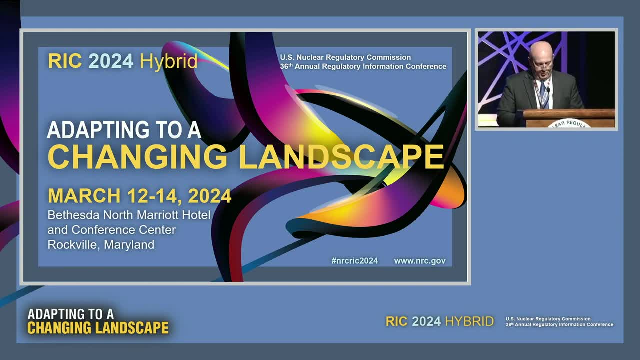 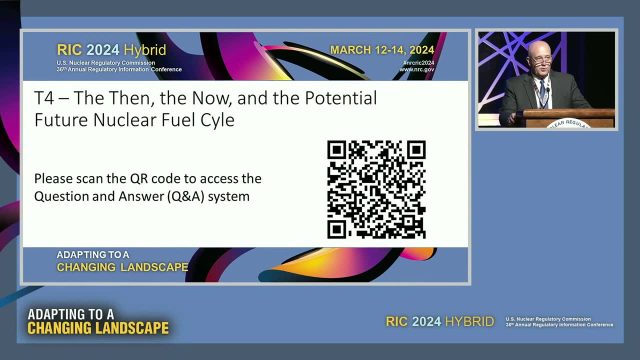 Jason Piotr. Jason currently serves as a Senior Program Manager for Accident Tolerant Fuel and Advanced Reactor Fuel Activities in the Division of Fuel Management in the Office of Nuclear Materials Safety and Safeguards at the NRC. He is also a Senior Mechanical Engineer and Technical 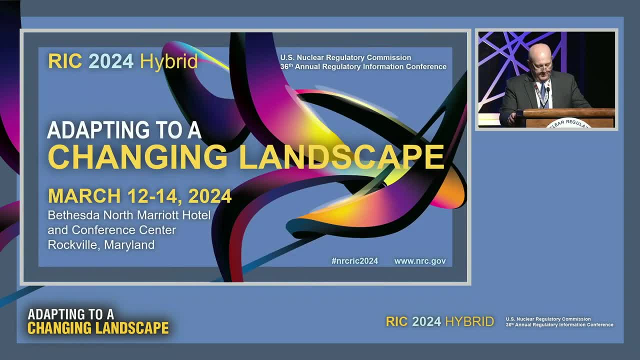 Reviewer for the Containment, Structural and Thermal Branch within his office. He started with the NRC in 2004, so he's just celebrated his 20 years at the NRC. He received a Bachelor Degree in Civil Engineering from the University of Iowa. 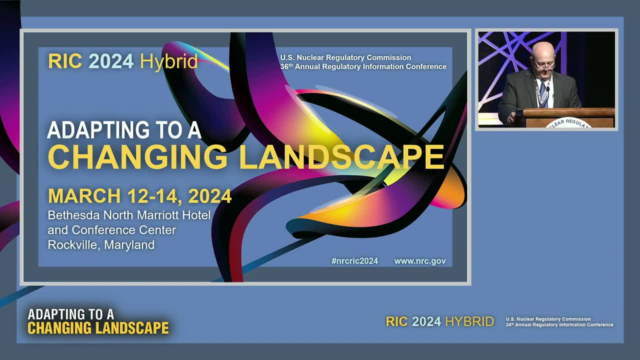 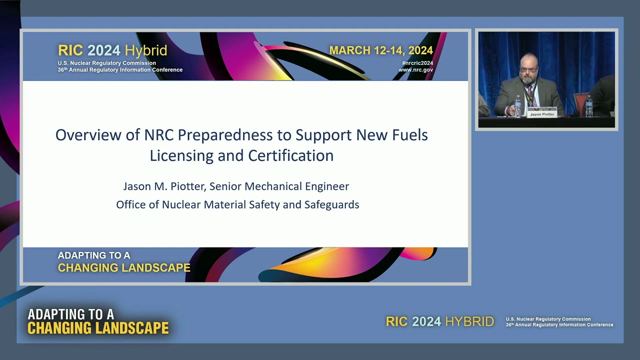 and a Master's Degree in Structural Engineering from Virginia Polytechnic Institute and State University. So let me turn to you, Jason. Thank you, John. Good afternoon everybody. I'm the lead-off hitter for this session. Hopefully everybody had a wonderful lunch and you're all refreshed. 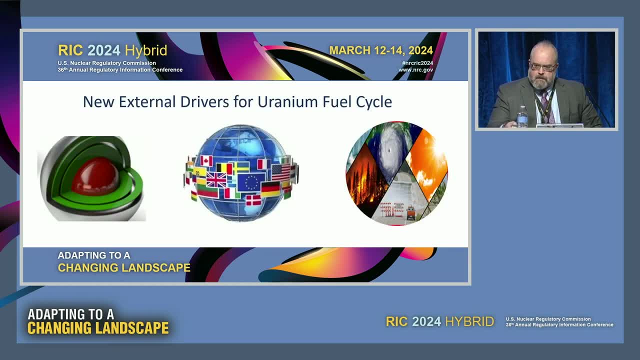 and ready to go for the afternoon. As you all no doubt well know, we're in a rapidly evolving environment that can have potentially significant and far-reaching impacts on the number and scope of new fuels licensing actions that are submitted to the NRC. We have seen significant interest in advancing nuclear power. 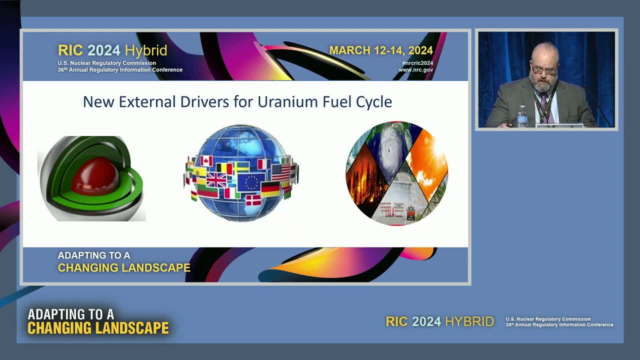 including what appears to be unprecedented bipartisan support for ATF and advanced reactors. as demonstrated at recent congressional hearings related to new fuels and, I think, any objective observer, this demonstrates that both legacy and accident tolerant LWR are a significant part of the NRC's mission. 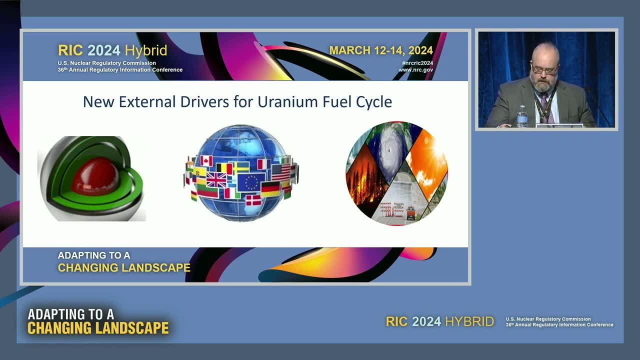 In addition, geopolitical issues and economic drivers may result in short-term or long-term supply disruptions, which has subsequently increased focus on enhancing and expanding the domestic fuel cycle for new fuels. A working understanding of these external drivers is essential to effectively plan regulatory workload. 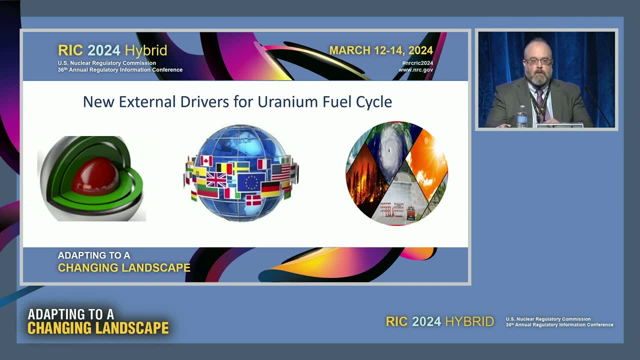 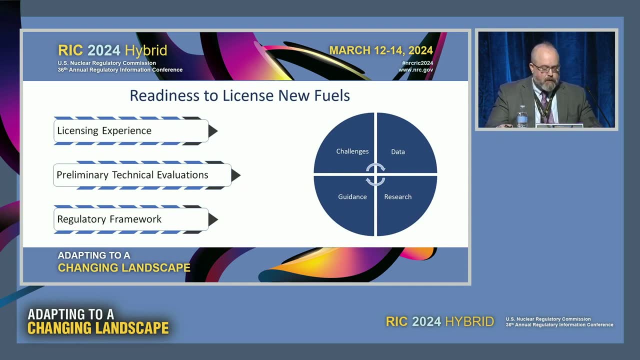 skill sets and resources at the NRC and within the industry. The NRC has been actively preparing for advanced reactor fuel reviews. by leveraging past licensing experience, performing preliminary technical evaluations and evaluating the regulatory framework and its applicability to non-LWR fuel designs, We have made significant strides. 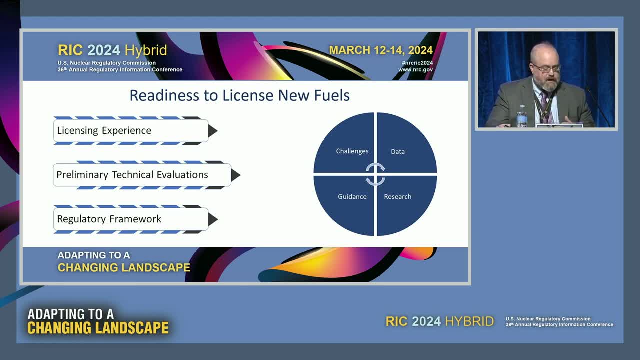 in our readiness to review applications for licenses and certifications for fabricating and transportation of near-term advanced reactor fuels. But a key point here has to be that we are not doing this preparatory work blindly or haphazardly. Our preparatory activities build upon this previous experience. we have licensing, enrichment and fuel. 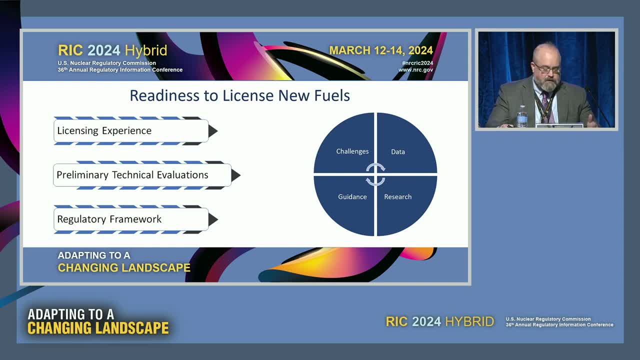 fabrication facilities at higher enrichments and certifying transportation packages, also with higher enrichments and novel fuel designs. We are actively gathering technical information for longer-term advanced reactor fuel concepts to support front-end fuel cycle licensing reviews. In addition, we are actively seeking technical information, including fuel performance data, which will inform ongoing evaluations of the regulatory framework and guidance for both the front end and the back end of the fuel cycle. 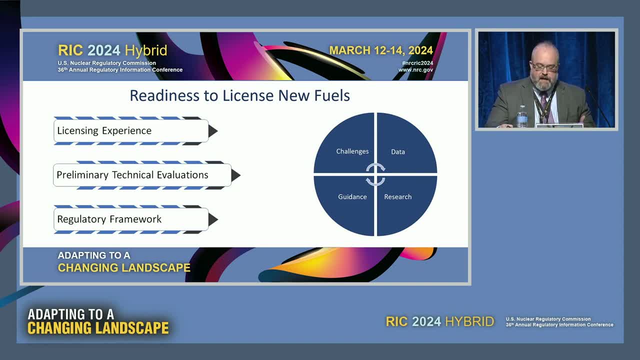 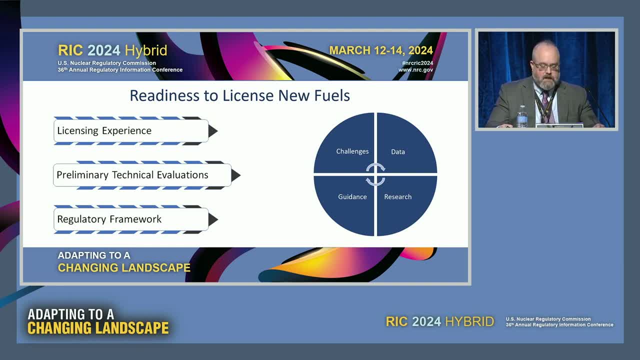 and fabrication operations, transportation and storage. While the NRC has not identified the need to make any changes to the regulations for near-term fuel concepts such as trisolar metal fuels, or longer-term advanced reactor fuel concepts such as molten salts, we must continue. 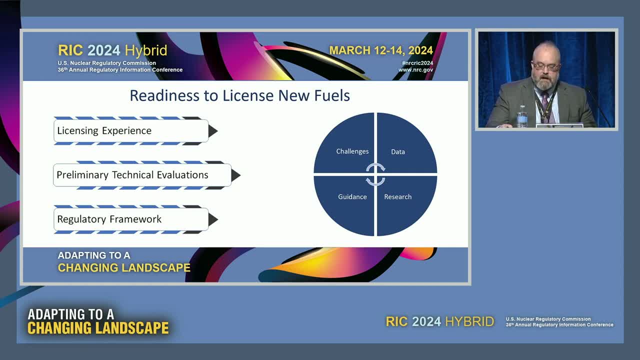 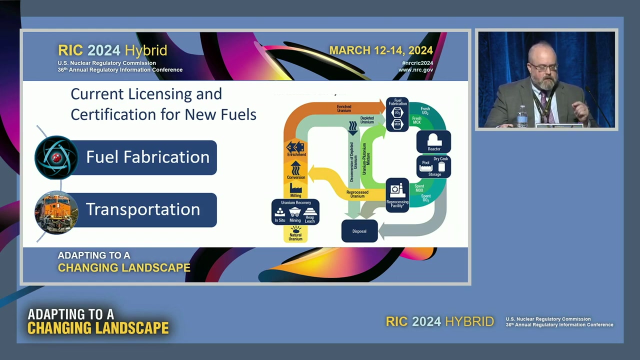 to assess our regulatory framework, to identify any challenge and or data needs, to ensure continued readiness to support licensing and certification. This must be done with a mindset of agility, active awareness and flexibility. So how do we test that? How do we test that? what we're doing, leveraging our past experience? 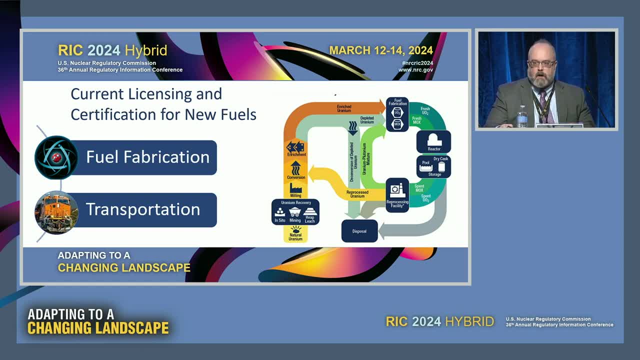 and our preparatory activities will actually be effective? How will it actually serve us well in the future And even in the now. we look at what we are actually accomplishing in the licensing and certification space, and it is a lot. Those areas of focus at the moment are fuel fabrication and precursor activities, such 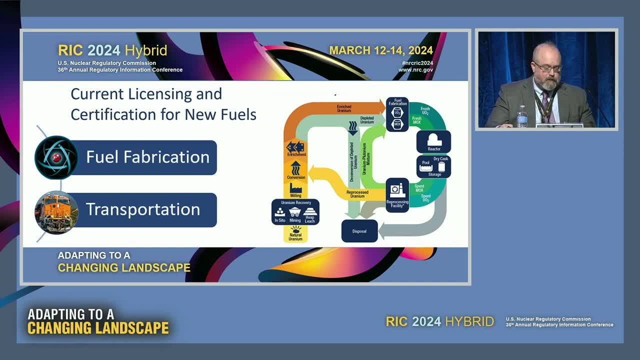 as enrichment, as well as transportation of feed material and fresh fuel for the front end of the fuel cycle. Consistent with our current practice, these applications for new fuel facility licensing, design certification of fresh fuel transportation and certification of fuel transportation packages, design certification of spent fuel storage gas and design certification. 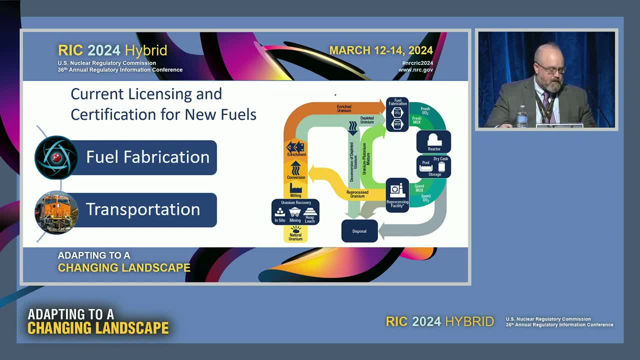 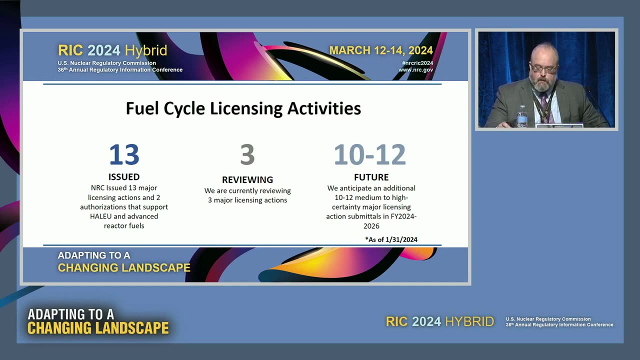 of spent fuel transportation packages must all demonstrate compliance with NRC regulations, such that new fuels can be safely managed in all areas of the fuel cycle. As I've already alluded to, the NRC has recently issued 13 major licensing actions and two authorizations. 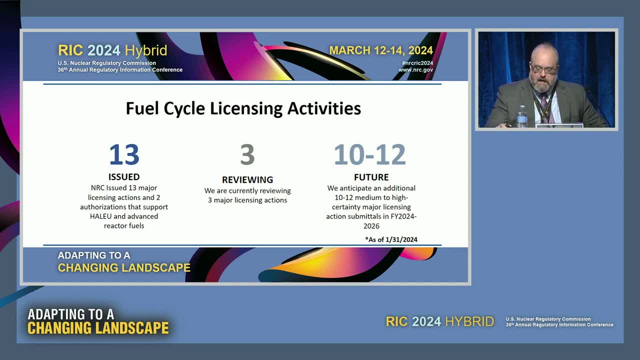 including licensing of the high assay low enriched uranium gas and industrial petrochemical- a low-enriched uranium demonstration at Centris American Centrifuge Plant, which you'll hear about later. We also issued an amendment allowing global nuclear fuels to produce accident-tolerant. fuel with increased enrichment up to eight weight percent. We've also approved several nuclear criticality methodology amendments to support accident-tolerant and advanced reactor fuels. We have met the need-by dates for all of these cases, all while performing thorough, transparent. 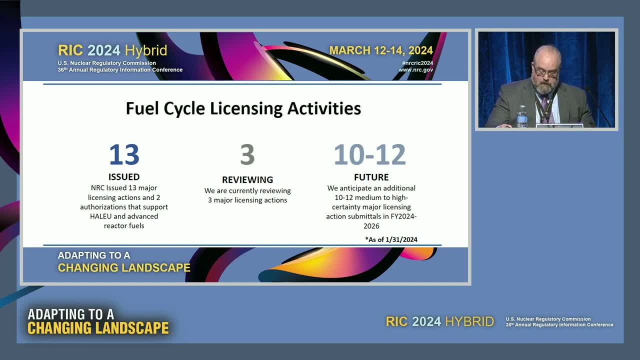 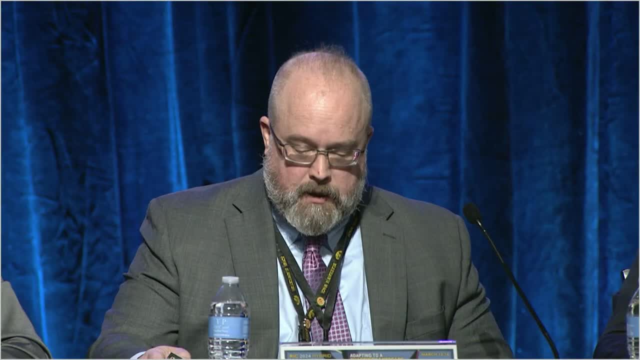 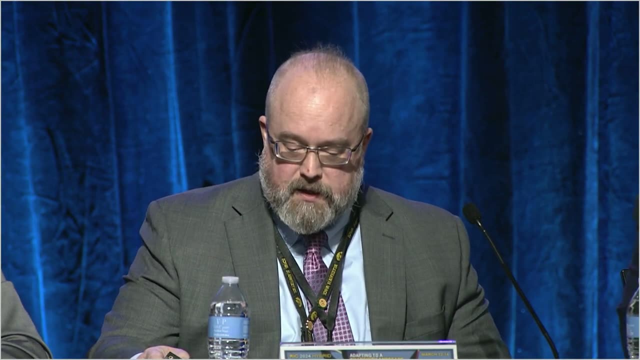 safety, security and environmental reviews. Currently we are reviewing three major licensing actions, including the TriSoX new fuel facility, And over the next three years we anticipate between 10 to 12 additional major licensing actions, including increasing enrichments up to 20 weight percent for enrichment facilities. 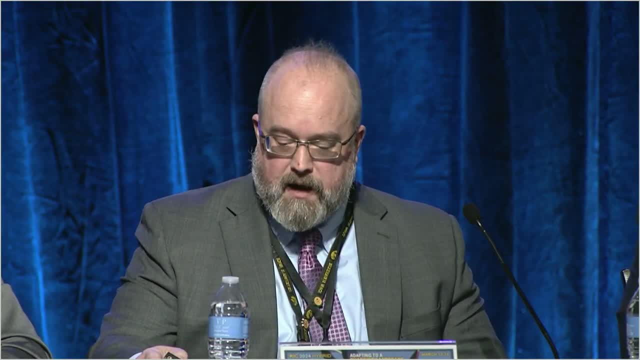 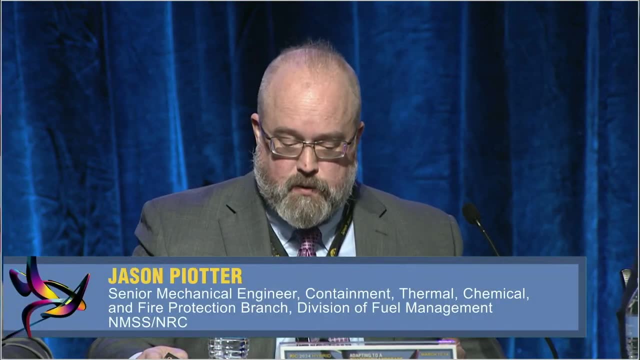 fabrication facilities and amendments for DOM blending of high-enriched uranium. In addition to these higher-certainty future actions, we have also approved a new fuel facility for the TriSoX. We have many informal discussions with potential enrichers, fuel fabricators and reprocessors. 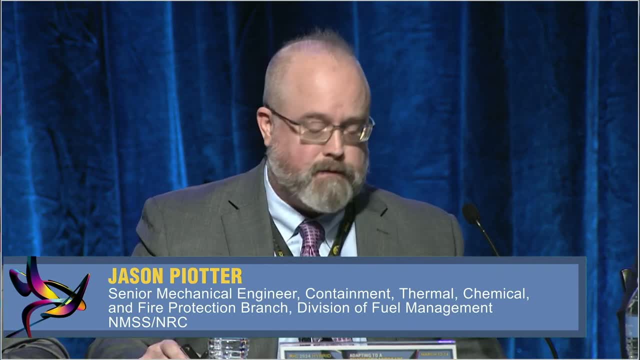 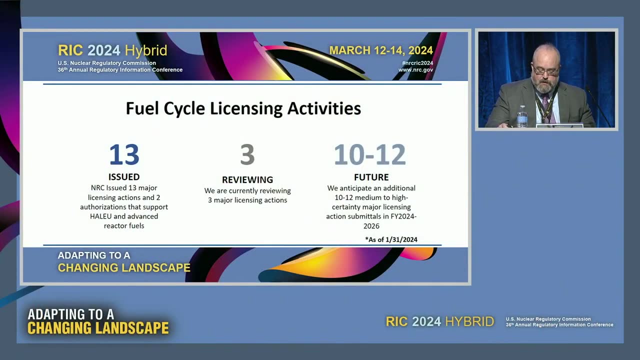 that would indicate sustained licensing activities for the near future. While the number of actions we have completed and anticipate are similar, the future actions are expected to be more complex, including completely new fuel facilities. As a result, we are paying extra attention to those future licensing actions to ensure 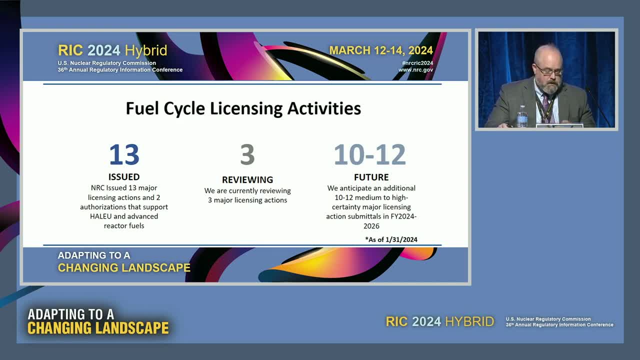 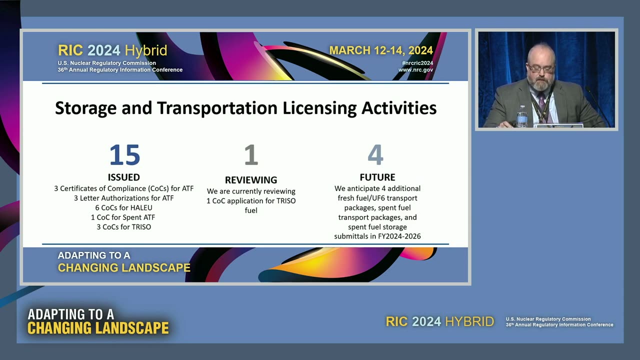 that we have the appropriate criticality. We have to make sure that we have the appropriate technical and technical skills and appropriate and necessary regulatory research and guidance identified in place when needed For storage and transportation. so to date, the NRC has issued 15 COCs and letter authorizations. 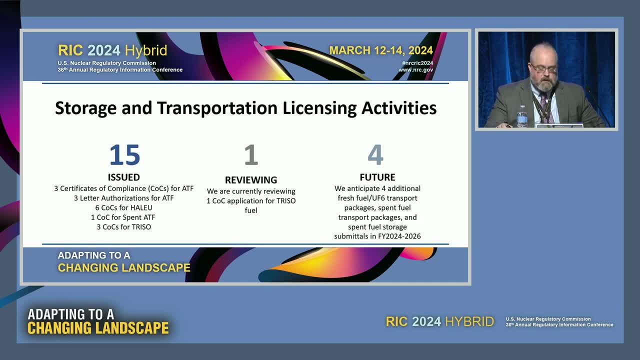 for transportation of accident-tolerant fuel, HALO, including UF6 and TriSoX fuel. Further examples for TriSoX fuel include the VersaPak and the Optimist. Finally, the DN30 transportation package, which allows for the transport of UF6 enriched. 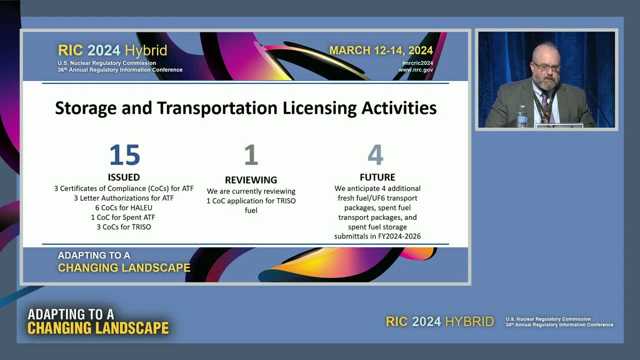 up to 20 weight percent was completed in March of last year and was a watershed moment for our activities in the new fuels arena. In the near term, we anticipate additional transportation packages for the back end of the fuel cycle, as well as storage applications related to ATF and advanced reactor fuels. 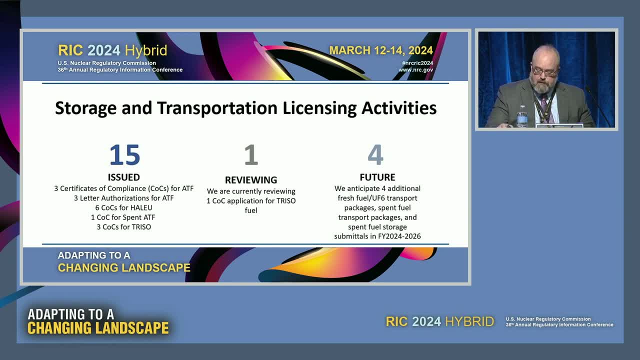 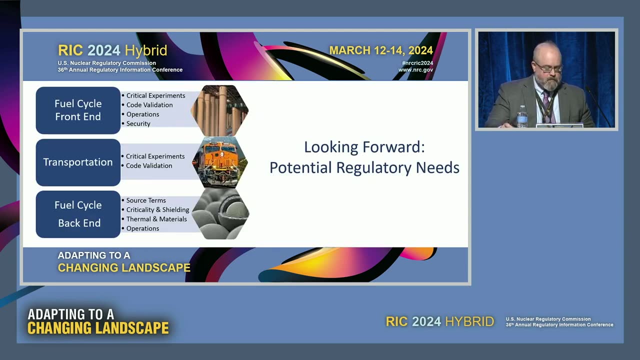 Early work has begun, both domestically and internationally, to evaluate any new technical challenges that may result from those waste streams and that may present new phenomenon that we have not encountered before with traditional LWR fuels. Looking forward, the NRC will focus on resolving technical issues as they become apparent. 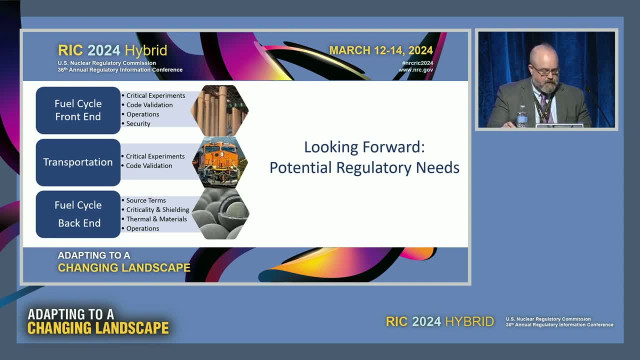 and seeking ways to enhance efficiency and effectiveness. With respect to the front end of the fuel cycle, there are potential challenges for HALO feed material and advanced reactor fuels, such as: limited critical experiments and benchmarks for higher enrichments. The additional availability of those critical experiments for the entire HALO range as 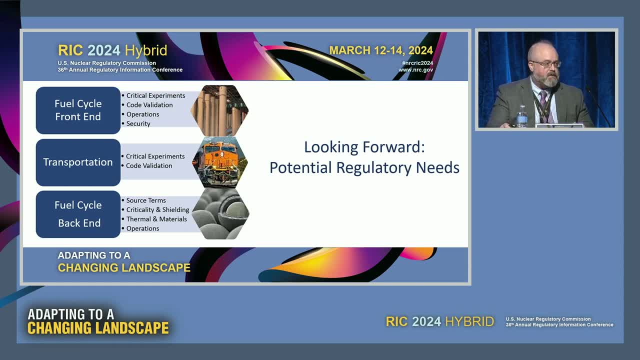 well as criticality benchmarks, would support the efficiency and effectiveness goals that I mentioned earlier. Similarly, there may be also operational challenges, such as chemical hazards or the security requirements for the possession, use and transportation of fuel. Thank you, Thank you. 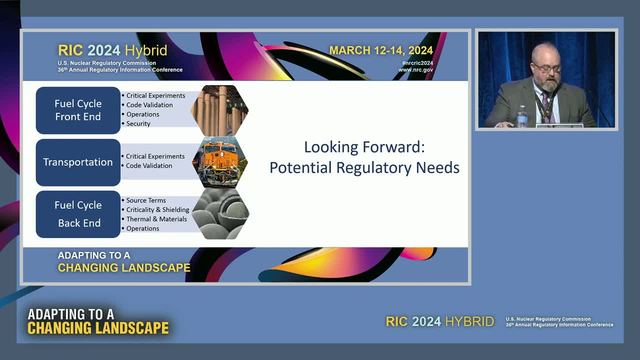 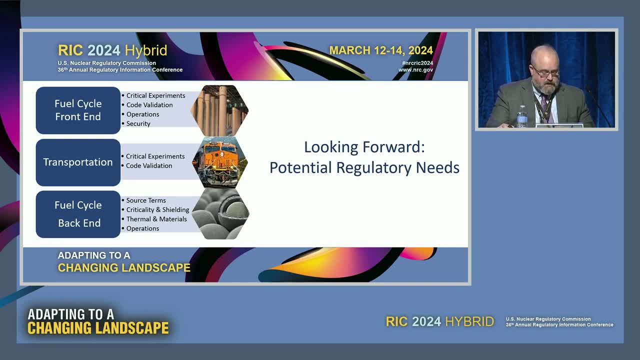 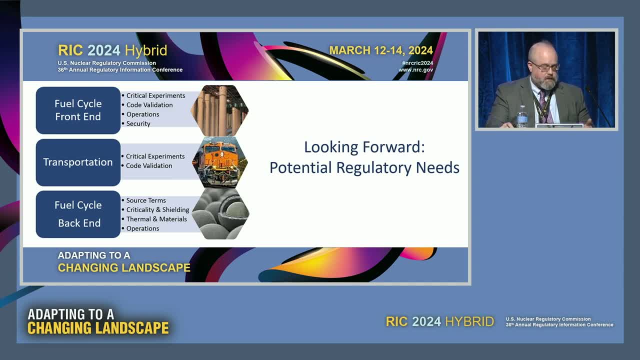 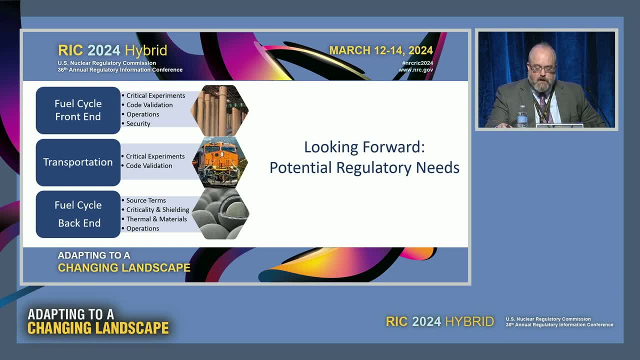 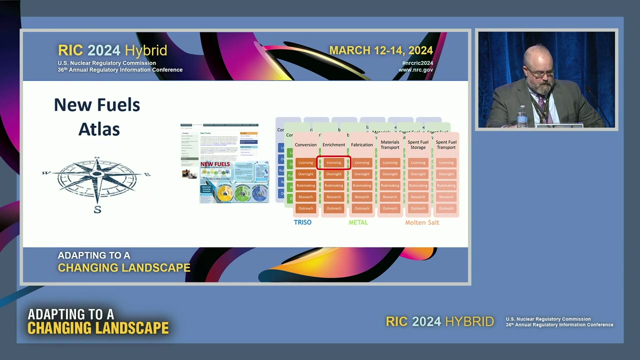 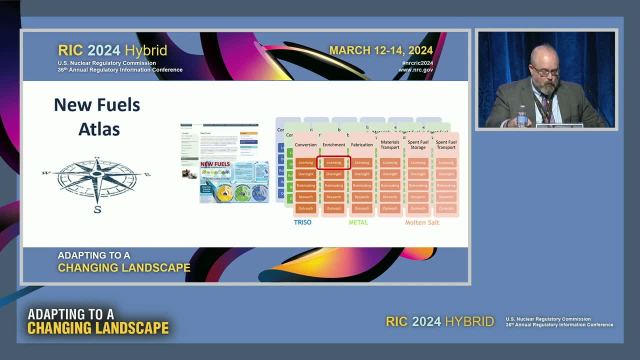 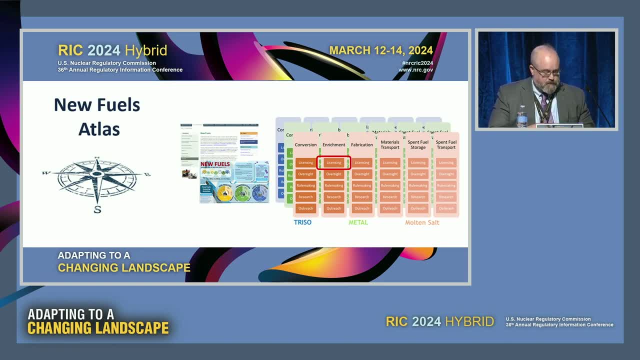 the NRC's continued readiness to regulate new fuels. The regulatory planner will consolidate information on current and future activities. It will cover the programmatic areas such as licensing, oversight and research activities associated with enrichment, fabrication and transportation of the different anticipated 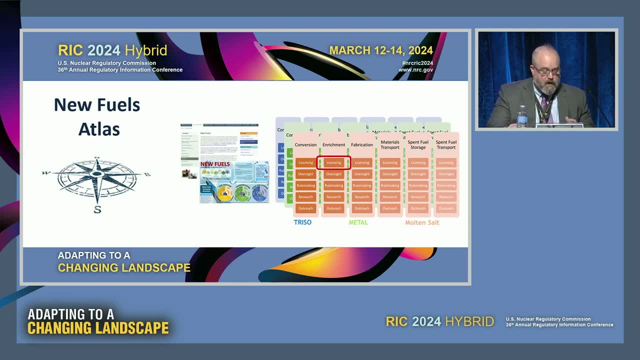 new fuel technologies. Obviously, I think everyone is aware, but in case you're not, this includes things like triso, metallic fuels and molten salt fuels. You'll hear more about this regulatory planner over the next several months as we get ready. 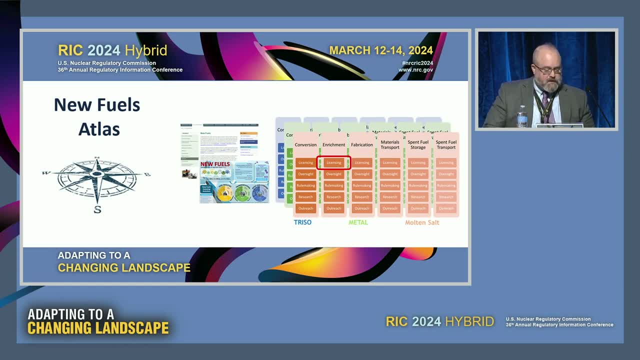 to deploy it. The Atlas is also intended to enhance our stakeholder communications through the use of an infographic, Part of which is picked. We hope to enhance public confidence in our abilities to effectively regulate these new fuel technologies by showing how our existing regulatory framework is able to accommodate. 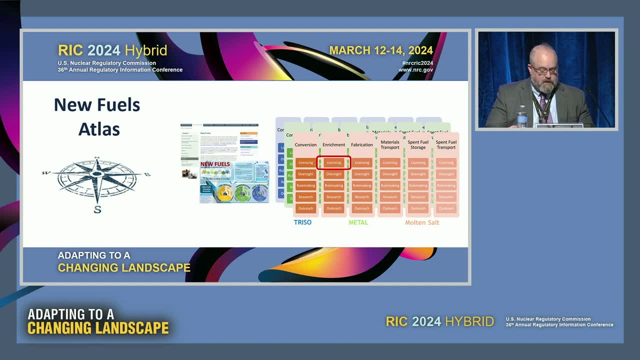 them. With respect to the communication tools, our intention is to enhance our stakeholder communications by providing a one-stop shop for everyone to find licensing and state of the industry information in a more user-friendly way. The Atlas is also intended to enhance our stakeholder communications by providing an 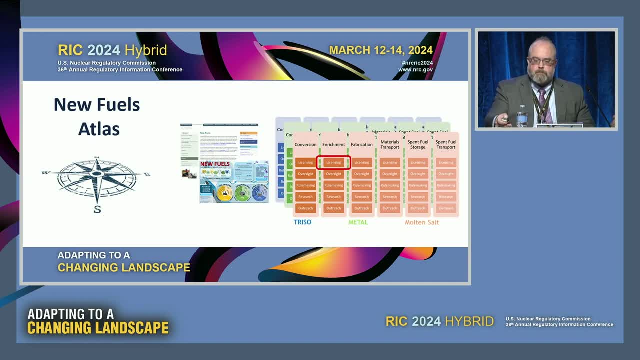 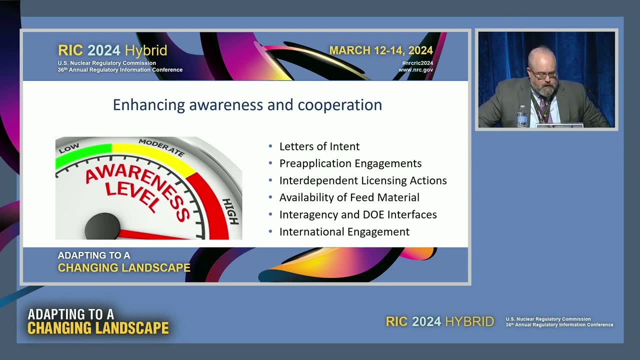 infographic. This includes things like triso, metallic fuels and molten salt fuels. We hope to enhance our stakeholder communications by providing a one-stop shop for everyone to find licensing and state of the industry information in a more user-friendly way. One last area I wanted to touch on before I close is how we go about maintaining and 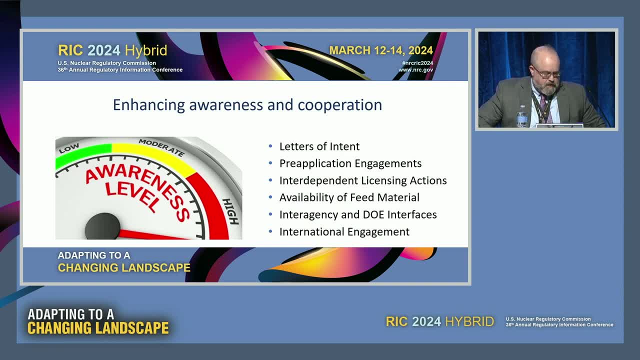 enhancing situational awareness and cooperation. I believe there are several areas in the Atlas that we should focus on, I think, to start with our day-to-day activities. this includes things like letters of intent, pre-application engagements and routine interactions with licensees and applicants. 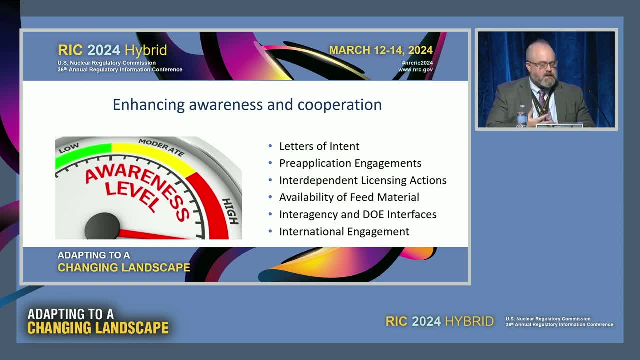 This helps us understand their policies, us understand their plans, their business needs, the external factors that they see could infect the impact and timing and scope of their submittals. I want to touch on the pre-application piece of this just for a second, because I think 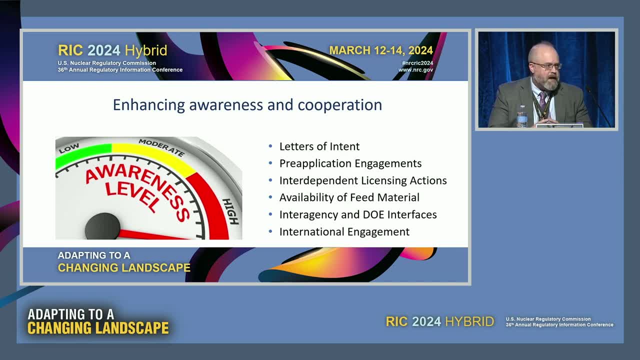 this is one of those areas which is probably the most underrated and most valuable tools that we have in the licensing realm. One of the points that I really want to make about this is that when we're looking at these types of activities, especially with new and novel technologies that we haven't seen, 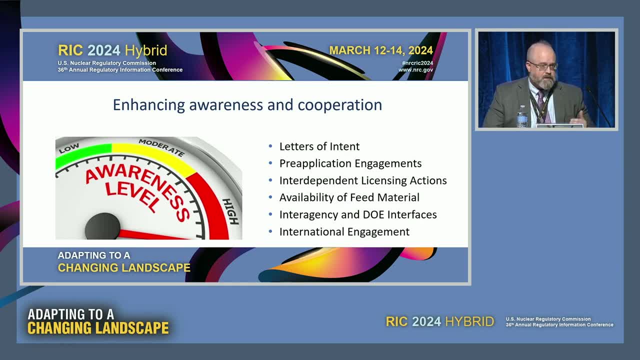 before. the place to sort of figure out what the path is going to be in terms of regulatory strategy is not inside the review cycle. Those things need to happen prior to the review cycle because the review cycle compresses a lot of what we do. 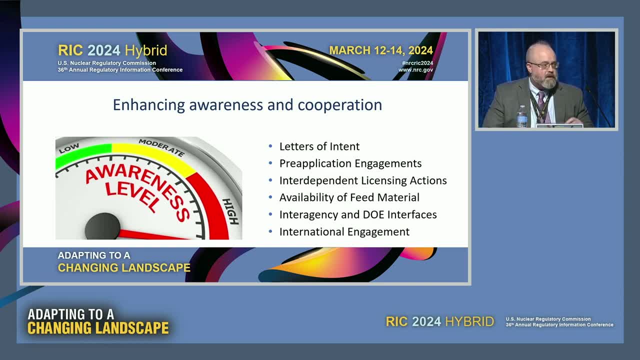 I can't stress this enough- that any applicant coming in that has something that's new or novel or something we haven't seen before or that we haven't looked at before, we haven't licensed before, we must have these pre-application engagements. It's absolutely critical to the success of not only the NRC but of the nation as a whole. 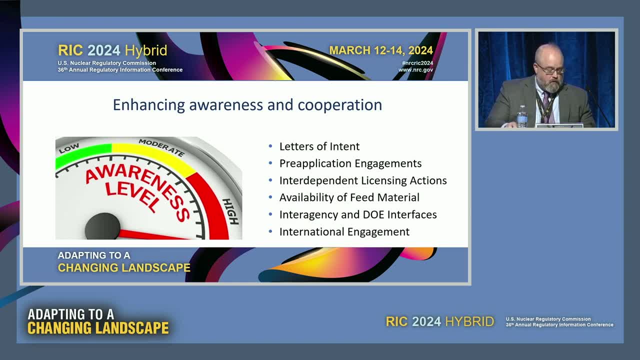 to be able to deploy these new fuels. Couple other points. Many of the licensing actions that will be needed at these facilities are interconnected, which means that we're going to have to make sure we understand what the flow of information is and how these licensing actions are going to come to us. 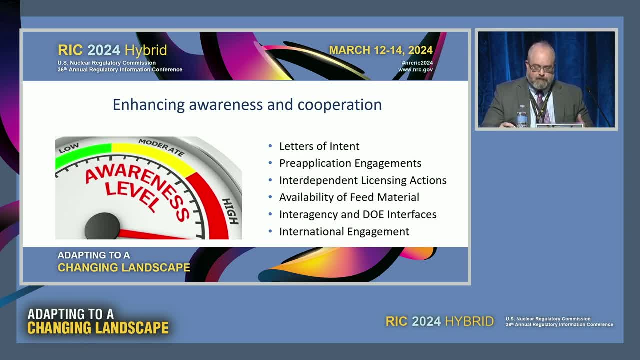 Such that we're able to plan for our resources accordingly. As I mentioned at the opening of the presentation, this rapidly changing environment is, and I think will be, the norm moving forward. So situational awareness and cooperation in areas slightly more removed from the norm. 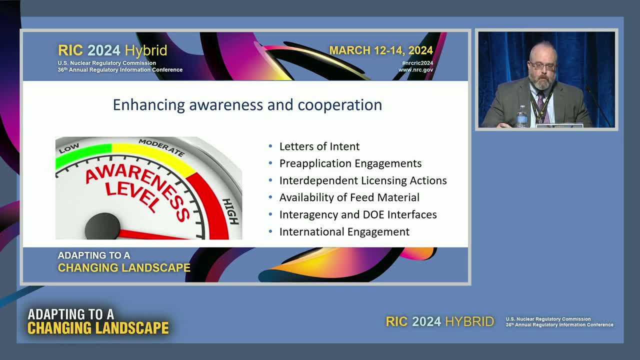 or from the day-to-day operations are going to be just as important as those day-to-day activities. This includes understanding what's happening with the uranium fuel supply itself and understanding where that How the industry is with that and where that feed material is going to be obtained from. 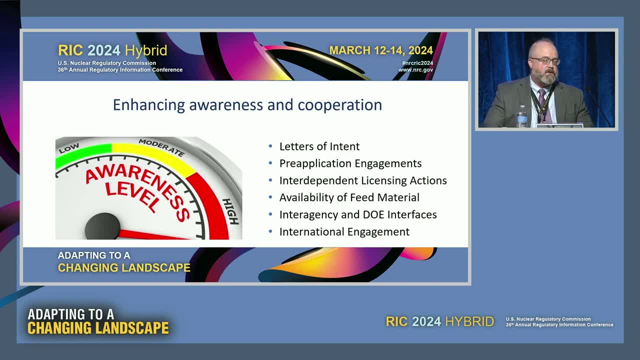 I think the other issue that we need to also make sure we pay attention to is what our other government partners are doing, Understanding the role and responsibility that they have and understanding the actions that they're taking for this new fuels, environment And, lastly, international engagement. 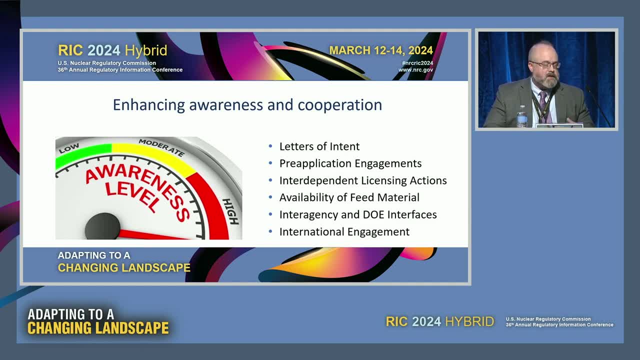 I would say that when we look at the international community, it is another backstop for us to be able to measure and assess whether or not we're meeting the needs with respect to new fuels and new fuels deployment. Final point I'd like to mention here is that, when viewed holistically, our current state 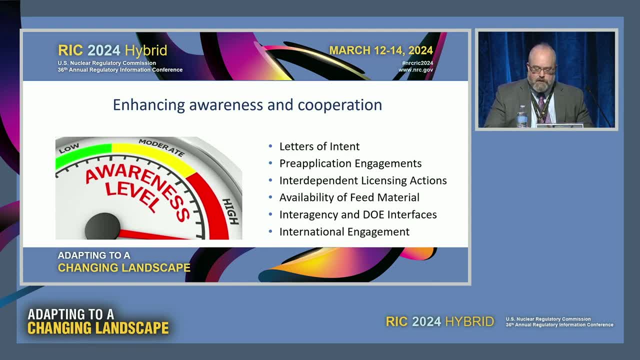 for licensing certification. our planning and preparation for the future and our proactive approach to understanding all facets of the uranium fuel cycle has positioned us well to modulate our workload, our workforce and our innovation risks and to make the best regulatory decision we can to protect public health and safety. 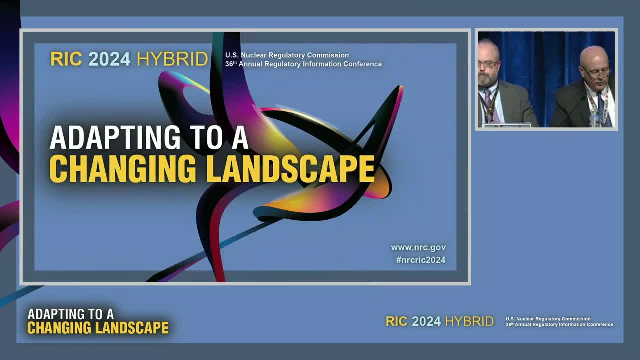 Thank you, MR, Thank you, Jason, Appreciate it. And one of your last couple points is a good lead in to our next speaker: Working and understanding where our partners are, both in the US government as well as internationally. And with that I'm going to turn to one of our partners at the Department of Energy. 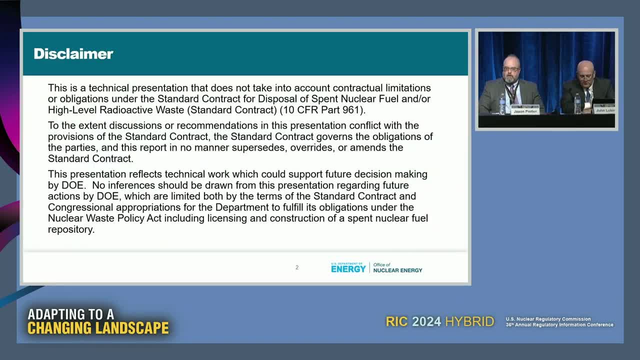 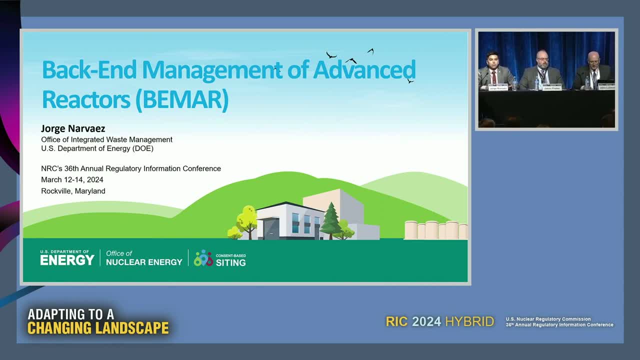 Jorge Narvaez, who is a general engineer at the US Department of Energy in the Office of Integrated Waste Management. in the Office of Nuclear Energy He leads the DOE He group tests with the technical analysis and considerations for incorporating small modular reactor and advanced reactor spend fuel into the waste management system. 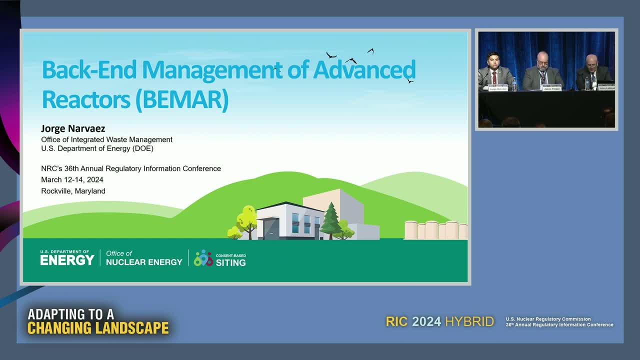 Prior to joining the Office of Nuclear Energy, Jorge worked as a project manager in the private sector, designing digital control systems for US and South Korean nuclear power plants. He has also served as a research associate for the White House Office of Science and Technology Policy. 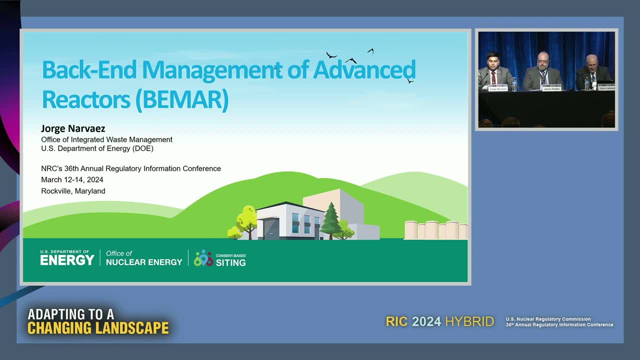 MR. Hello everyone. My name is Jorge Narvaez. I'm the National Technology and National Security Fellow at the Assistant Secretary of the Army. Jorge received his Bachelor of Science degree in Physics and Mathematics from Adelphi University and his Master's in Nuclear Engineering and Engineering Physics from the University of 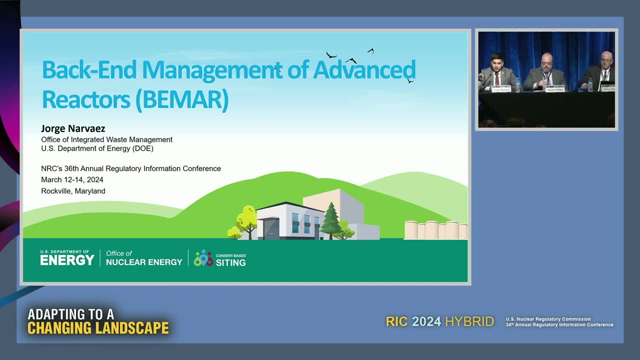 Wisconsin-Madison. Welcome, Jorge. Thanks, MR. Thank you, John. Good afternoon everyone. My name is Jorge Narvaez And in the next couple of minutes I'm going to be talking about some of the activities at the US. 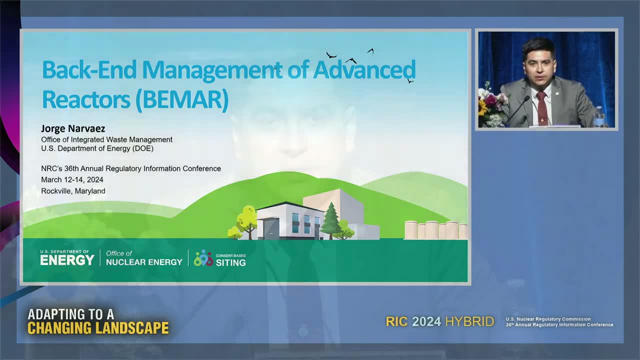 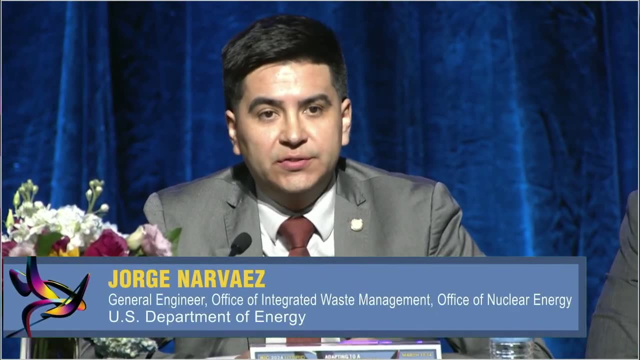 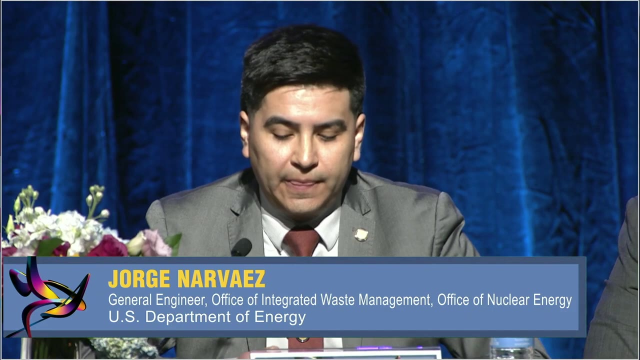 Department of Energy, Office of Spend, Fuel and Waste Disposition is doing to prepare to manage spend nuclear fuel from advanced reactors. This is just a disclaimer that more or less says that anything that I say to you today will not preempt anything that isn't a standard contract. 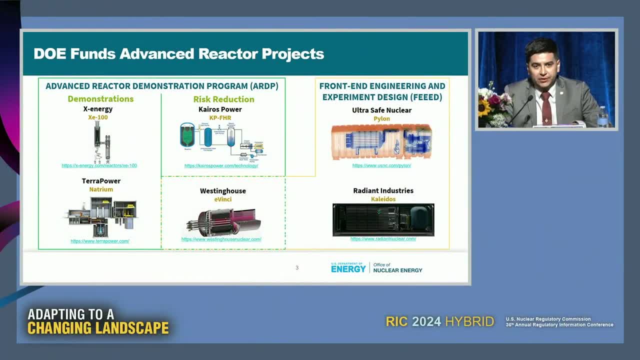 There is a lot of interest around the world and also here in the US, to deploy advanced reactors. The last time that I checked, there's around 20 advanced reactor designs from companies based in the US, And that's increasing every single month. 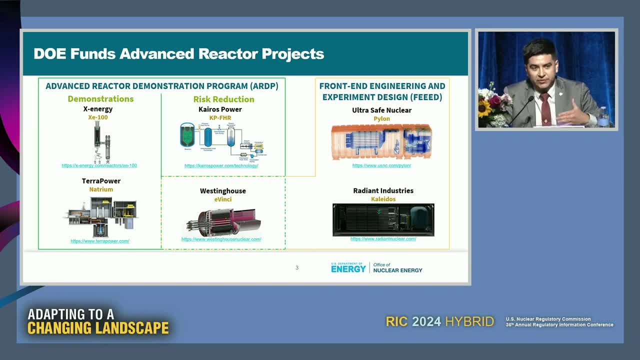 You see in the news, there's a new advanced reactor company proposing a new design. I want to highlight three companies here. Two of them are being funded by the Advanced Reactor Demonstration Program, which is trying to bring the X-Energy XE-100 reactor to the US. 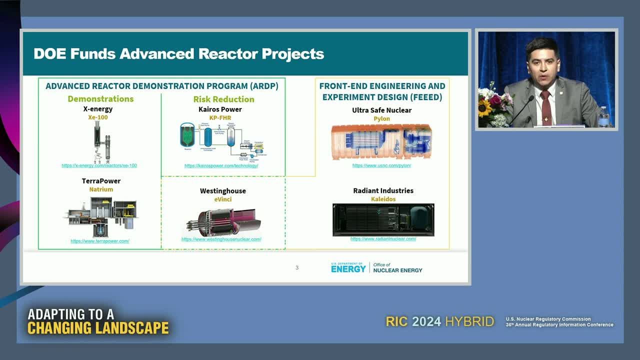 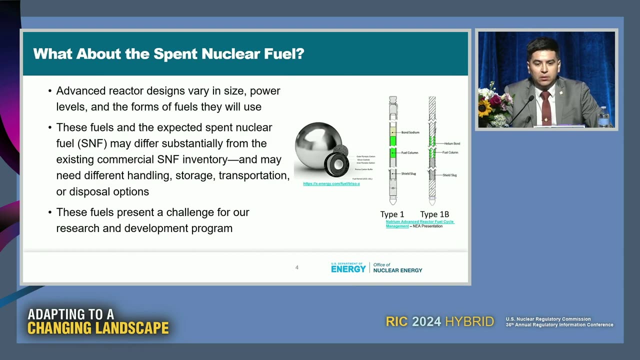 Department of Energy Office of Spend Fuel and Waste Disposition. I'm going to talk a little bit about that. And also Terra Powers, an Asian reactor for near demonstration, And also Kairos, which is working on the Hermes reactor facility in Tennessee. 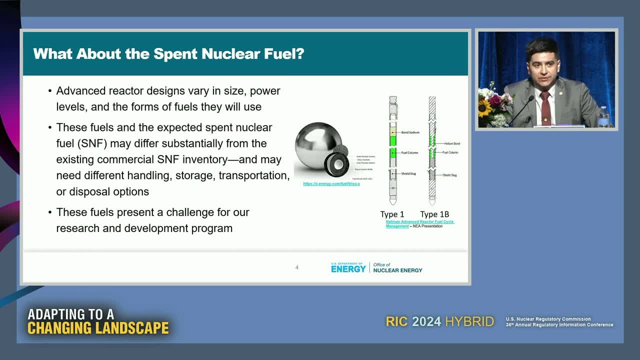 So there's a lot of advanced reactor interests. Many of these designs typically vary in the type of fuel that is being proposed to be used and the power levels. This is a challenge for the program. This is a challenge for the program that the Department of Energy is conducting, because 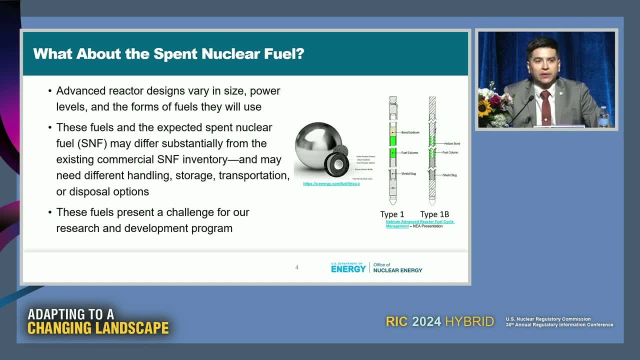 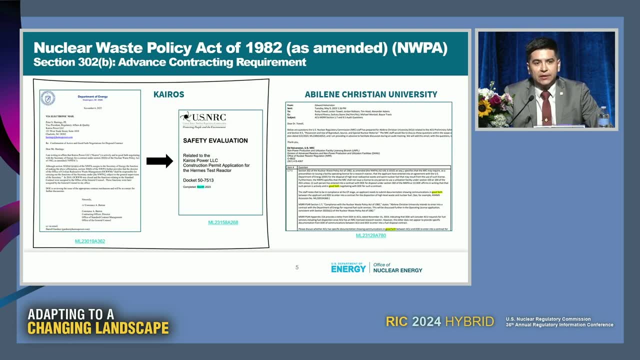 the spent nuclear fuel is going to differ from the current inventory of light weather reactor spent nuclear fuel. Under the Nuclear Waste Policy Act of 1982, the Department of Energy is responsible to take title and control of the spent nuclear fuel from the commercial utilities. 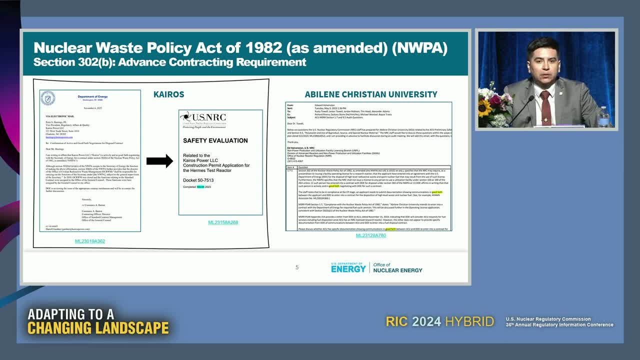 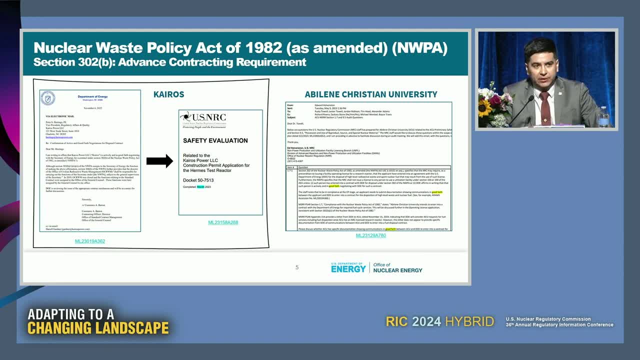 a license, typically two steps must be completed. For a construction permit, it would typically the NRC requires under the Nuclear Waste Policy Act it requires proof that the company has obtained a letter of good faith negotiating with the Department of Energy. And for an operating license, the NRC requires under the Nuclear Waste Policy Act that any 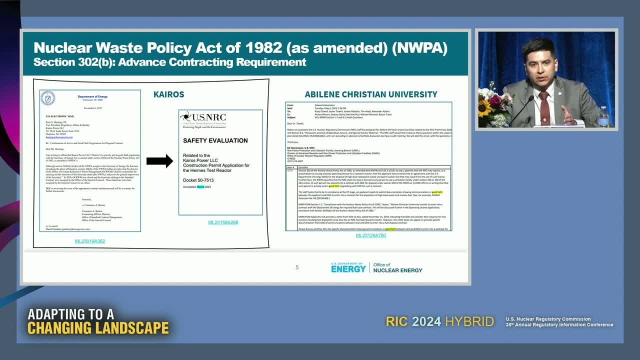 applicant shows proof that the applicant has entered into a standard contract with the Department of Energy for the Department of Energy to take title and control of the spent nuclear fuel for disposition services. In this slide I'm showing on the left two examples. These are publicly available documents that you can find on the NRC ADAMS website. 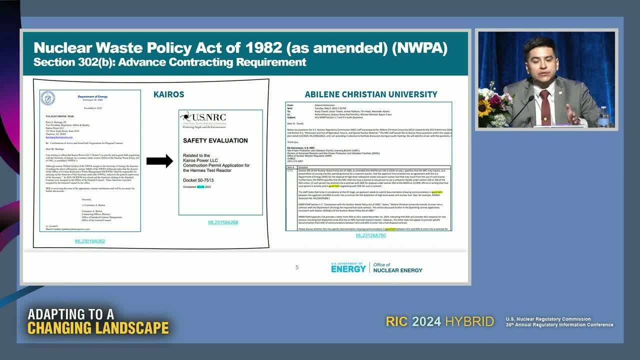 On the left side you can see all the way to the left. there is a letter Issued by the Department of Energy Office of General Counsel to Kairos Power saying that Kairos is engaging in good faith, negotiating with the Department of Energy. 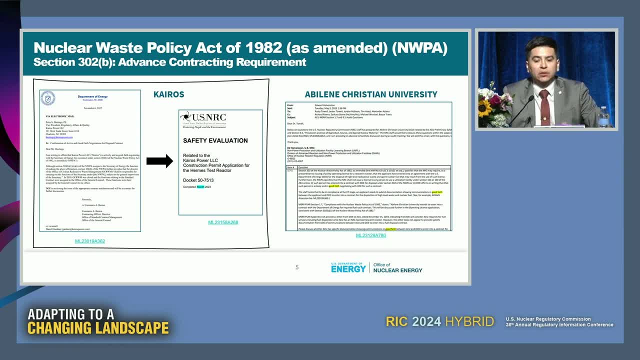 And this letter was used by the NRC as a checkmark to say that they fulfilled that requirement in order to get a construction permit. To the right side you see a letter from the NRC to Abilene Christian University asking Abilene Christian. 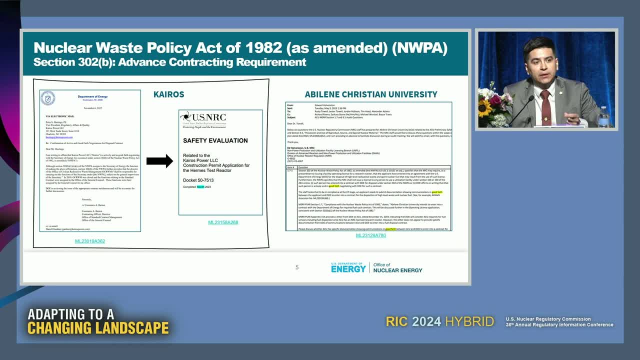 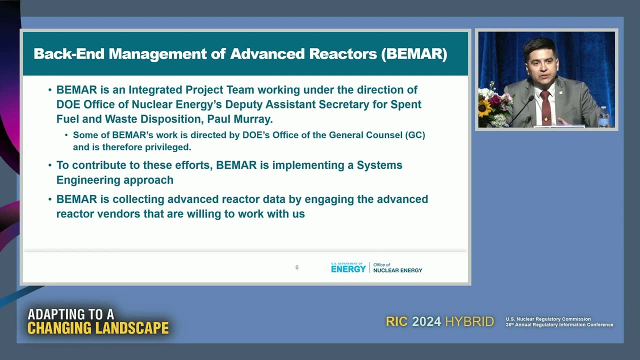 Abilene Christian University to provide proof that Abilene Christian University is engaging with the Department of Energy to obtain a good faith negotiating letter. So in the Department of Energy there are different activities trying to prepare to manage the spent nuclear fuel from advanced reactors. 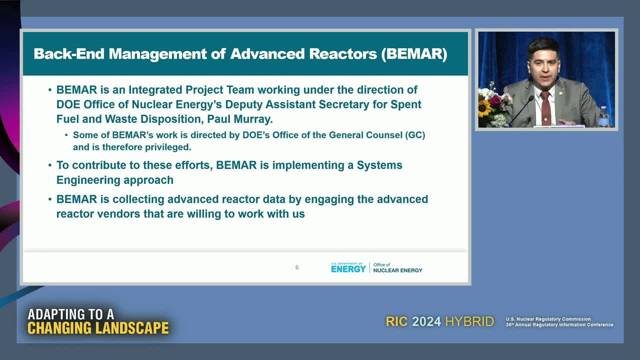 One of those activities is called the Backend Management of Advanced Reactor, or BMAR. I will be referring to BMAR. It's an integrated project team, which is more or less a fancy word for a working group that we use in DOE. 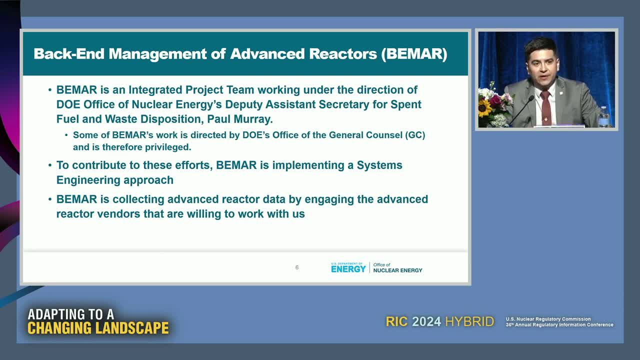 And it's being directed by the Deputy Assistant Secretary for Spent Fuel and Waste Exposition, Paul Murray. But I do have to mention that some of the work that we are doing in BMAR is also being directed by the DOE Office of General Counsel. 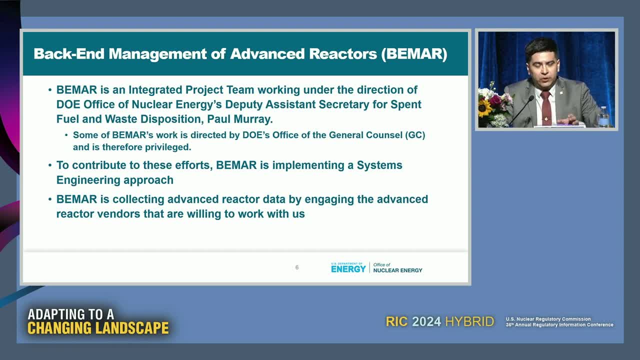 For details. Thank you. So for the BMAR effort, we are using a systems engineering approach to divide the work into a system of systems, if you will, And one of the main objectives, essential work, of the BMAR team is to collect and consolidate. 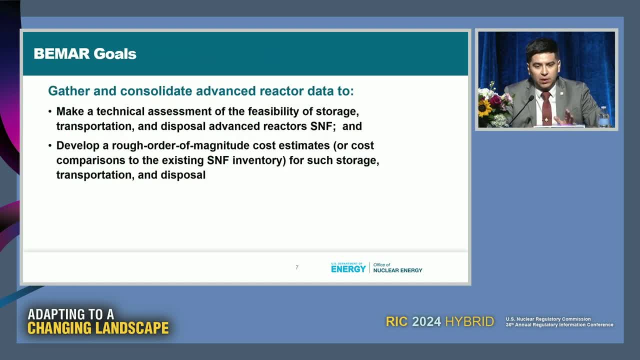 data from advanced reactor vendors To do the following two things: First is to make a technical assessment on the feasibility of storage, transportation and disposal, And this may include doing some tests and configurations if it's necessary. The second is to make a technical assessment on the feasibility of storage transportation. 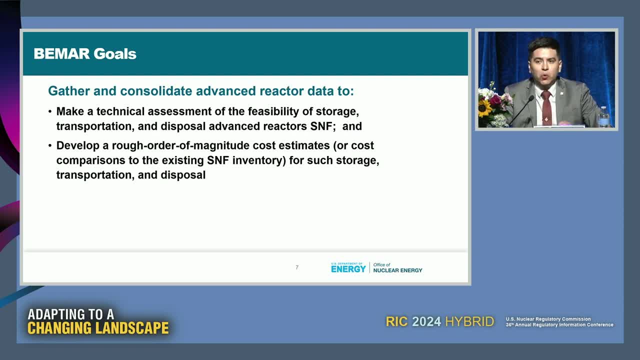 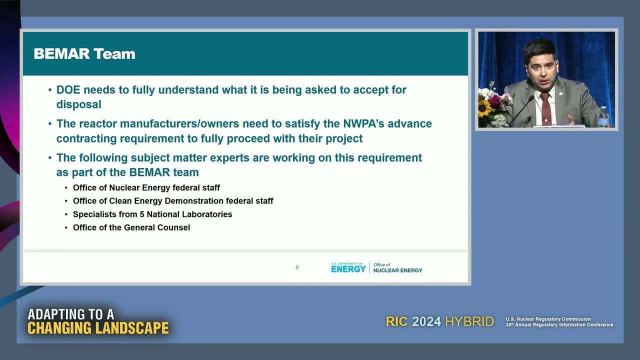 and disposal, And the second one is to develop a rough order of magnitude cost estimate and compare that to the same activities, but for light water reactors. The reason why we're doing this is because eventually, under the Nuclear Waste Policy Act, DOE is going to take title of the spite nuclear fuel. 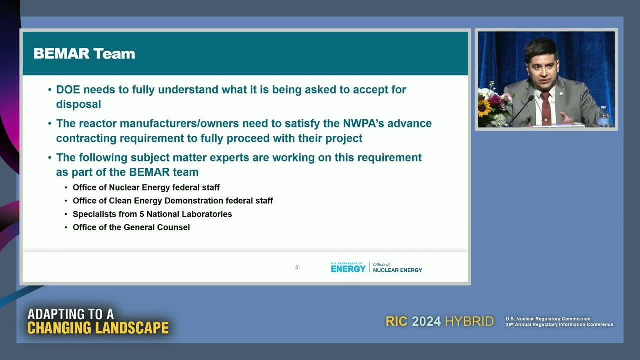 So DOE needs to understand what it needs to dispose of eventually. However, at the same time, the advanced reactor companies need to know what they are doing So they can do their job. So what we're doing now is in order to make a tactical assessment on the feasibility of 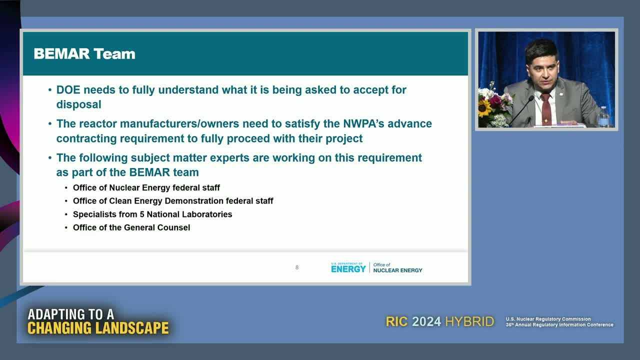 the question of what we're doing, But one of the things that we're doing in this idea is that we're taking this policy to the upper left corner of the graph. need to understand the requirements that they need to satisfy under the Nuclear Waste Policy. 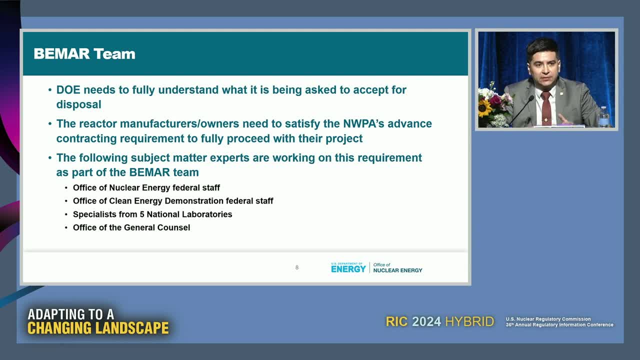 Act. In the BMR team, we assemble a team that is composed of different offices. So we have the Office of Nuclear Energy, which is the office directing this work. We also have federal staff from the Office of Clean Energy Demonstrations. We have experts from five different national laboratories. 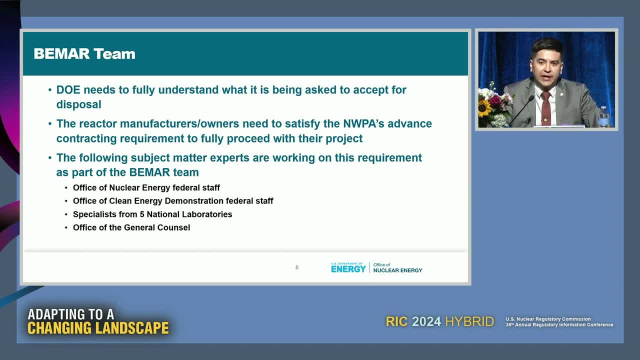 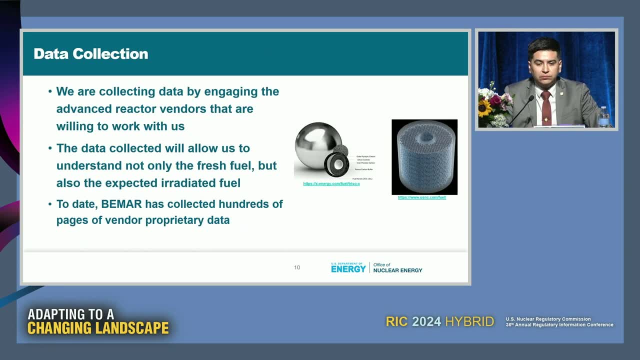 We also have a collaboration with the DOE Office of General Counsel. These are some of the advanced reactor vendors that we're working with And I mentioned before, at the very center of our work is a data collection effort. We are working with any advanced reactor vendor that is willing to work with us. 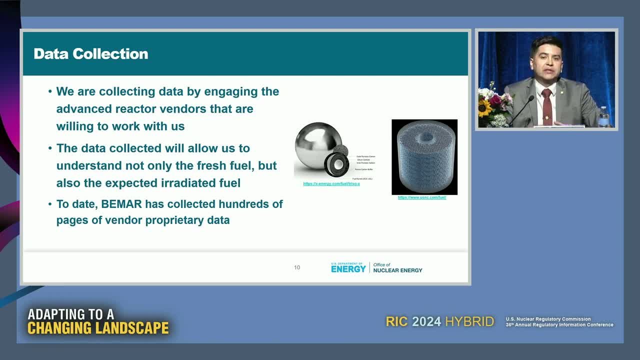 The data that we collect is not only going to help us understand what the field looks like before it goes inside the reactor, but also how it looks like after it comes out of the reactor. To date, we have collected hundreds of vendor, proprietary and expert-controlled data. 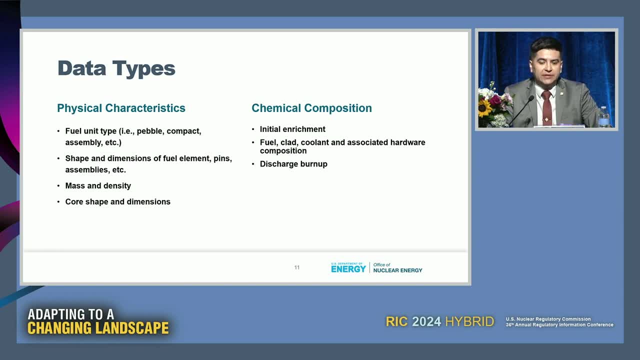 In the next few slides I'm going to be talking about the different types of data that we collect. So we are very interested in being able to characterize the data. so that requires DOE to understand how the field looks like. So we're looking at data. 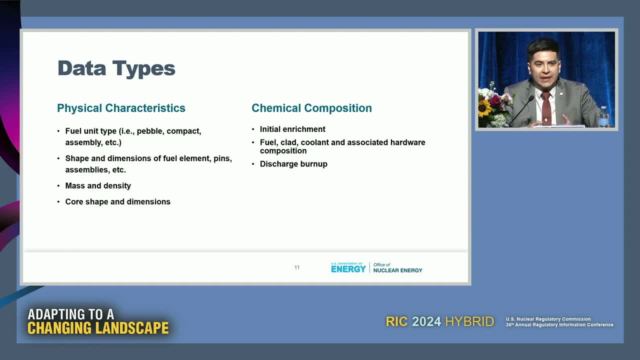 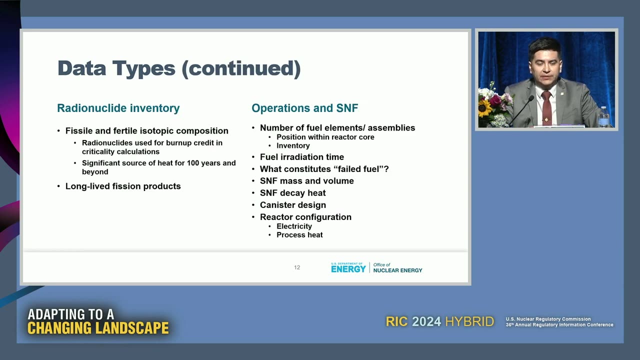 We're asking the vendors questions about the volume, the mass, the density of the field For the fuel, for the chemical composition. we're looking at the initial enrichment and any remaining enrichment after it comes out of the reactor burn-up, other types of data. 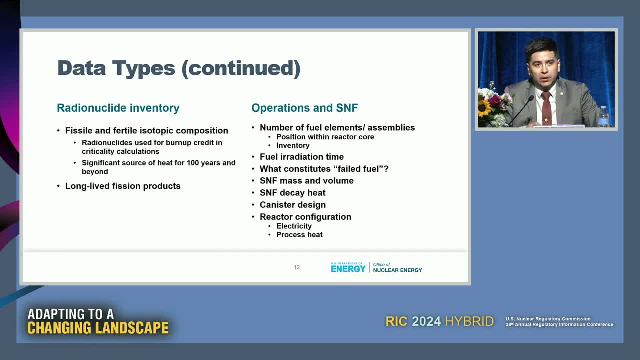 that help us manage for storage, transportation and disposal includes looking at the composition of the fissile and fertile material, any long-lived fission products and also interesting data points that also help us plan accordingly. Thank you, Thanks, Bill, Thank you. 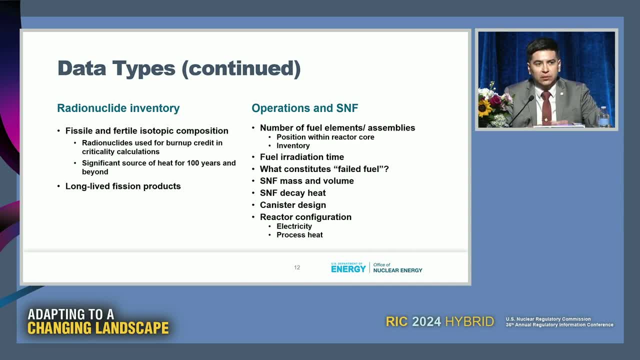 So let me say that the last thing that I will be showing is I will be speaking to our panel and I will be telling you a little bit about the lifecycle and what we've been thinking about. I will be talking about the future of fuel- each fuel and its internal****—but basically. 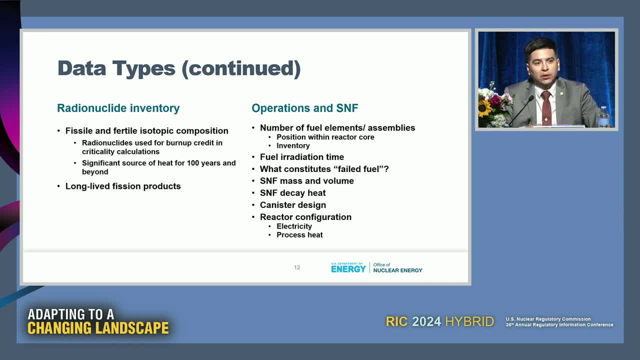 in the future we will be meeting areas where there's a lot of variation on how fuel works. So we have a few things here. One of the first things is to look at the operations and the rate at which a spinocle fuel is being discharged from our reactor. 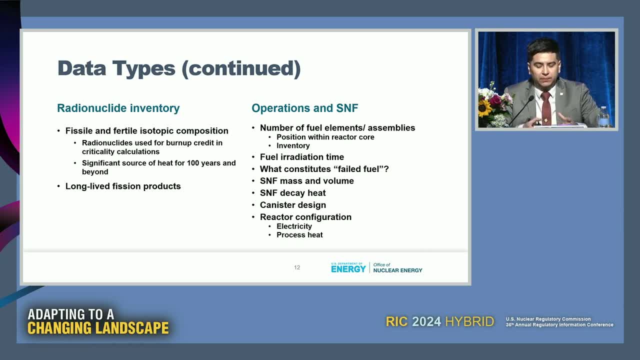 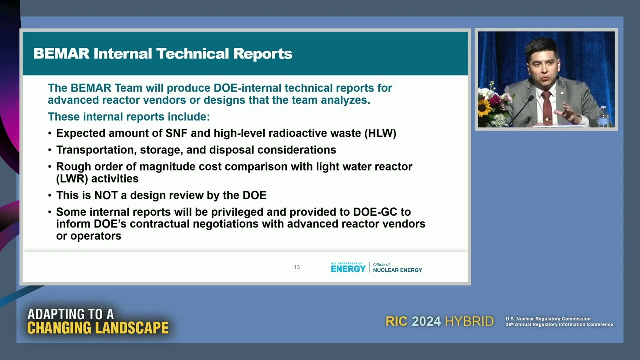 So that includes looking at the core. how many fuel elements are in the core, how often spinocle fuel needs to be removed, what is a fuel element, among other things? So once we collect all of this data, we start to look at the size of the fuel. we start. 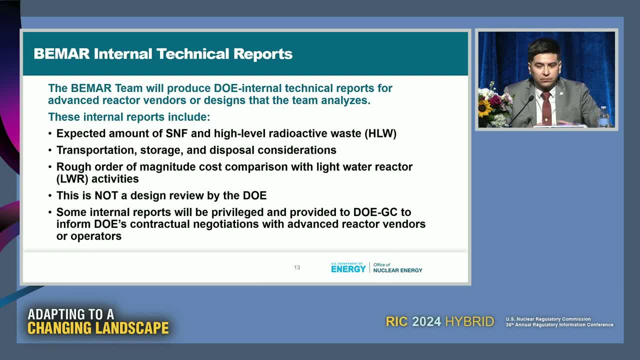 we start working on internal reports, and these internal reports include the expected amount of aspenucle fuel and high-level waste that a reactor design or a company is planning on generating for the lifetime of the reactor, some considerations for transportation, for storage and disposal, a rough order of magnitude cost comparison with light-water reactors. 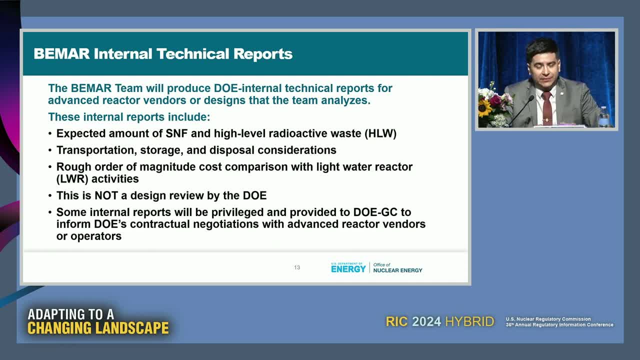 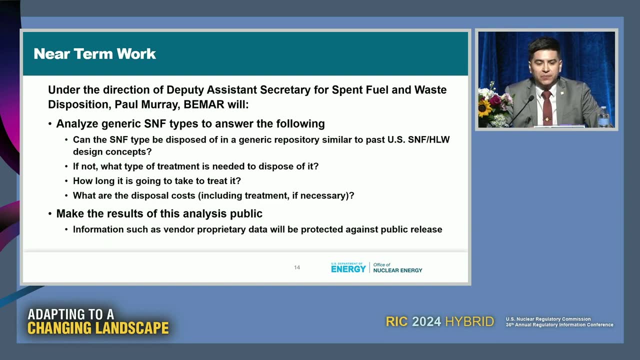 I need to specify that this is not a review by DOE. We're only looking to collect data so that we can inform ourselves and also the DOE Office of General Counsel. So for the last couple of minutes that I have, I want to talk about the near-term work that 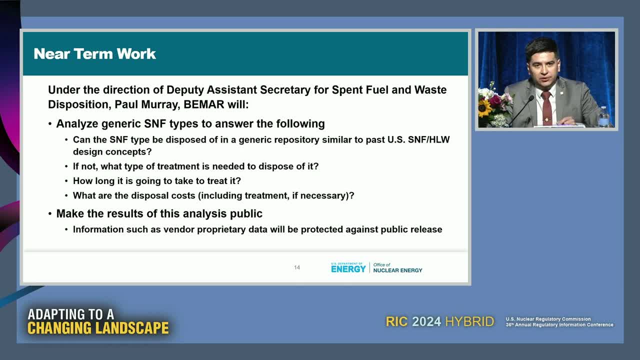 BMR is doing So under the leadership of Deputy Assistant Secretary for Aspen Fuel and Waste Disposition, Paul Murray. BMR has been tasked to analyze the generic types of aspenucle fuel from advanced reactors. So think about tris of aspenucle fuel, metallic fuel and molten-sol reactor aspenucle fuel. 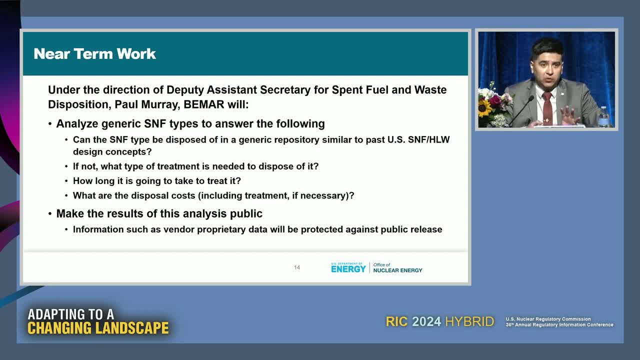 And the goal of this is to answer the four following questions. The first one is: can the generic aspenucle fuel be disposed of in a generic repository that is similar to previous DOE concepts? If not, then what is it going to take to dispose of the material of the aspenucle fuel? 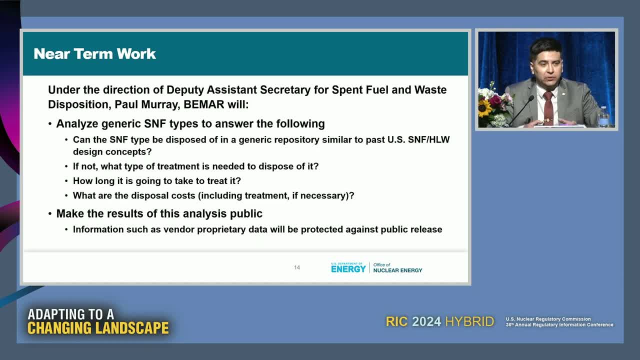 So that would involve: what kind of treatment do we need to do on the aspenucle fuel to make it disposable? How long is it going to take and how much is it going to cost to dispose of the aspenucle fuel, including any treatment cost if that's applicable to a particular generic type of? 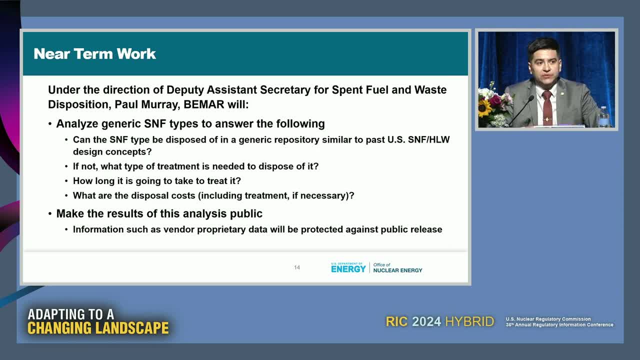 aspenucle fuel. We are hoping to make the results of this work available to the public. That's going to be forthcoming. We started doing this work at the beginning of this year and hopefully we can have some of that available to the public, maybe next year. 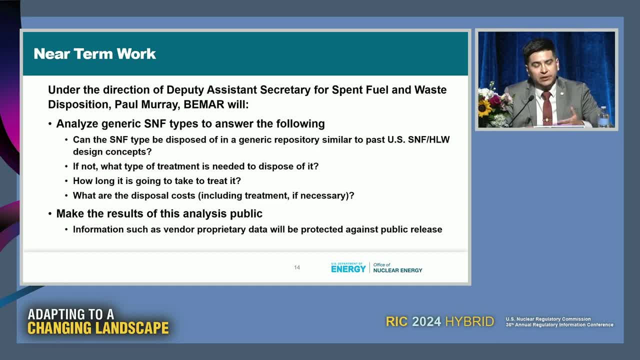 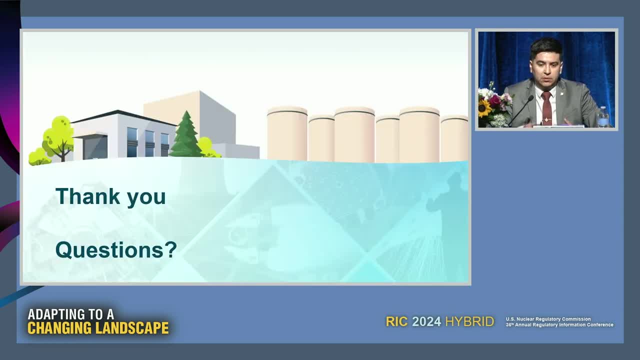 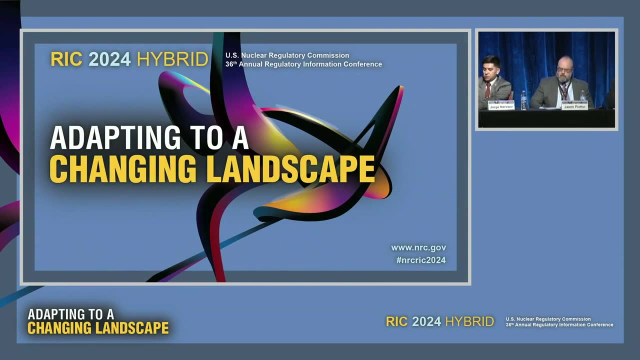 So we are planning on making this publicly available. We are required to protect vendor proprietary data against public release, And I believe that's all for me. Thank you very much. Thank you, Jorge, Appreciate it, And it's great to hear what our fellow federal agencies are doing. 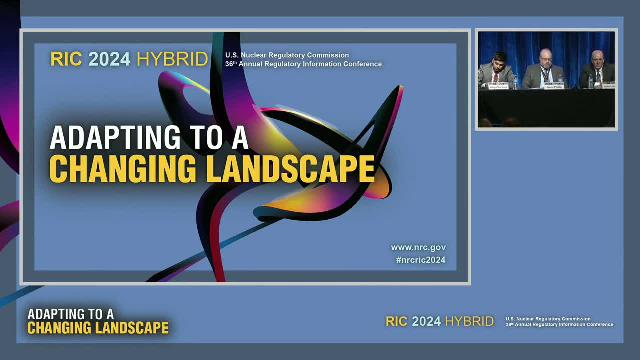 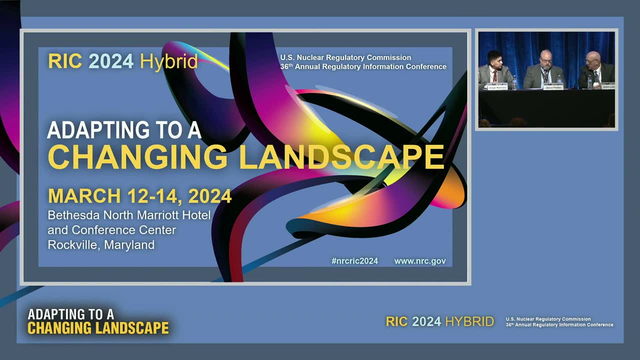 It really helps us, being independent from DOE, to really get an understanding of where we see some of the drivers out there and what we can see coming forward, And having that coordination early really helps. as Jason said, it helps with understanding where we can budget and engage in pre-application activities. 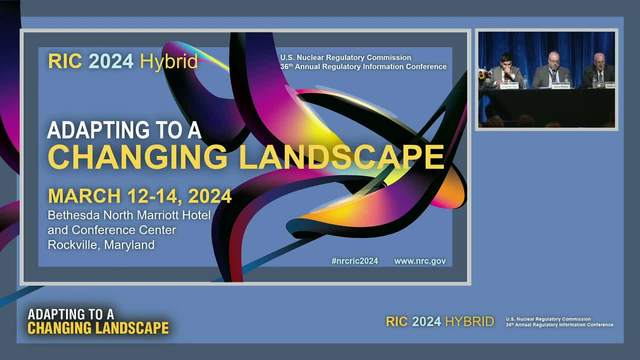 Next, I'd like to introduce Victoria Huckabay. Victoria currently serves as a senior project manager in the NRC's Office of Nuclear Reactor Regulation in the Division of New and Renewed Licenses. She joined the NRC 10 years ago as a reactor operations engineer. 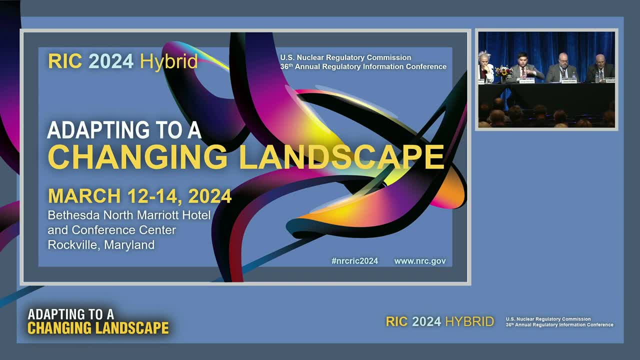 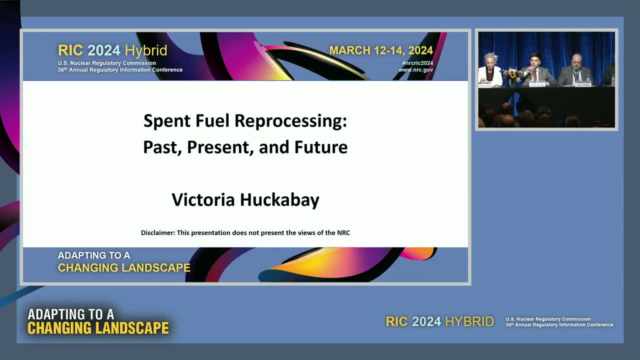 Prior to working at the NRC, Victoria worked in the private sector as an engineer and a quality assurance manager. She graduated from Georgia Institute of Technology with a master's degree in aerospace engineering. So thank you, Victoria. Thank you So good afternoon. 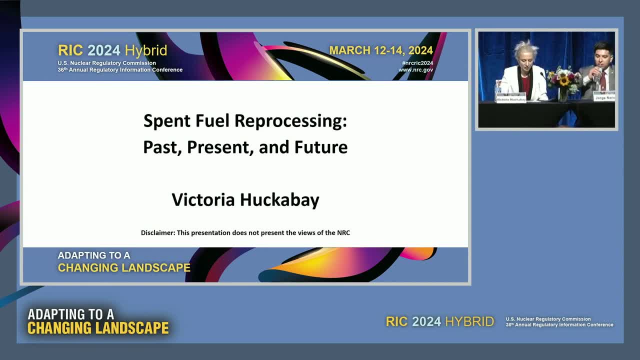 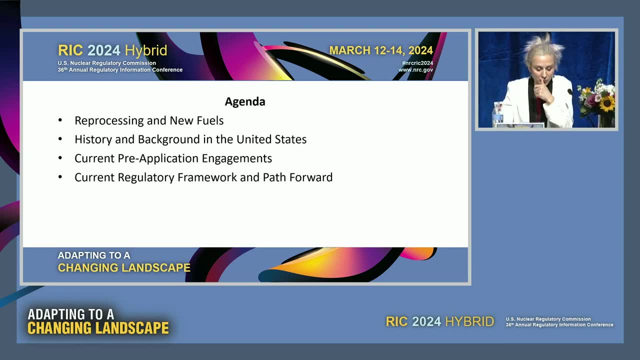 My name is Victoria Huckabay and today I'm going to discuss the NRC's perspective of the past, present and future of spent fuel reprocessing. I will briefly talk about the role of reprocessing in the manufacturing of new fuels provide. 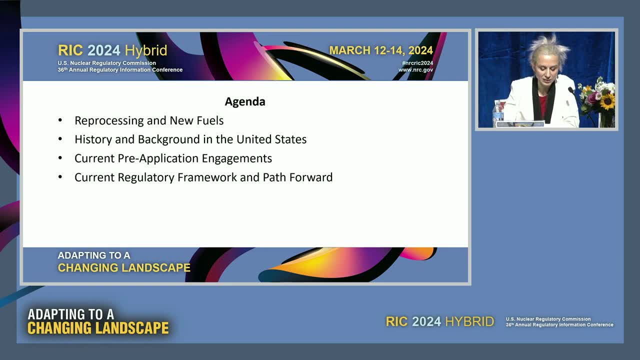 an overview of the history of reprocessing facilities in the United States. We will discuss the ongoing pre-application engagements with the NRC by potential future applicants for reprocessing facility licenses. We will close with an overview of the current regulatory framework for reprocessing facilities. 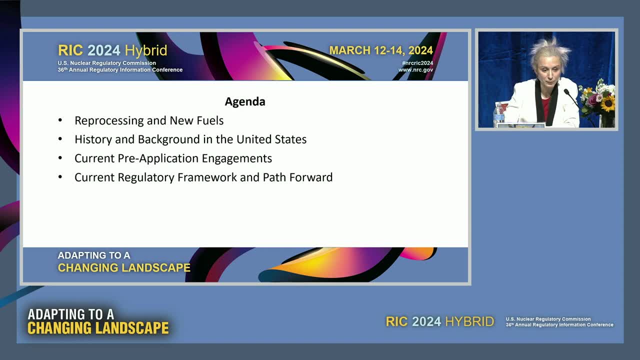 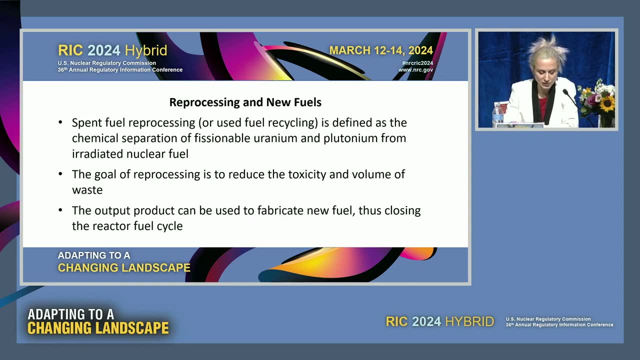 and the path forward for future development and enhancement. Spent fuel reprocessing, which is sometimes referred to as used fuel. recycling is defined as the chemical separation of fissionable uranium and plutonium from irradiated nuclear fuel. Several processes exist for reprocessing of spent fuel with a chemical-based plutonium-uranium reduction. 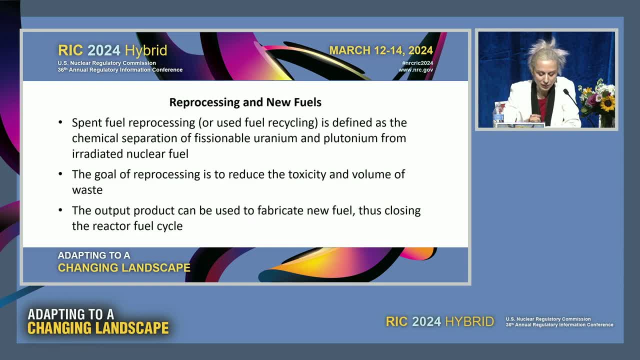 extraction or PUREX process dominating. This process works by chopping up fuel elements, dissolving them in concentrated nitric acid and chemically separating uranium and plutonium using tributyl phosphate. There is a modified version of PUREX called UREX, which does not. 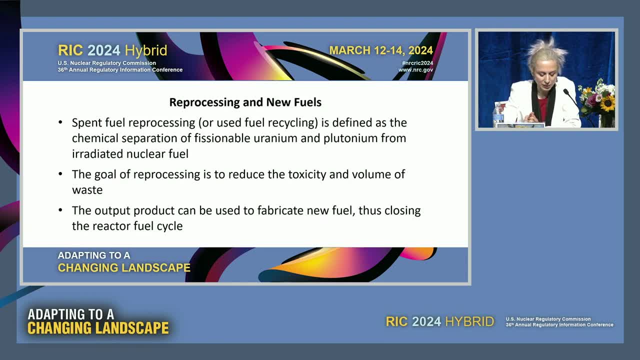 involve the isolation of the plutonium stream. Spent fuel reprocessing reduces the volume of material to be disposed of as high-level waste and reduces the consumption of raw materials. In addition, the level of radioactivity in the waste from reprocessing is much smaller. 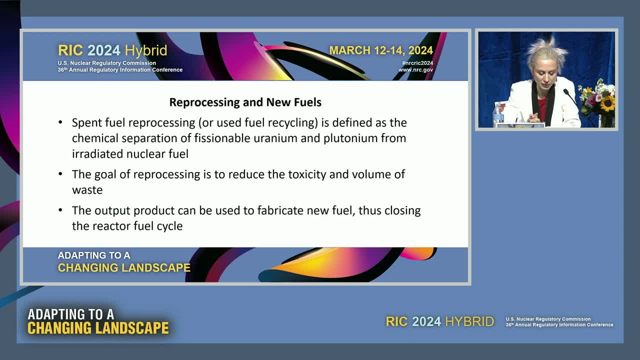 and after about 100 years, falls much more rapidly than in the spent fuel itself. The recovered unused plutonium and unused uranium can be used to manufacture new fuel, gaining some 25 to 30 percent more energy from the original uranium in the process. 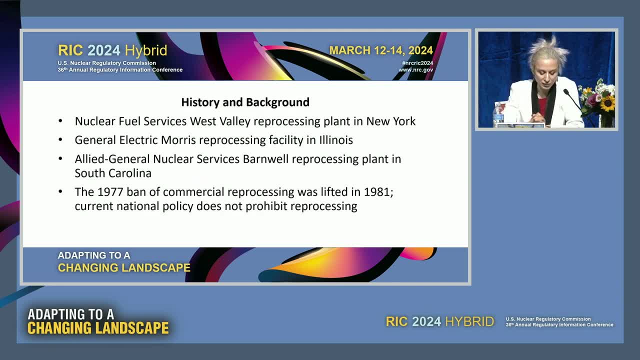 In 1964, the US Department of Defense and the US Department of Defense and the US Department of Defense, the Atomic Energy Commission, granted an operating permit for commercial reprocessing to the Nuclear Fuel Service for the West Valley plant. The West Valley plant. 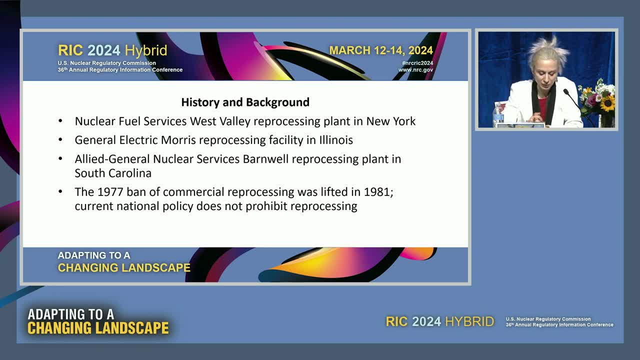 operated from 1966 to 1972.. A total of 640 metric tons of spent reactor fuel was processed, which resulted in a large amount of radioactive waste which was left on site for many years. However, most of it went through a vitrification process in the early 2000s. In 1967, the Atomic 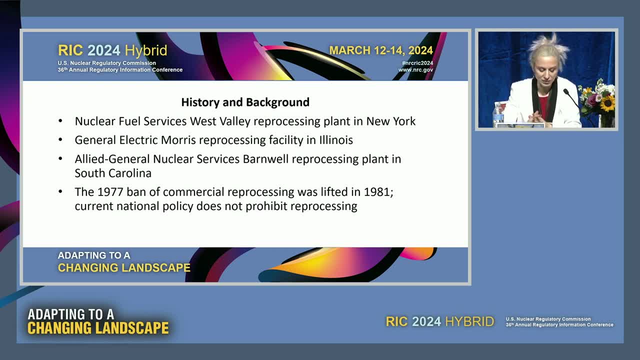 Energy Commission authorized General Electric to construct a spent fuel reprocessing facility in Morris, Illinois. The facility was built in 1971, conducted functional testing but did not operate as a reprocessing facility on a large commercial scale. In 1972, it received a license. 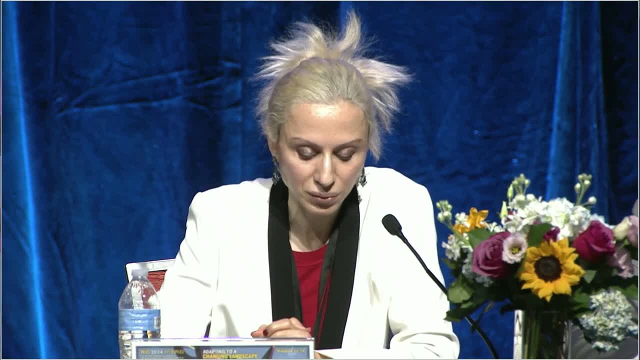 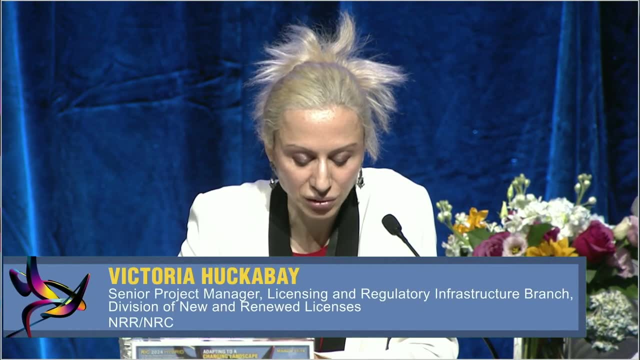 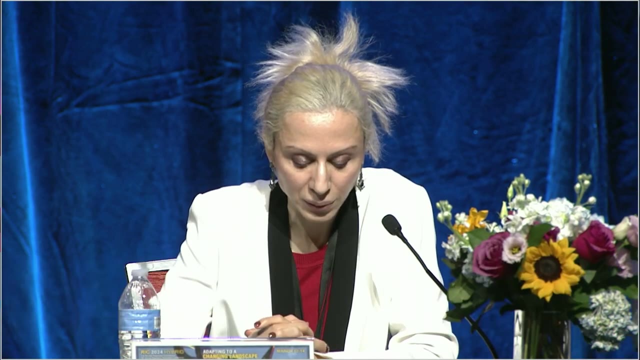 to store spent fuel and for many years Morris served as a wet-independent spent fuel storage installation. In 1970, Allied General Nuclear Services began construction on a larger commercial reprocessing plant in Barnwell, South Carolina. However, in 1974, the Atomic Energy Commission stated that any decision to permit nuclear fuel 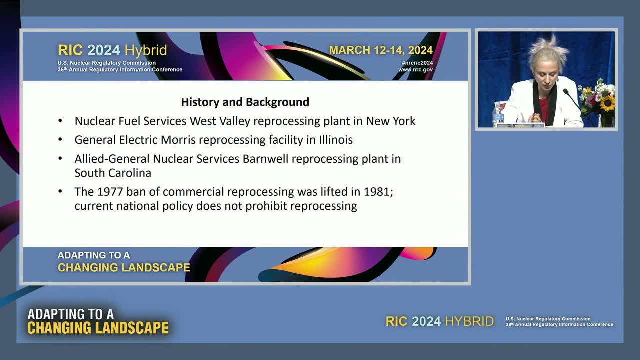 reprocessing on a large scale would require the development of an environmental impact statement under the National Environmental Policy Act. In 1976, the facility was halted mid-construction due to the risks of proliferation, Although the ban on commercial reprocessing was lifted by President. 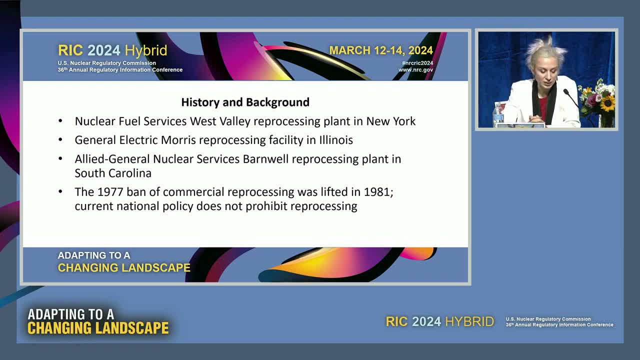 Reagan in 1981, it did not regain support in the United States due to economics and historical changes in national policy. The Atomic Energy Commission stated that any decision to permit commercial reprocessing on a large scale would require the development of an environmental impact statement. 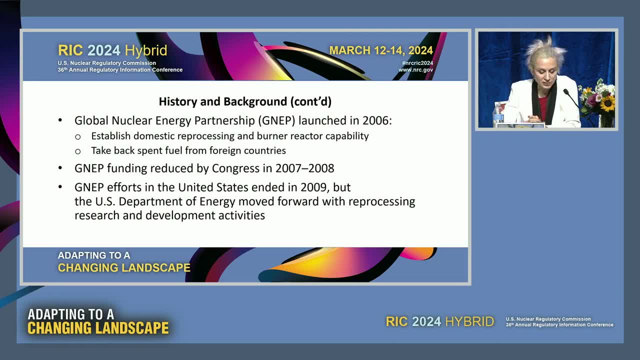 under the National Environmental Policy Act. There were no advances in the area of reprocessing in the United States until 2006, when the Department of Energy announced the Advanced Fuel Cycle Initiative to create a scale demonstration of the URX-Plus separation process and develop an advanced fuel cycle facility. The intent 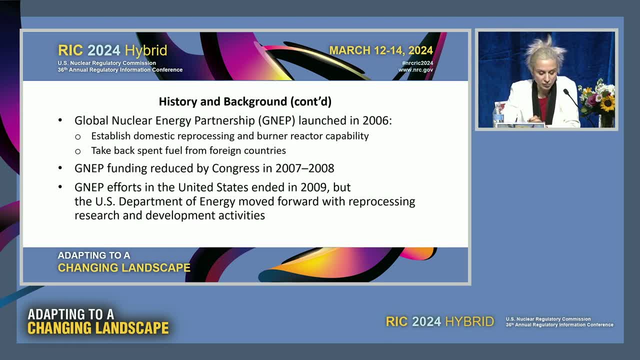 for the Advanced Fuel Cycle Initiative was to develop proliferation-resistant nuclear technologies with the help of the Global Nuclear System. The US Department of Energy's Nuclear Energy Partnership, or GNEP, was also involved. The goals of GNEP included reducing the US 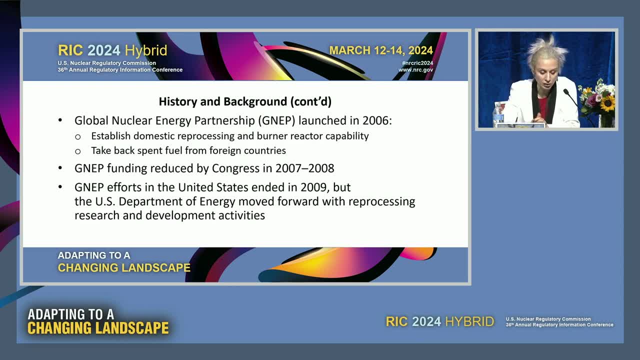 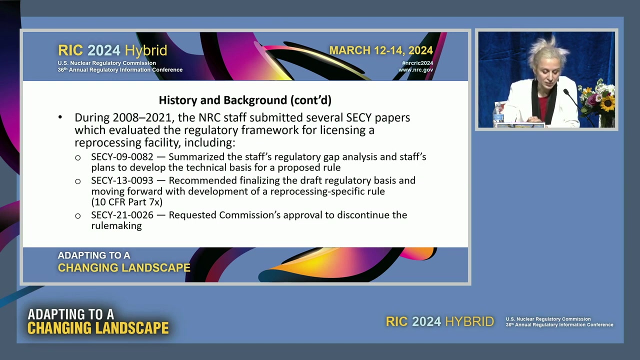 independence on foreign sources of fossil fuel and encouraging economic growth, as well as recycling nuclear fuel using new proliferation-resistant technologies to recover more energy and reduce waste. However, in the following years, Congress significantly reduced GNEP's funding, while DOE continued moving forward with reprocessing research and development, Starting in 2006,, the NRC staff 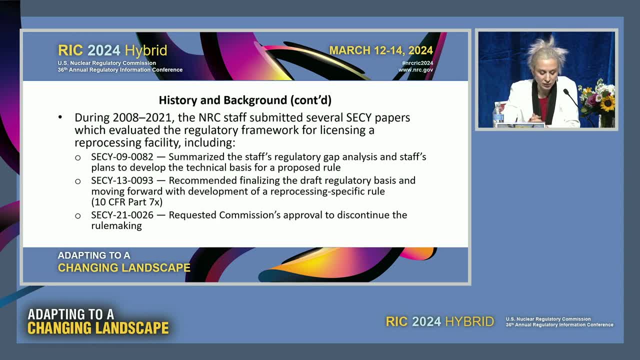 began to work on the project. and the NRC staff began to work on the project, and the NRC staff on interacting with the Commission regarding the topics related to the development of conceptual framework for licensing GNAP facilities, as well as licensing of any commercial reprocessing. 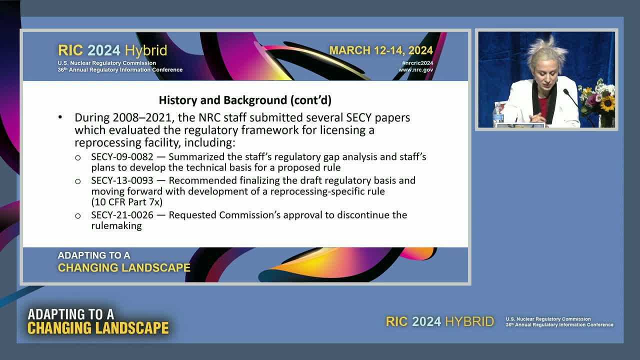 facilities in the United States. The NRC staff submitted several SECI papers to the Commission, some of which are highlighted in the slide. SECI 090082,. in that paper, the staff provided an update summary of the regulatory gap analysis and informed the Commission of its plan to develop. 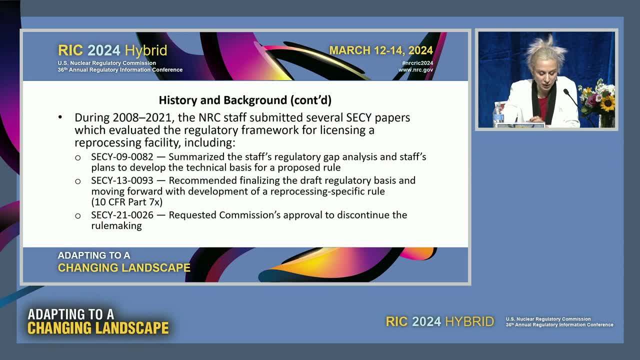 the technical basis for a proposed rule that would resolve the high-priority gap In SECI 110163, not shown on the slide. the staff provided a draft regulatory basis for licensing and regulating reprocessing facilities that addressed the previously identified regulatory gaps and discussed a path forward for updating the regulatory framework Then in SECI 130093,. 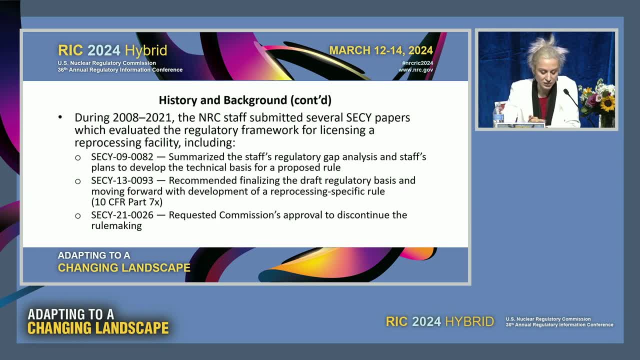 the staff recommended moving forward with developing a reprocessing-specific rule, Part 7X, which would provide an individual-specific rule, which would provide an individual-specific rule, which would provide an integrated and cohesive regulatory framework that would address the specific safety and safeguards needs of a reprocessing facility. And finally, in SECI 210026,, the staff requested 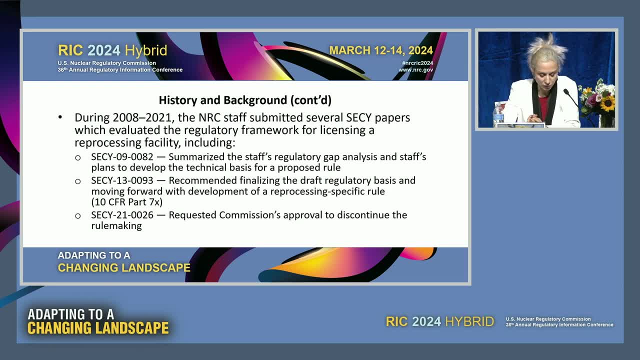 Commission approval to discontinue spent fuel reprocessing rulemaking activity. The staff stated that in the event that the NRC received an application for a commercial reprocessing facility, the NRC would likely use the existing regulatory framework in Part 50, noting, however, that exemptions from certain Part 50 requirements would not be required, The NRC would likely use the existing regulatory framework in Part 50, noting, however, that exemptions from certain Part 50 requirements would not be required, The NRC would likely use the 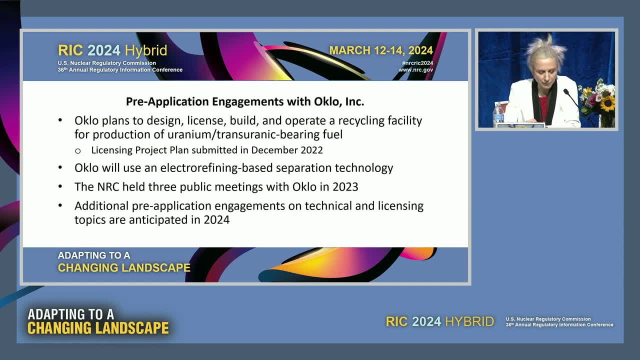 existing regulatory framework, in Part 50 requirements would not be required. The NRC staff is currently in pre-application engagements with two vendors regarding potential future applications for a reprocessing facility. The first vendor, Oklo, has expressed interest in designing building. 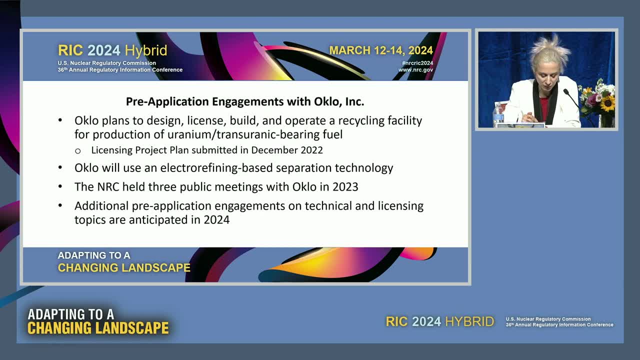 and operating a fuel recycling facility that would produce uranium transuranic-bearing fuel, referred to as U-True fuel. The facility would produce fuel for Oklo's metal-fueled fast reactors, closing the advanced reactor fuel cycle. The proposed facility would be used to produce fuel for 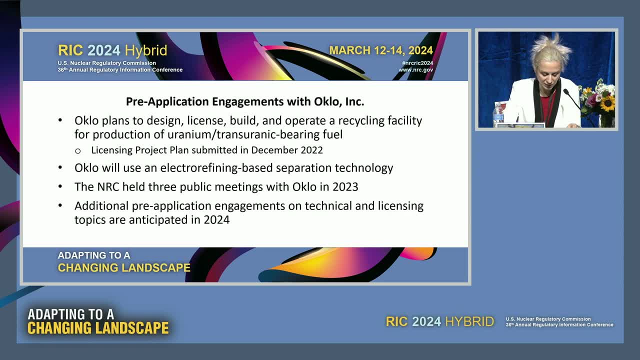 Oklo's metal-fueled fast reactors, closing the advanced reactor fuel cycle. The proposed facility would be technologically different from the previously licensed facilities in the United States, such as West Valley, Barnwell and Morris, which were AQS-based facilities. 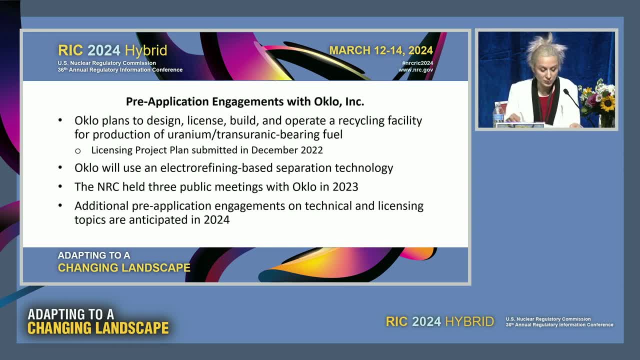 and would be based on electrochemical processing technology that has been extensively studied at Idaho National Laboratory and Argonne National Laboratory. In December 2022, Oklo submitted a licensing project plan outlining the pre-application engagements with the NRC. Since then, Oklo participated in three public meetings with the NRC staff, discussing topics: 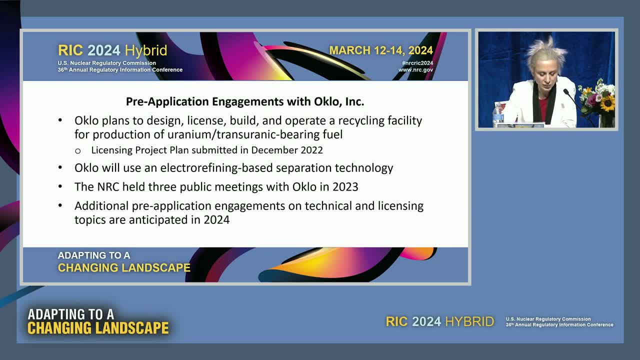 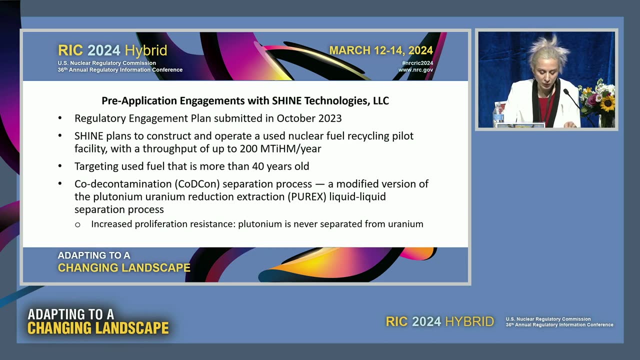 such as the licensing strategy and approach and the preliminary material categorizations for a fuel recycling facility. Additional public meetings on technical and licensing topics will be planned throughout calendar year 2024.. The second vendor, Shine Technologies, plans to construct and operate a used nuclear fuel recycling pilot facility to demonstrate the technology and economics necessary. 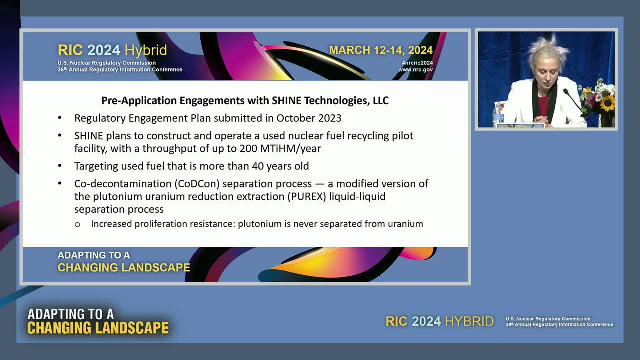 for the used nuclear fuel recycling to be viable. Shine plans to extract usable materials, including uranium and plutonium, for nuclear fuel recycling. The second vendor, Shine Technologies, plans to extract usable materials including uranium and plutonium for new mixed oxide and recycled. 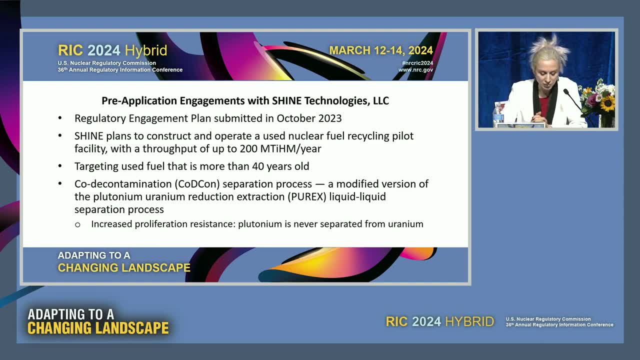 uranium fuel and valuable fission product isotopes such as neptunium-237.. Shine also intends to harvest the actinides for sale or future destruction through transmutation, further reducing the toxicity and longevity of the remaining waste. Shine estimates that, after reprocessing, 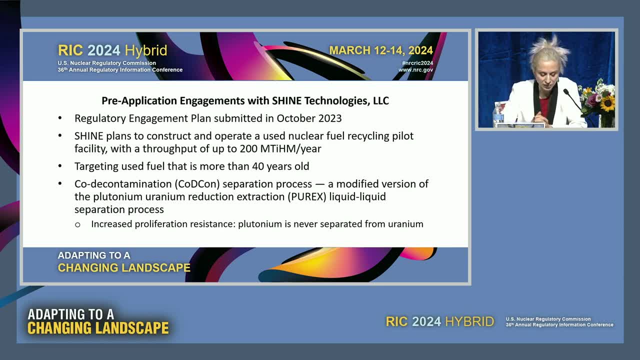 approximately 95% of waste will be suitable for near-surface disposal. Shine's proposed facility throughput is estimated to be up to 200 metric ton of initial heavy metal per year. The pilot facility will process spent fuel that has been decayed at least 40 years after. 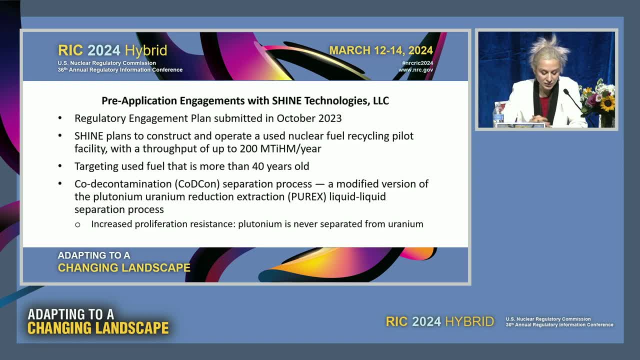 discharge from the reactor. Shine's reprocessing technology will use the co-decontamination process called CODECON, which is a modified version of the PUREX liquid-liquid separation process that is used to separate the major actinides from the bulk dissolved spent fuel, A key differentiation. 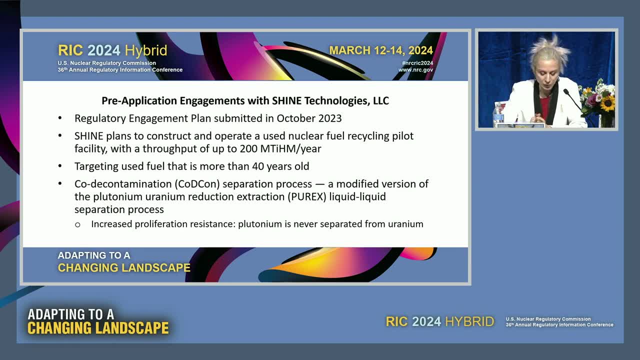 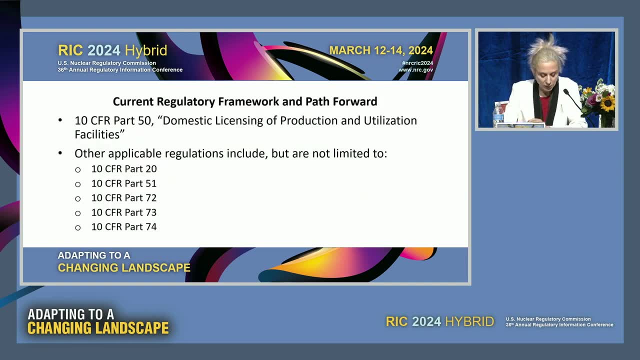 from the PUREX process is that plutonium is never separated from uranium, which provides increased proliferation value. The PUREX process is used to separate the major actinides from the bulk dissolved resistance. Currently, 10 CFR Part 50 provides the licensing framework for production and utilization. facilities. A reprocessing facility would likely fall under the definition of a production facility in 10 CFR 50.2.. In addition, licensees under Part 50 must also comply with the requirements found in other parts of Title 10 of the Code of Federal Regulation, some of which are shown. 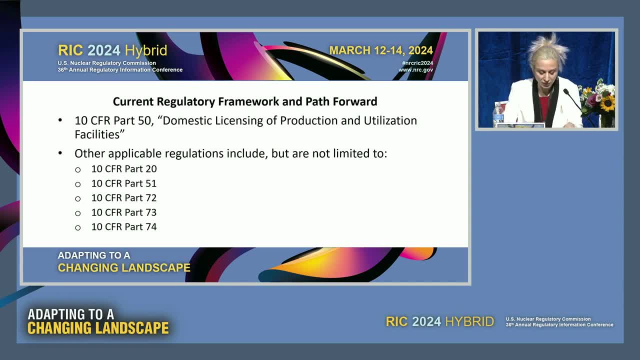 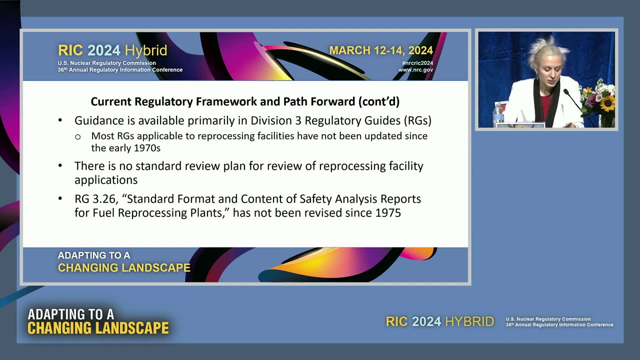 on the slide, such as, for example, 10 CFR, Part 20, standards for protection against radiation, 10 CFR, Part 51, environmental protection, regulations for domestic licensing and related regulatory functions, and so forth. There are approximately two dozen regulatory guides that provide guidance on various topics. 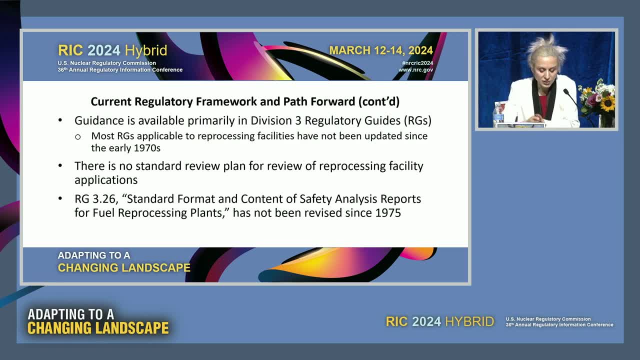 applicable to reprocessing facilities. With a few exceptions, the majority of these documents have not been updated since the early 70s and, as a result, the guidance contained in these documents is rather limited and may be inconsistent with the regulations as they have. 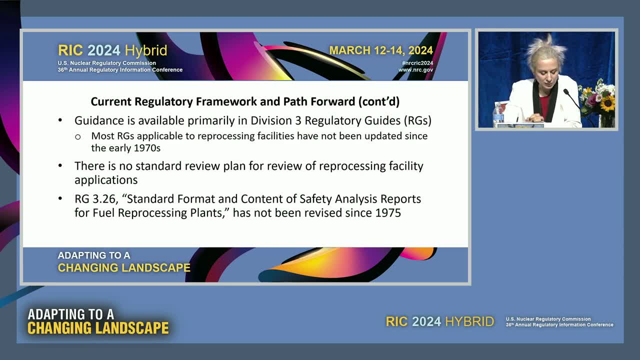 evolved in the past five years, 50 years. There is no standard review plan developed specifically for reviewing a fuel reprocessing facility application, which may present a challenge both for the NRC staff and potential applicants in terms of defining clear expectations for the format, content and acceptability. 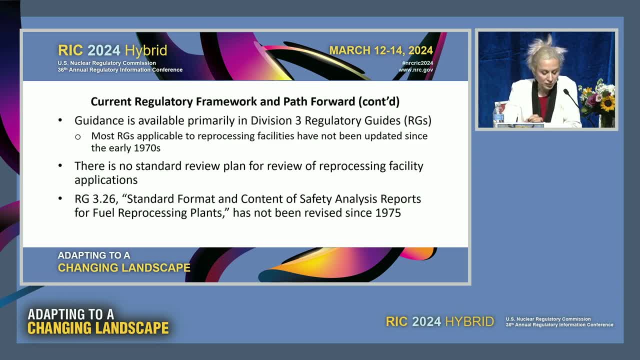 of an application for a reprocessing facility. However, regulatory guide 3.26, standard format and content of safety analysis reports for fuel reprocessing plans provides some guidance for various technical topics that the NRC staff would expect to see addressed in an application for a reprocessing facility. 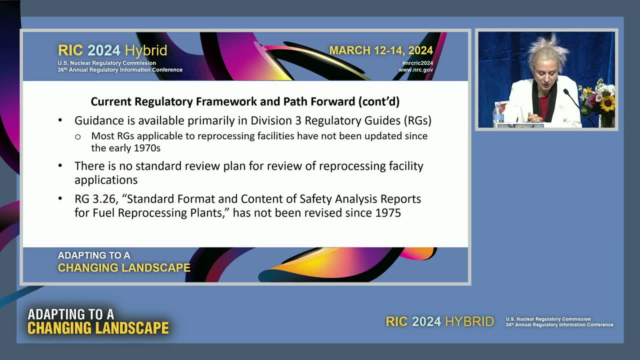 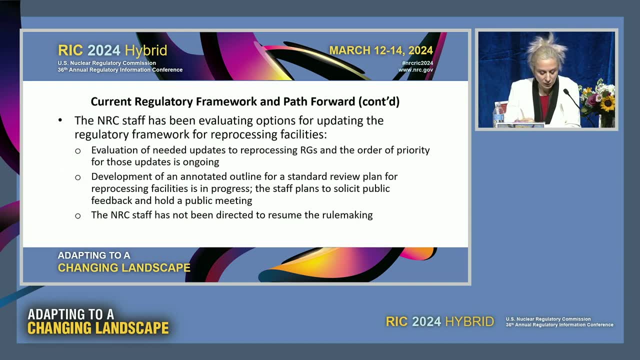 The NRC staff cautions, however, that this document has not been updated since 1975, and therefore the guidance contained therein is incomplete and may be out of date In 2023,. the NRC staff formed a working group aimed at evaluating the regulatory framework. 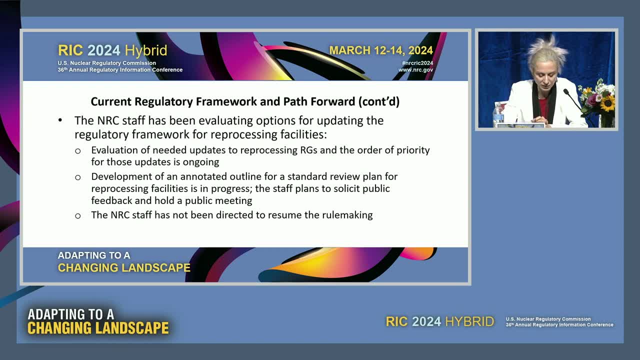 that would be used by future applicants for reprocessing facilities. The staff is evaluating whether any updates would be needed. The working group recommended the development of an annotated outline for a standard review plan that is specific to reprocessing facilities. This work is currently in progress and the staff is planning to hold a public meeting. 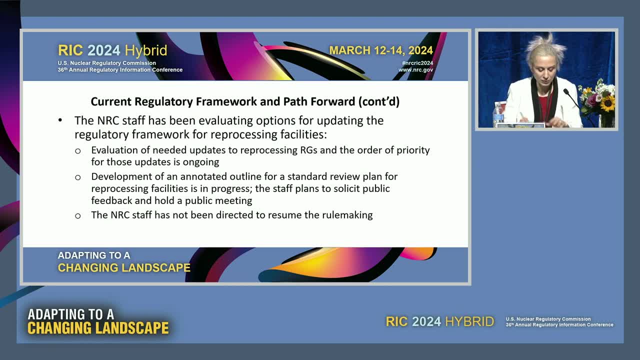 in a few months and soliciting public feedback on the document. The annotated outline will then be used in the development of the standard review plan. The staff's view remains that licensing a reprocessing facility can be adequately and safely accomplished under the existing framework and 10 CFR Part 50.. 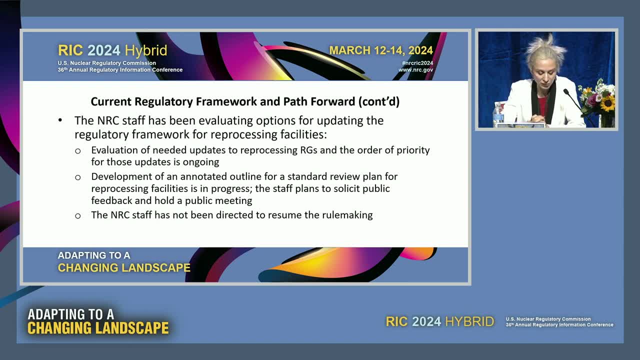 Moreover, the Commission has not given any new direction to the staff to resume the reprocessing rulemaking. However, the NRC staff continues to look for opportunities to develop and update existing guidance to improve the efficiency of the future licensing reviews of reprocessing facility. 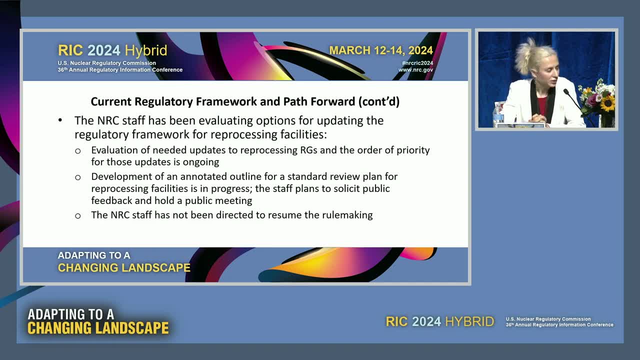 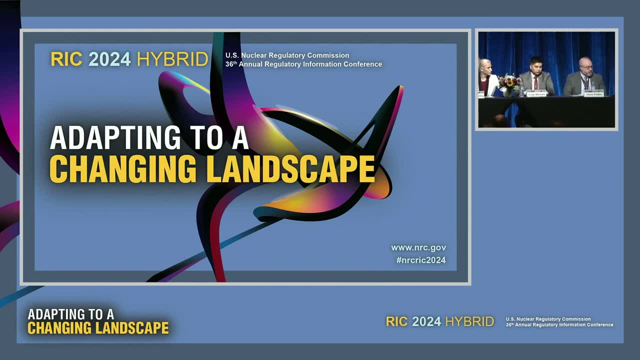 applications. And this concludes my presentation. Thank you, MR. Thank you, Victoria. I appreciate it. I think it's really great to hear the you know from the three presentations so far. I appreciate it. I think it's really great to hear that both the NRC and DOE are looking at the entire fuel. 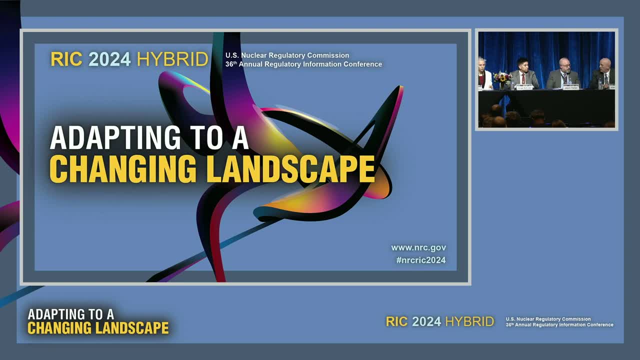 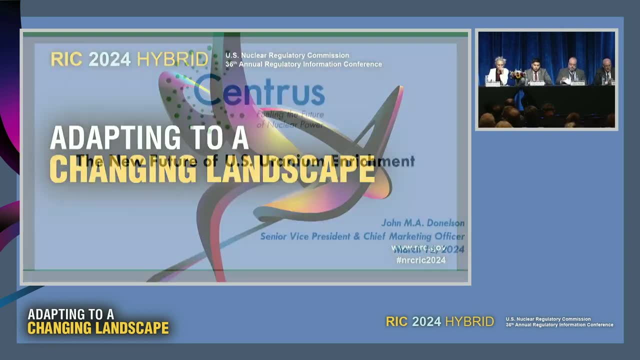 process, and not only the front end, but the back end and even potential for recycling that we're starting to see as well. Thank you. Next, I'd like to introduce John M A Donaldson, who is Senior Vice President and Chief Marketing. 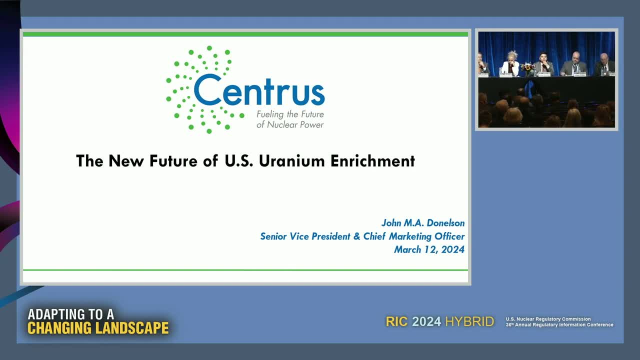 Officer for Centris Energy Corporation. Mr Donaldson joined Centris in 1995 in the Advanced Technology Department. He holds a Bachelor of Science degree in physics. MR. I'm John M A Donaldson, from Hamden-Sydney College a Master's degree in nuclear engineering. 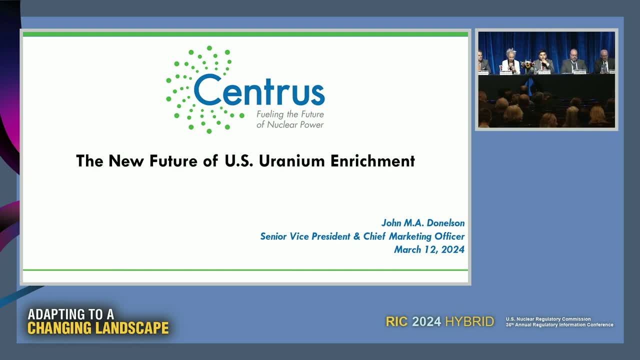 from the University of Virginia and a Master of Business Administration degree from Queens University. Thanks for being here with us, John MR, JOHN M, Good afternoon. I was lucky enough at lunch today to sit in on a NEI-hosted event where they had a speaker. 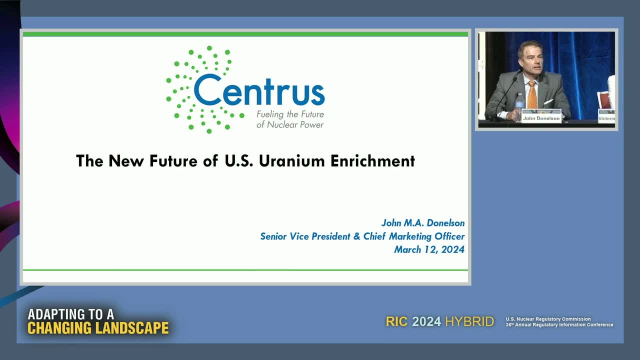 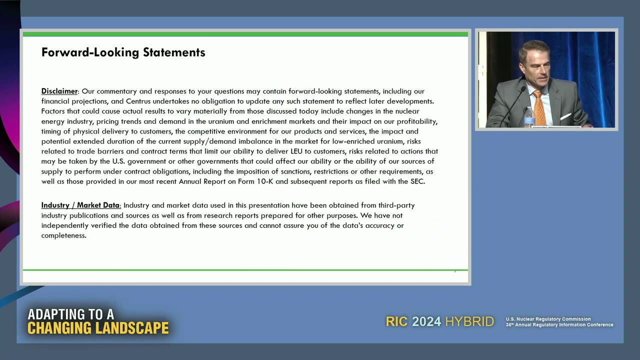 who has published a book called Smart Brevity, and the gist of his presentation- that is, an audience when they receive a presentation- only remembers one thing. So unfortunately I've already written this presentation before this lunch today, so bear with me. I work for Centris Energy. 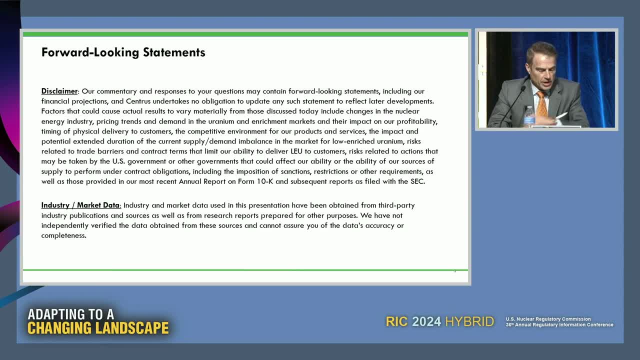 We're a publicly traded company. We're traded on the New York Stock Exchange. This is our safe harbor language. It's our company disclaimer. My personal disclaimer is that I'm a nuclear engineer, not a regulatory person. However, I have brought our company. regulatory expert with me, so if you have any tough questions in that area, I may have to phone a friend Who we are. Centris Energy is the only American-owned uranium enrichment company. Our headquarters is in Bethesda, Maryland. It's about two miles straight out the back door there. 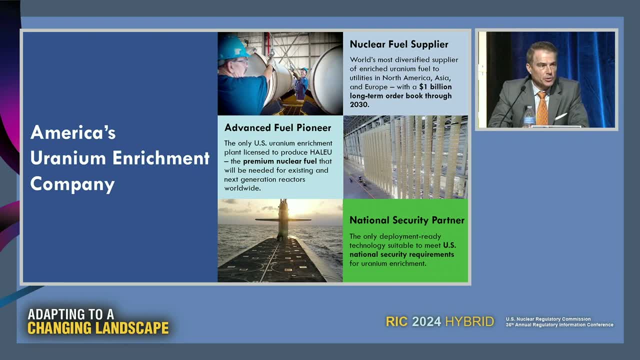 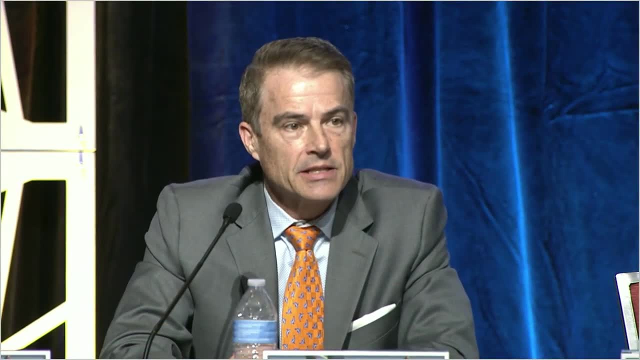 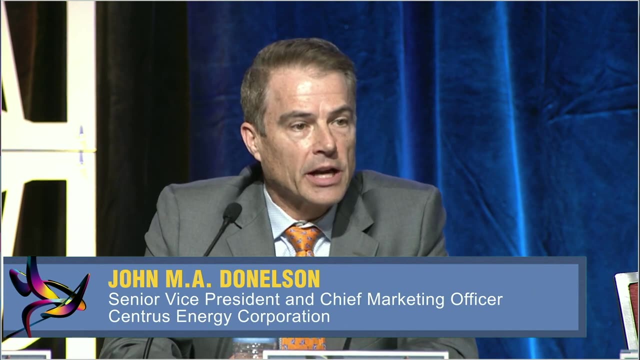 We have two business units. I run our commercial broker-trader LEU low enrichment company, LEU low enriched uranium supply business. We have customers in the United States, Asia and Europe. Our second business line is American Centrifuge Operations with locations in Oak Ridge, Tennessee. 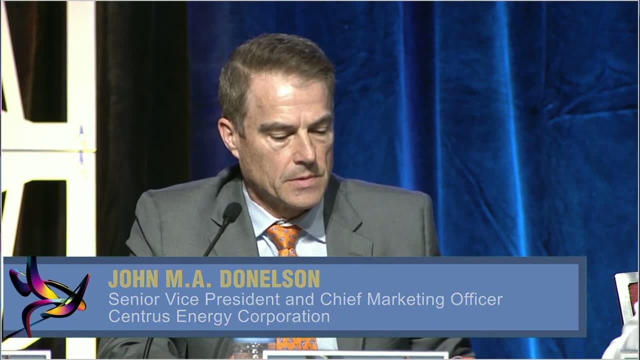 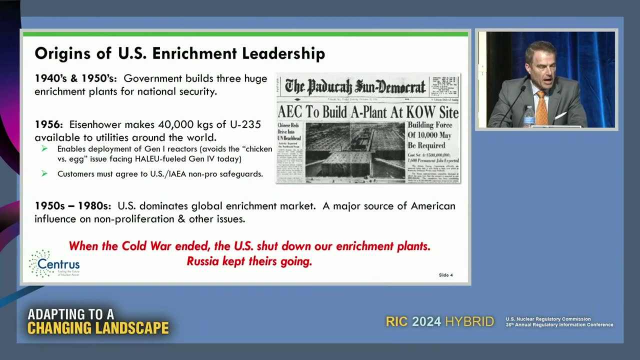 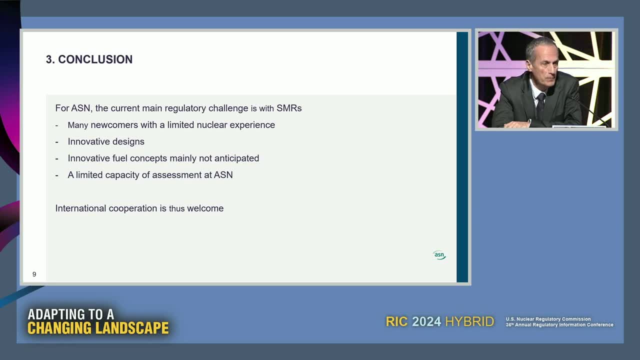 You know, for those of you that haven't seen the movie- Oppenheimer won seven Academy Awards, many newcomers with sometimes a very limited nuclear experience. also innovative designs, innovative fuel concepts- mainly not anticipated, and also for us, for ASN. 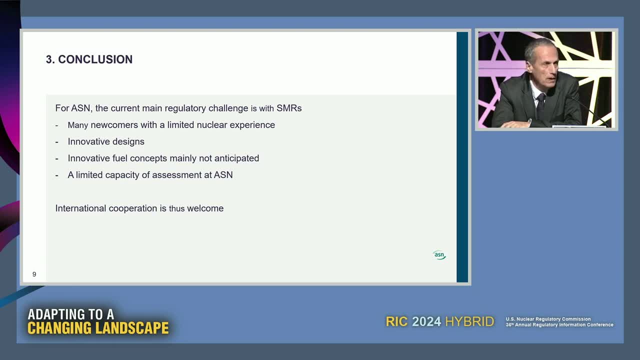 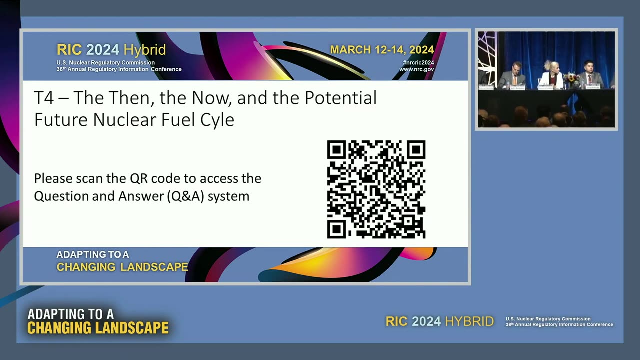 limited capacity of assessment, So that's why international cooperation is thus welcome. Thank you for your attention. Thank you very much, Commissioner Le Choum. Before we go to Q&A session, I do have a list of questions online here. I'd like to thank all the panelists for the presentation. 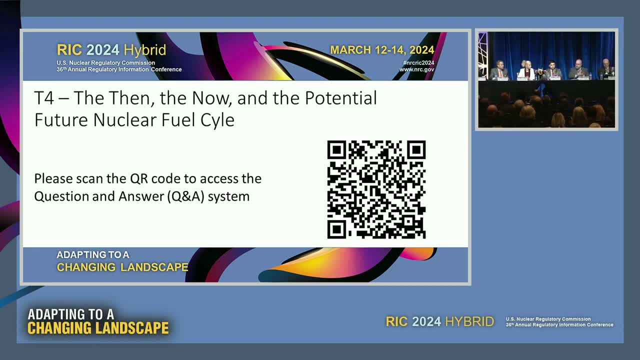 very informative and I'd like to give them a round of applause. So we have time to start going through the questions. We don't know if we'll make it through all of them and I'm going to try to start with a couple of easy ones. 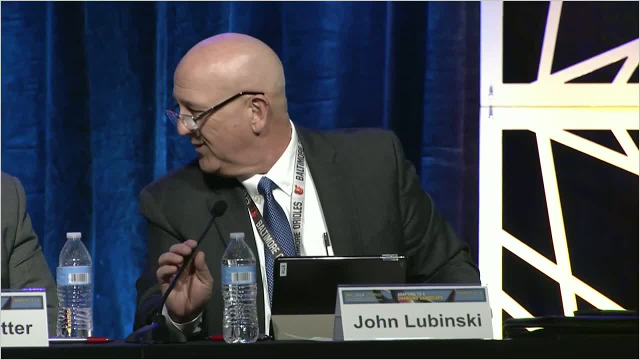 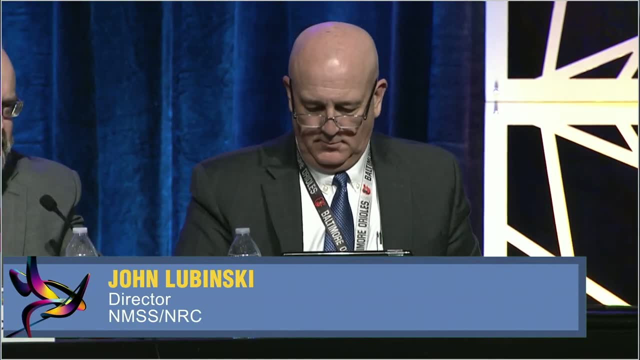 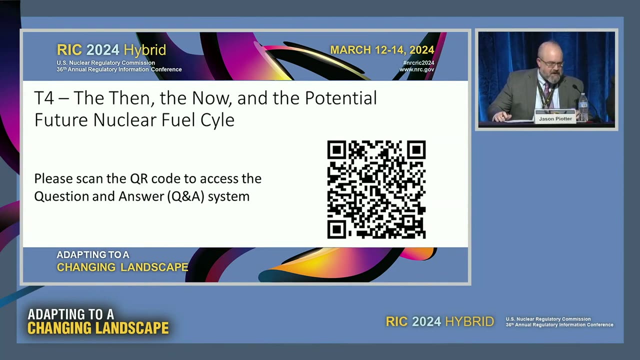 And they may get hard pretty quick, but we'll start. So, Jason, is the fuels atlas you mentioned available online? So I'm not sure which hedge words I'm going to use to start all my answers, but it depends or it's complicated. So part of the atlas is online. I mentioned the infographic. 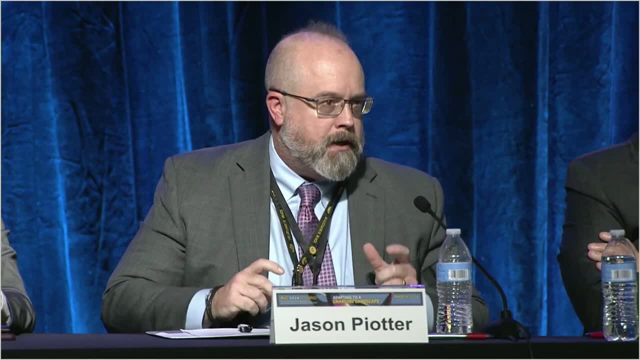 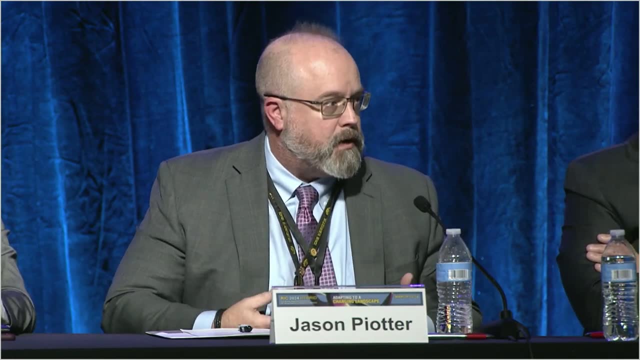 and I mentioned the webpage. Those are sort of our two initial efforts to get information to the public. Thank you. So the regulatory planner piece- that's the complicated part. We're still working on that. We're gathering information, We're still trying to determine what that's going to look like. 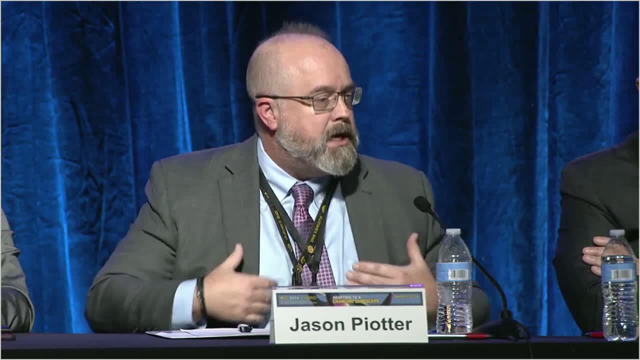 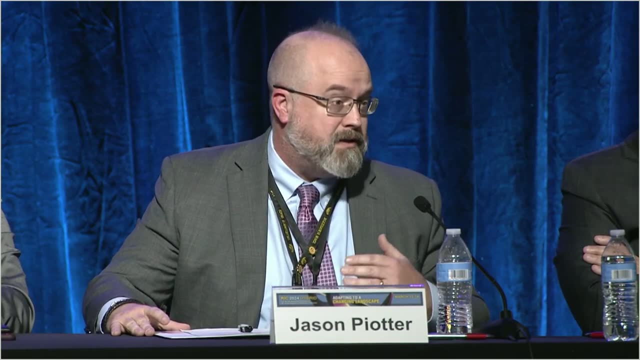 both internally and then how we're going to take that information and get it to the public. But, as I mentioned, the goal is to get as much information as we can to the public and to anybody else that's interested, to make sure that we're communicating exactly what it is we're doing. 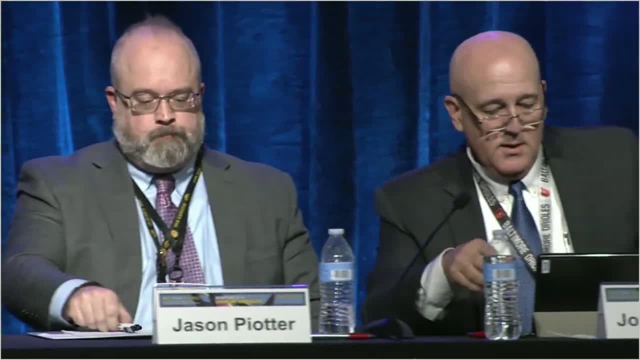 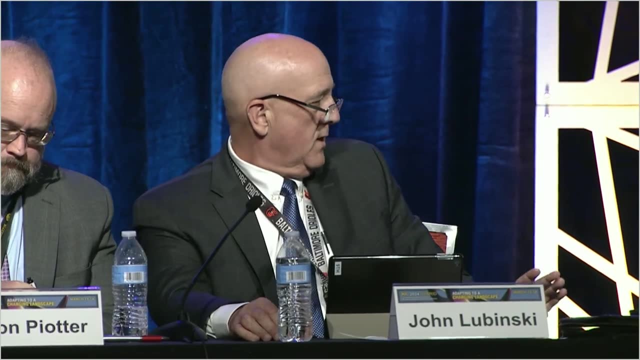 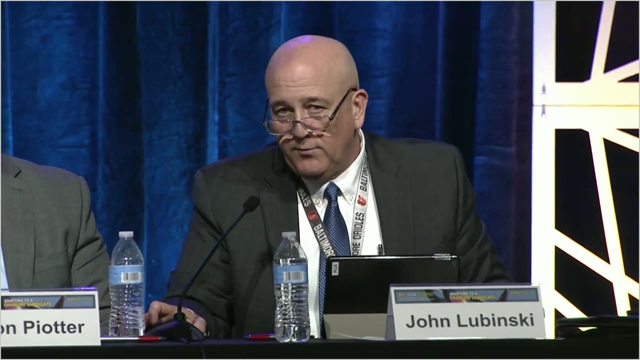 with respect to new fuels. Great Thanks, Jason. The next one: we had a question: How can I get copies of these presentation slides? And I'm looking to my folks over here and they're all online, correct. So if you go to the website how you logged into this session, all the slides should be available. 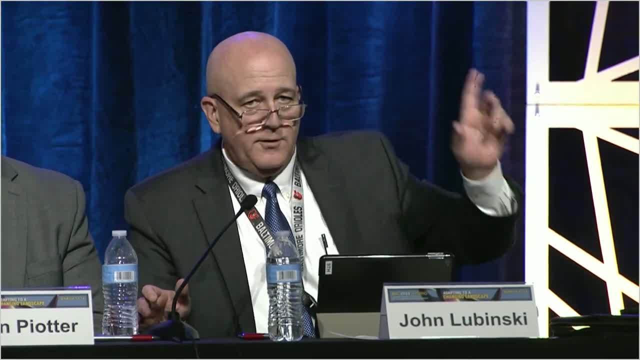 If you're having trouble, please stop and see one of the ladies at the front desk here and they'll get you to the right person. The next question: I see Victoria and Jorge are sharing a mic, so I'm going to have them share. 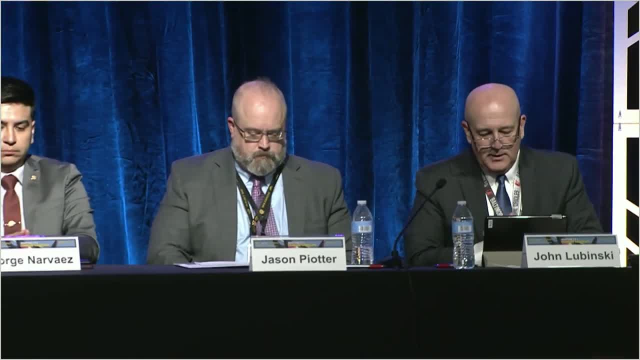 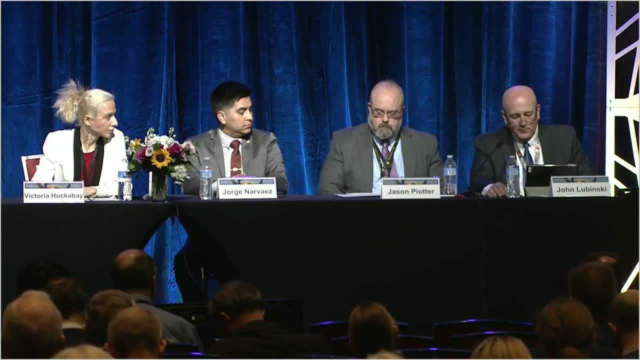 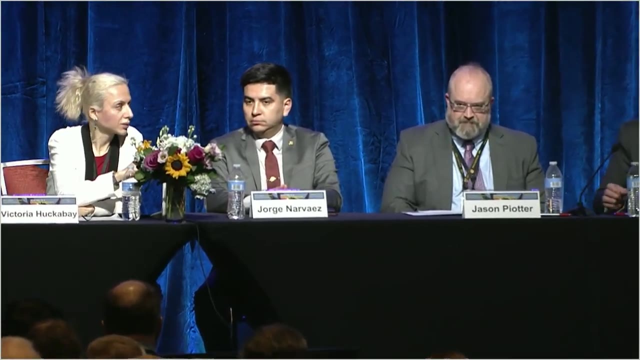 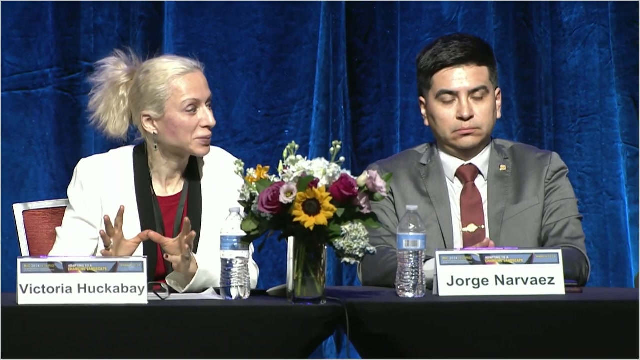 a question here. They both may want to chime in on this one. Are there any legal barriers preventing a private company who wants to do reprocessing, such as Oklo or Shine, from taking the spent fuel from a utility Right? So thanks, John. So I have to preface my answer with a statement that I'm actually not an expert. 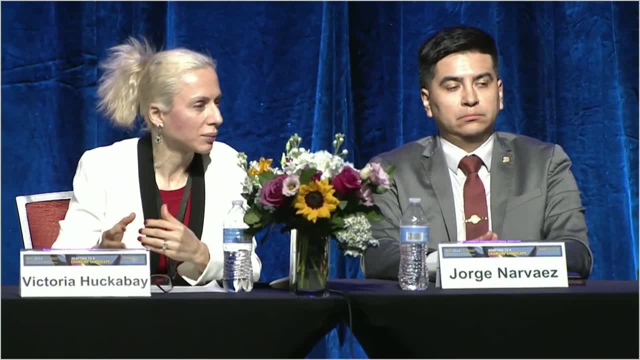 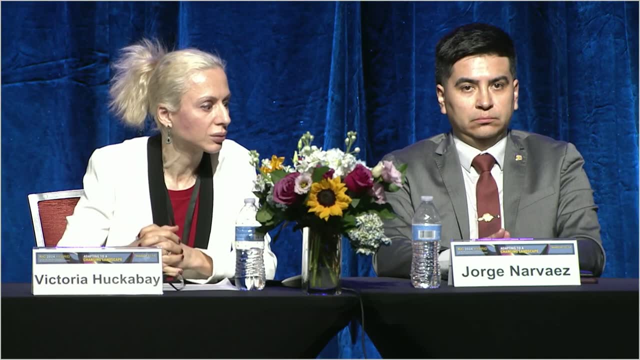 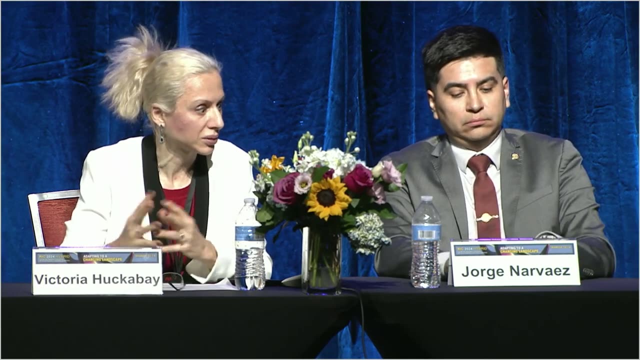 on the possession of spent fuel. So I'm sure there's certain questions that need to be explored there. So there's certainly going to have to be a conversation with- we would encourage a conversation with- the NRC about what plans such private entity- whether that's Oklo, Shine or any other potential applicant- would have. 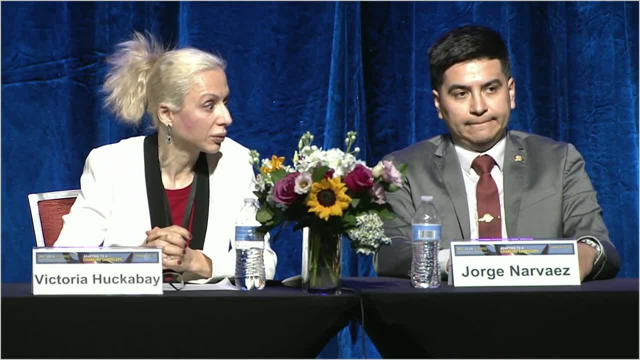 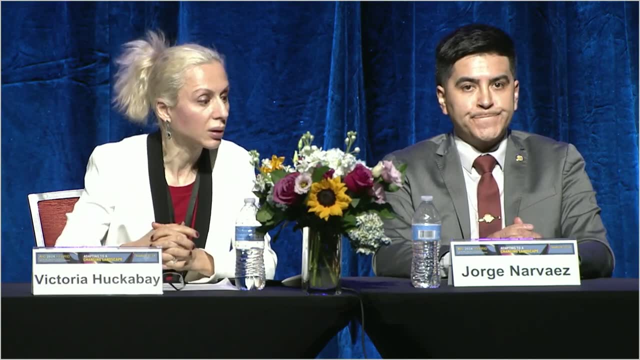 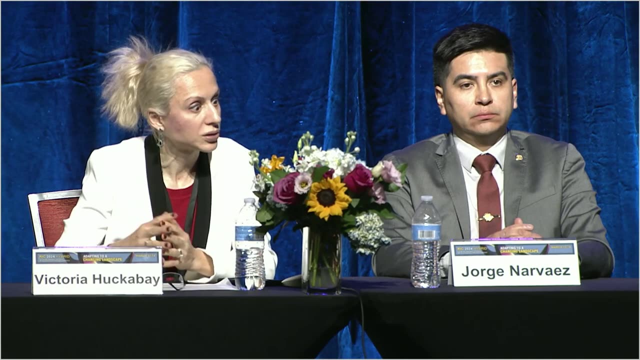 with regard to taking title of spent fuel and how that's going to work out and sort of what part in the process they plan to take possession, if at all. But there's perhaps another question I'd like to kind of bring up, just sort of thinking back to one of the 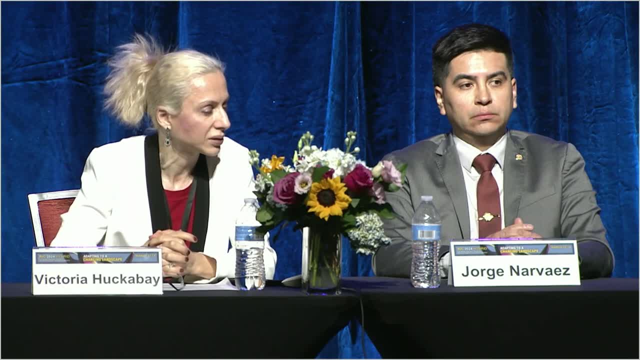 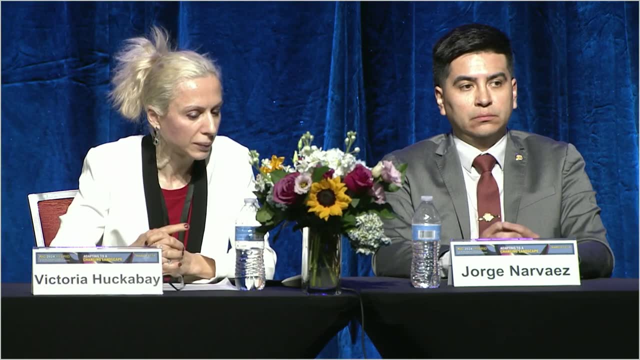 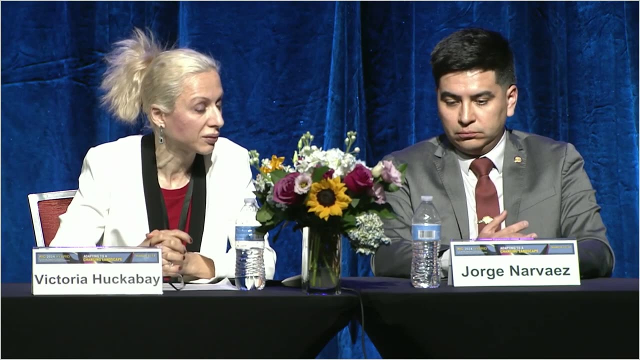 SECI papers that I've mentioned, and specifically the 2011 SECI paper. The draft regulatory basis discusses another important question, which was the question of disposition of high-level waste, And this was actually one of the regulatory gaps identified in the regulatory basis. 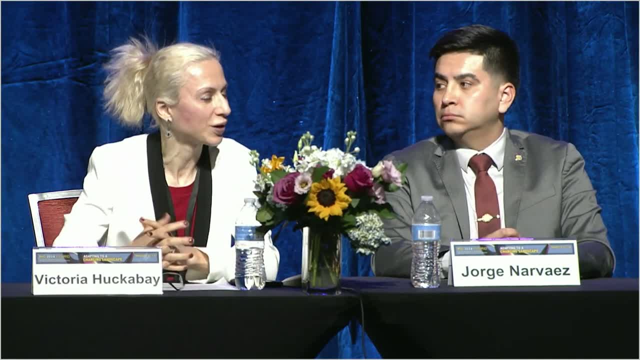 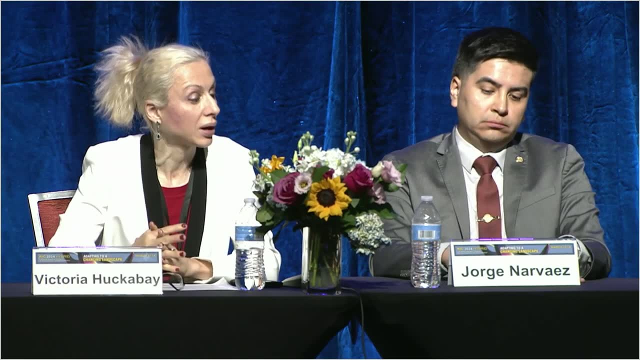 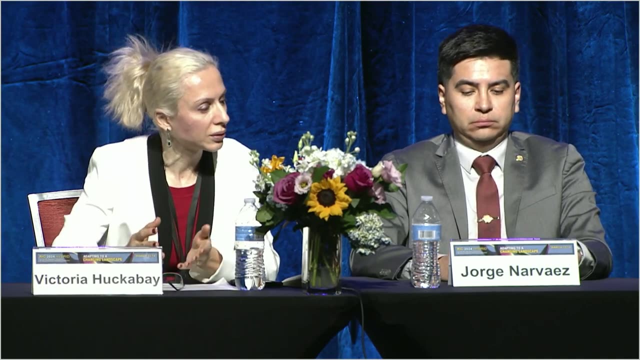 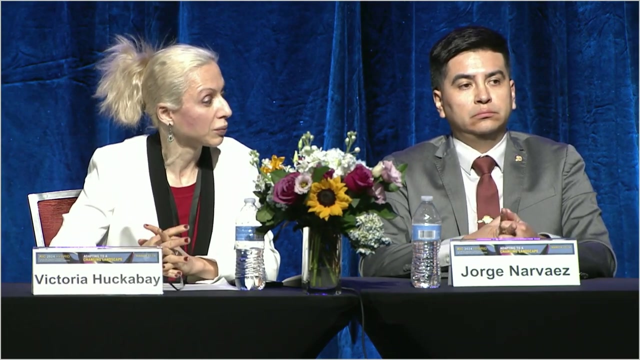 And I just looked it up on my phone. It was regulatory gap number two, So it discussed the potential issue of the generation of high-level waste from reprocessing, which we believe is likely, And so the question that would definitely need to be reviewed very closely and addressed is: what's going to happen? 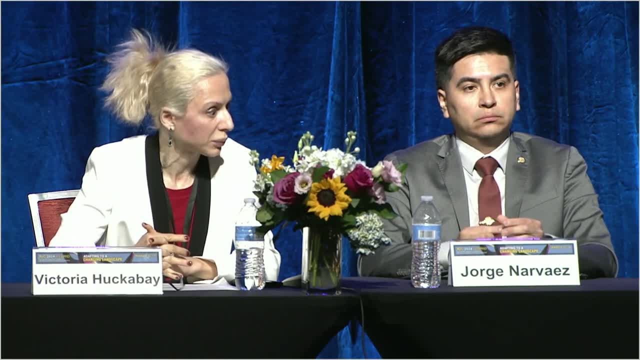 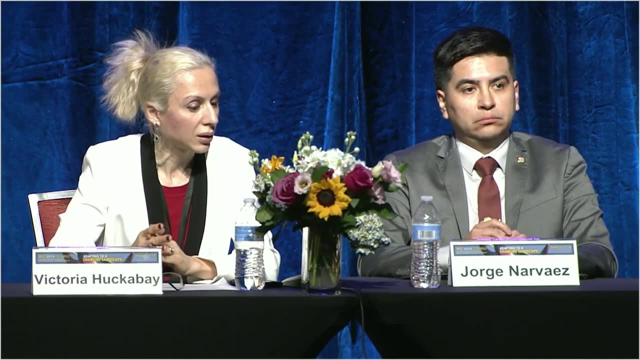 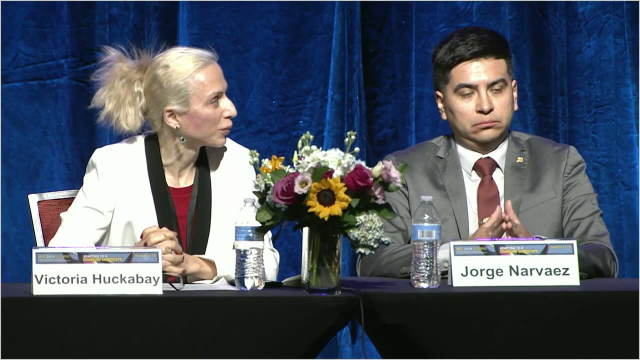 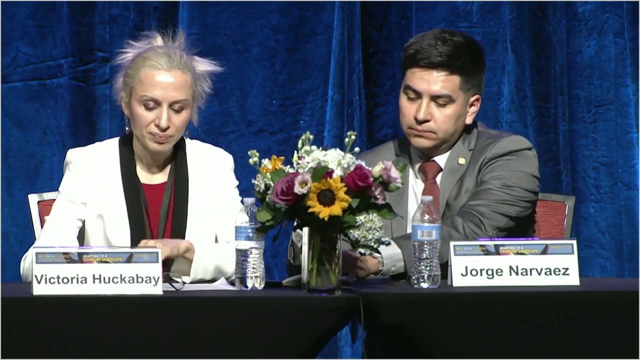 with the high-level waste that may result from reprocessing and how that is going to be dispositioned. So I think there is definitely a potential policy question there and definitely a regulatory challenge that we would need to take a look at closely. Great, If I could ask, Jorge, if you would want to add any to that response from DOE's perspective on legal barriers preventing the possession. 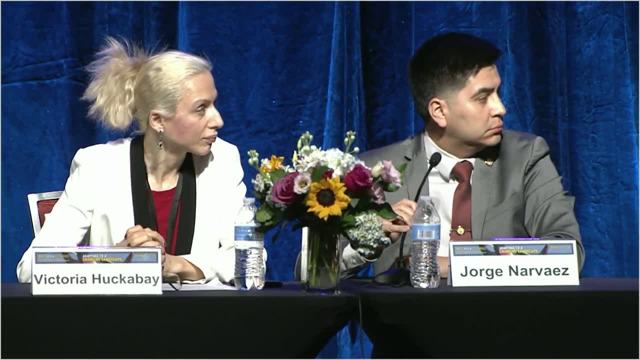 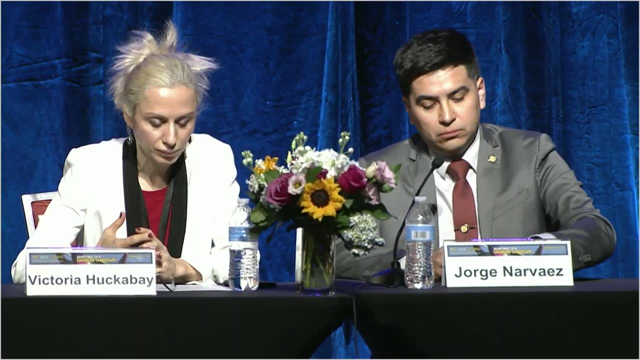 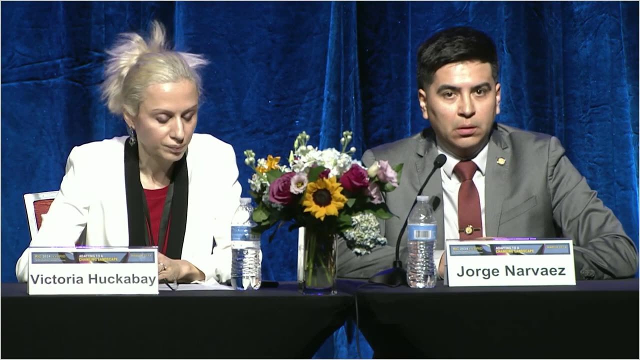 And maybe Victoria already touched into something related to this, And another question that was marked for your attention was: where is SMR, spent nuclear fuel, likely to end up being stored? What is the physical location? So, in regard to the first question, I cannot comment on any of the legal aspects. 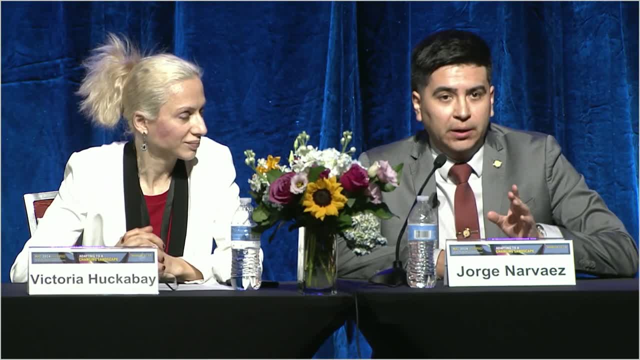 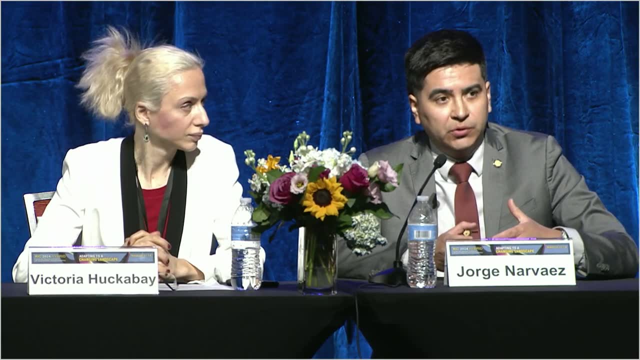 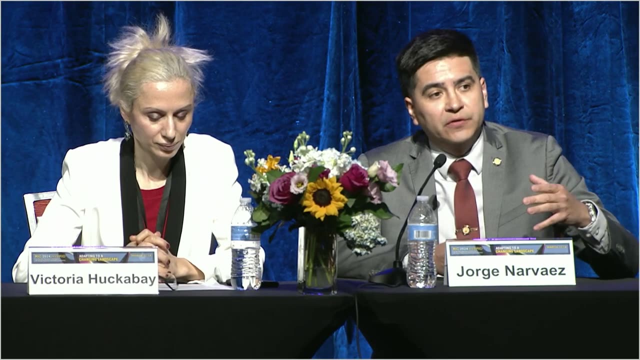 However, I can tell you that the Department of Energy is learning on the technical aspects that companies like Oklo and Shine are proposing, So we're trying to get an awareness of what's being proposed From the Department of Energy. there's another office in charge of reprocessing, research and development. 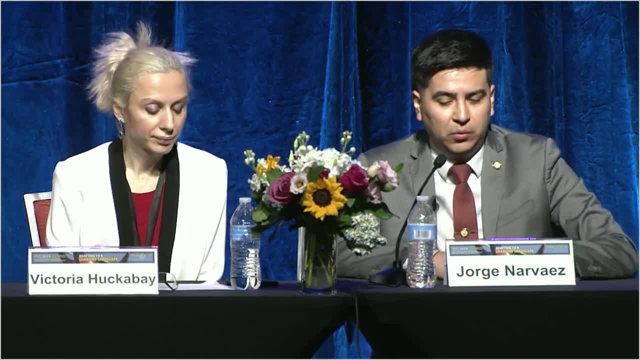 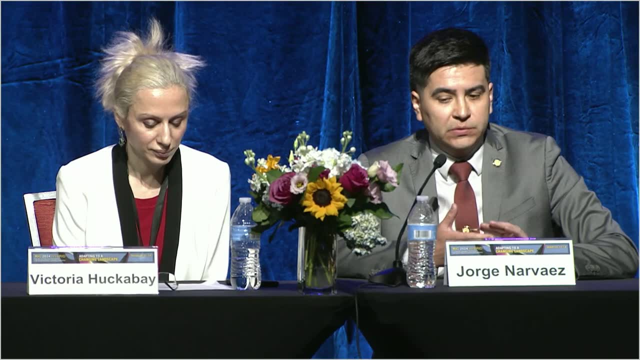 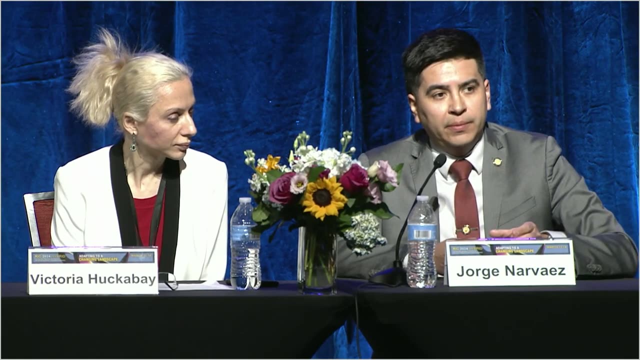 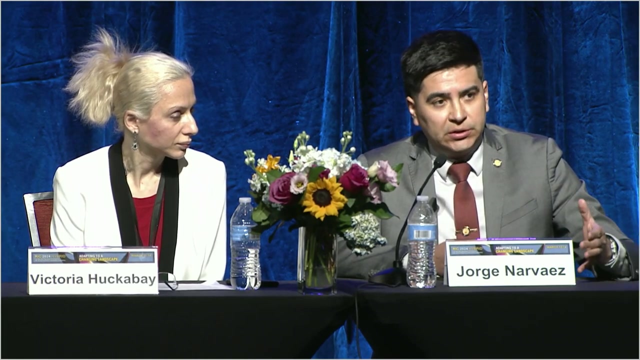 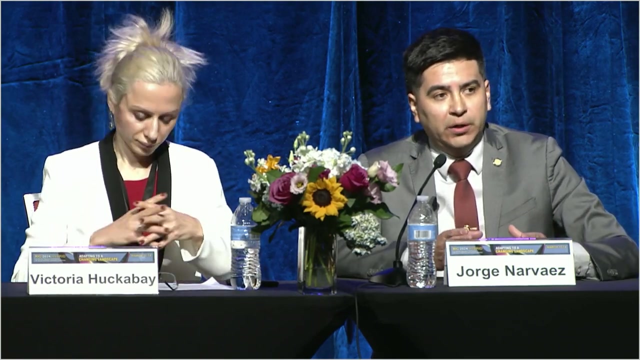 So they might be more informed in terms of what would that be. And then for the SMR question, I can mention That some of the vendors working near deployment or near demonstration have designed spent nuclear fuel storage as part of their reactor design. So for some of them you would see some facilities collocated in the reactor facility where they are planning on storing spent nuclear fuel. 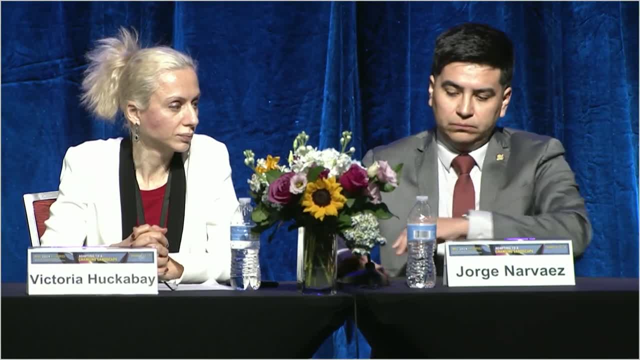 Thank you Appreciate that. I'm glad to hear that DOE, as we said earlier, like NRC, is already looking at the back end. I'm glad to hear that DOE, as we said earlier, like NRC, is already looking at the back end. 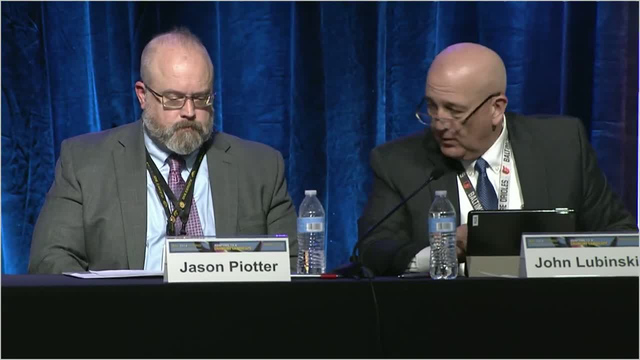 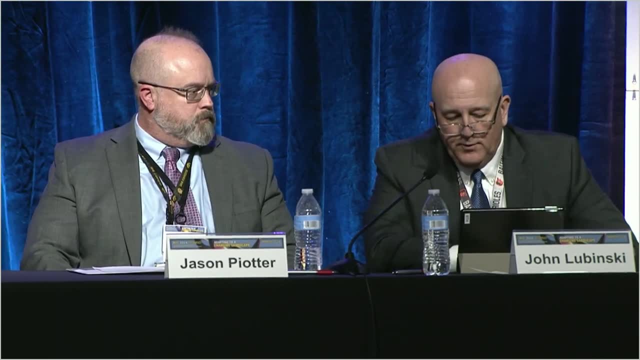 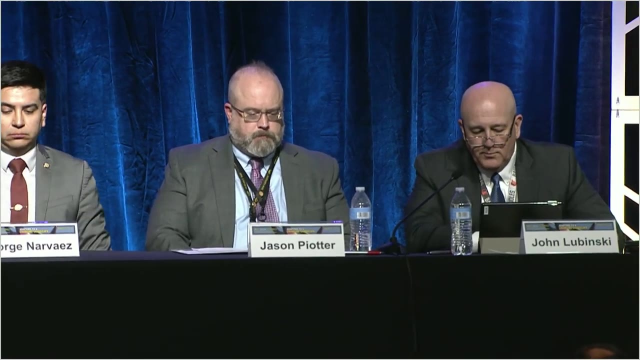 from any of those processes. So the next question I have was for Mr Donaldson, And I'll read the question verbatim: Since losing out on a loan guarantee over a decade ago, how much has Centris been able to bring down its cost per SWU so that you can commercially compete with the likes of URINCO or RONO? Yeah, So Centris has made several changes from the prior program run by its predecessor, USEC. Yeah, So Centris has made several changes from the prior program run by its predecessor, USEC. Now, at the time, USEC was the only one that was able to bring down its cost per SWU. 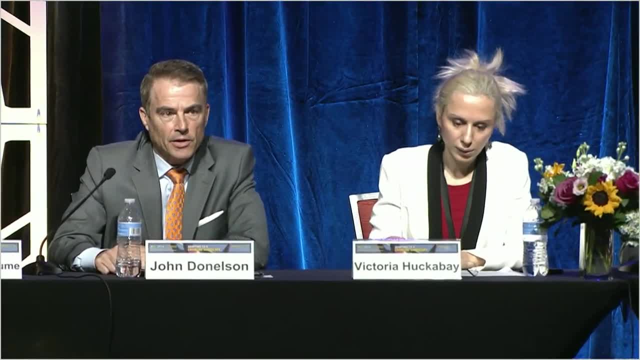 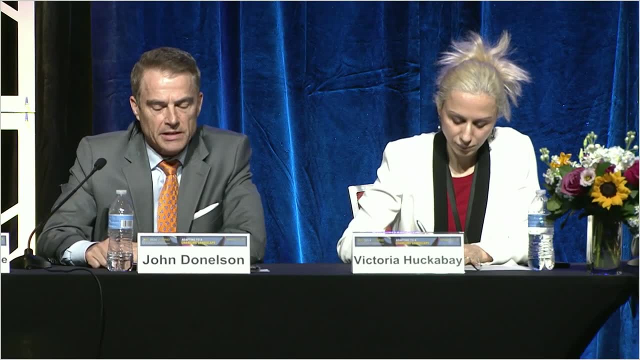 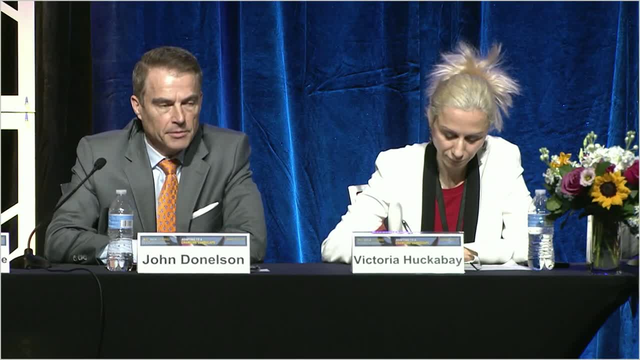 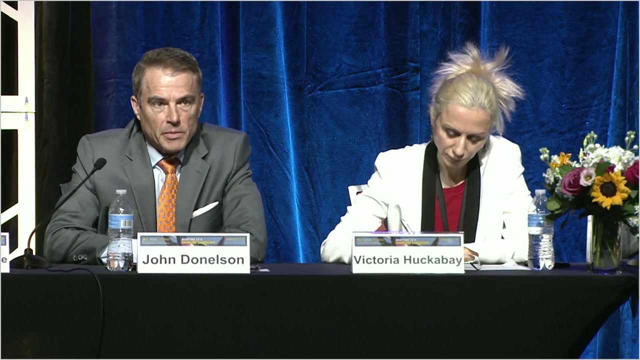 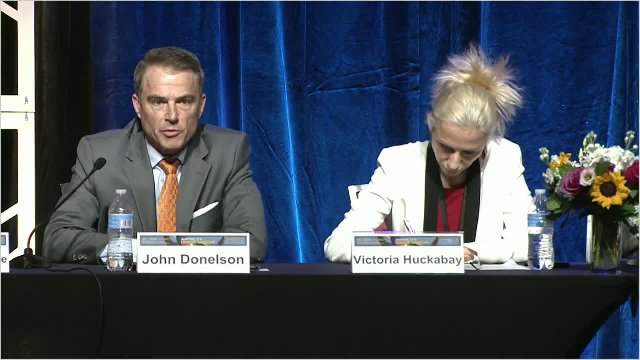 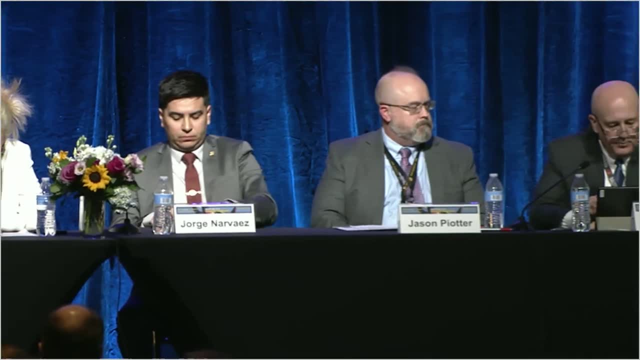 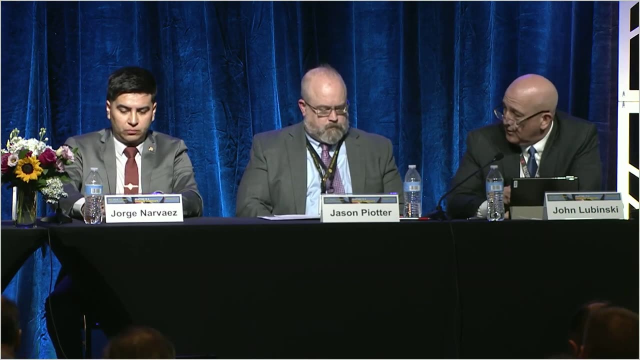 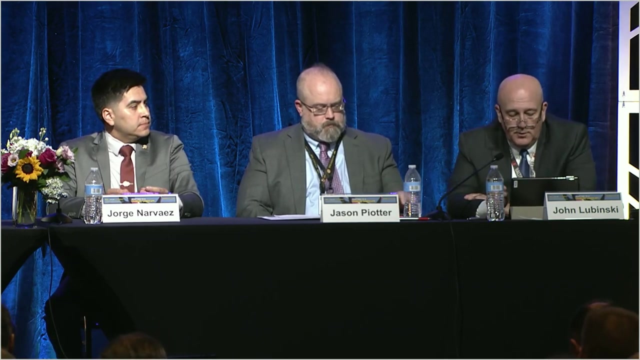 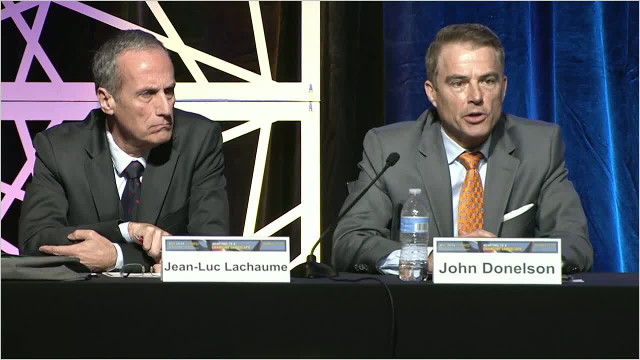 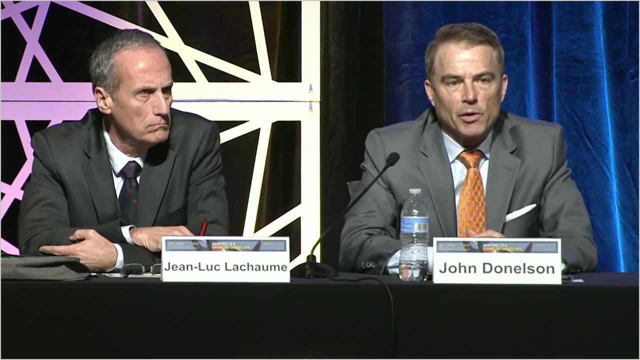 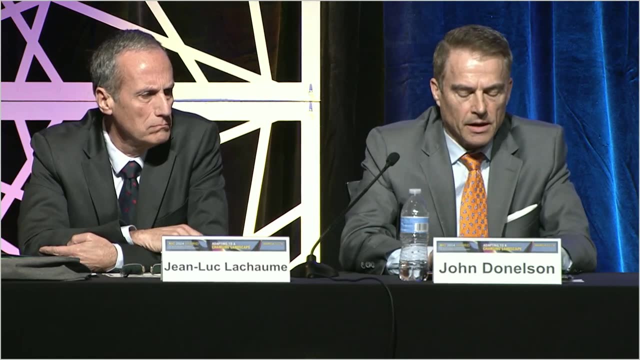 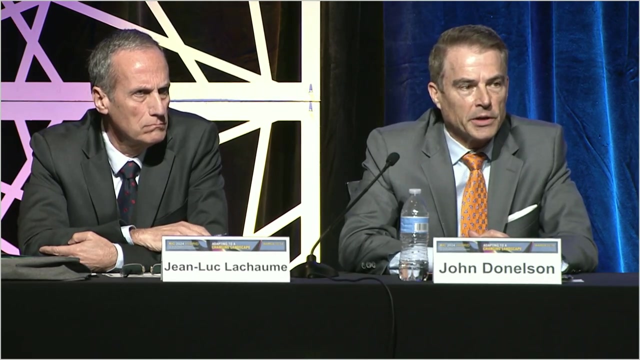 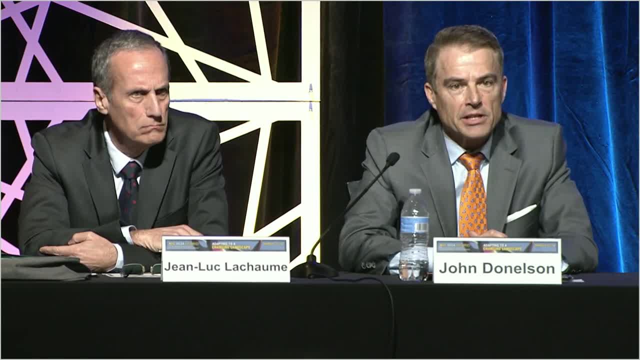 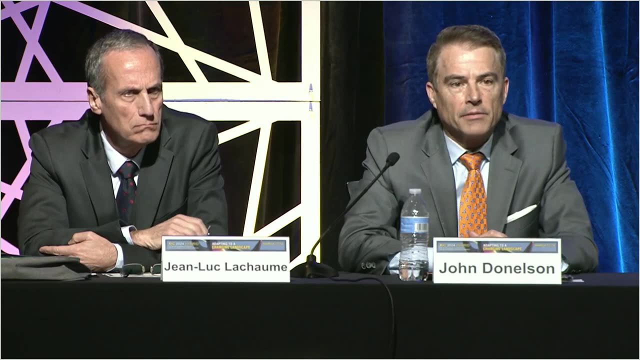 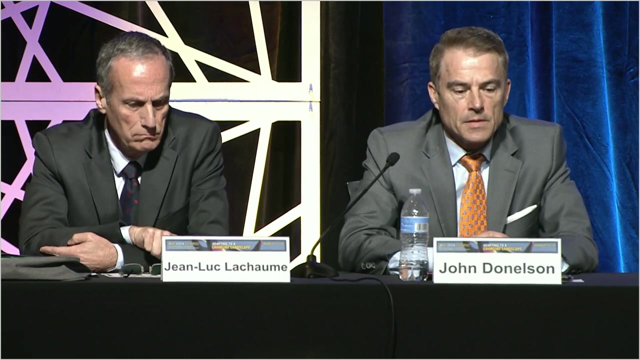 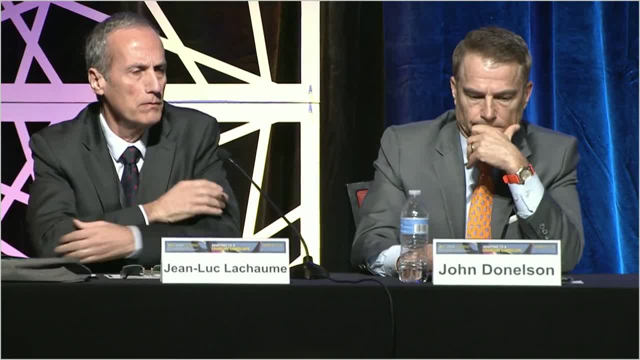 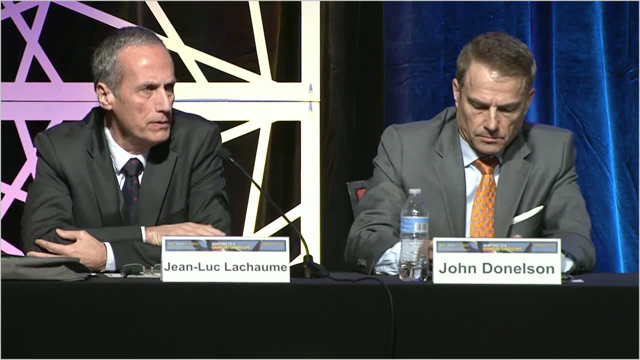 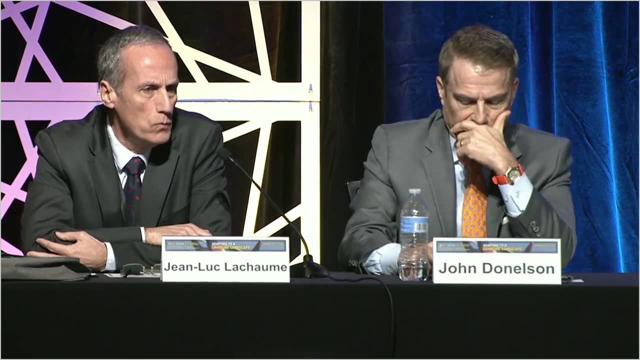 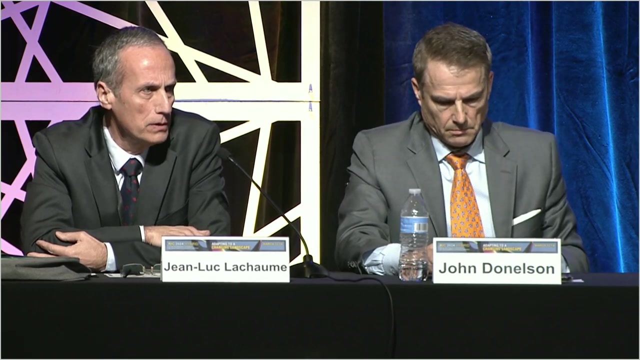 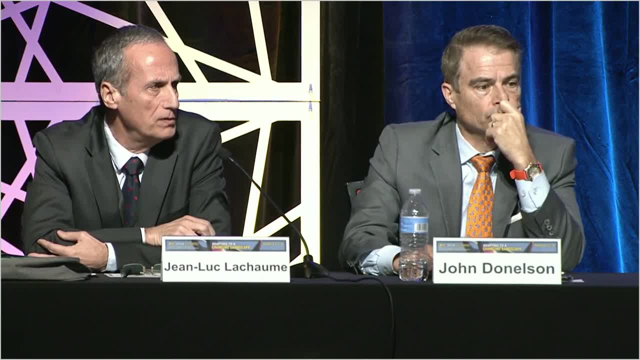 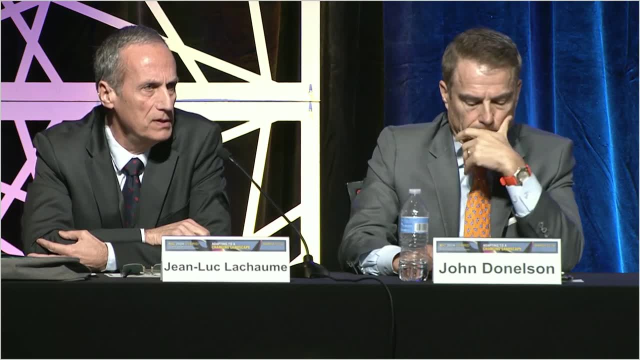 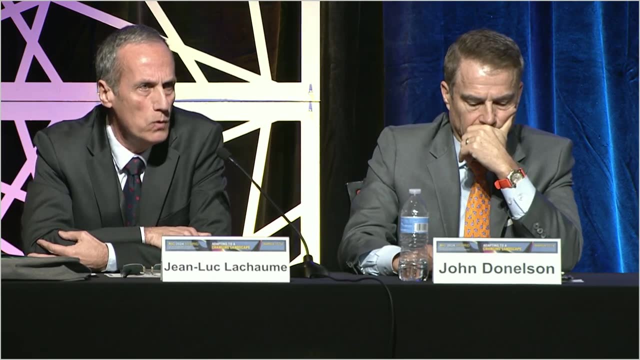 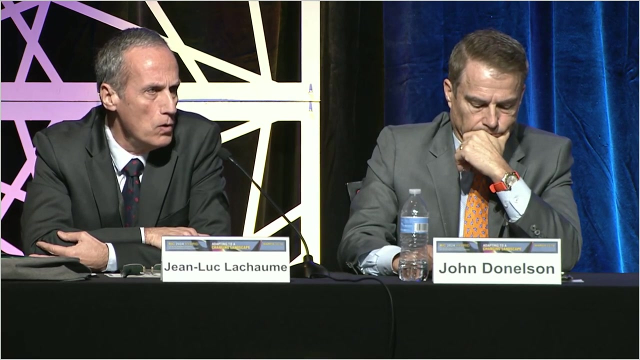 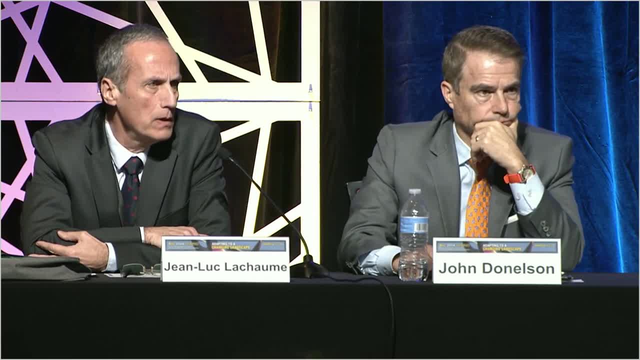 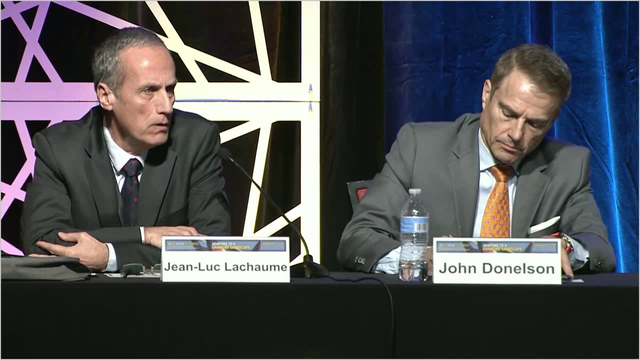 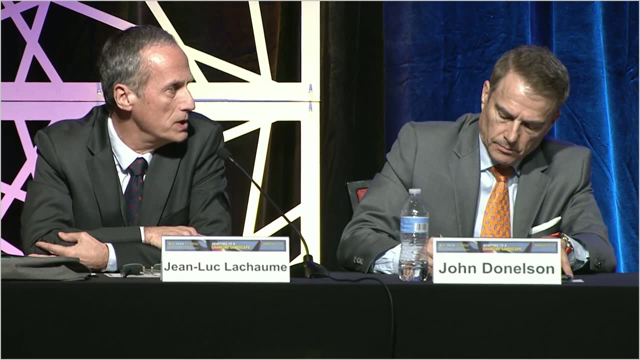 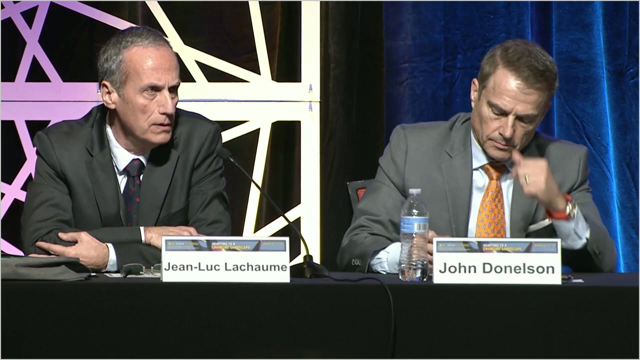 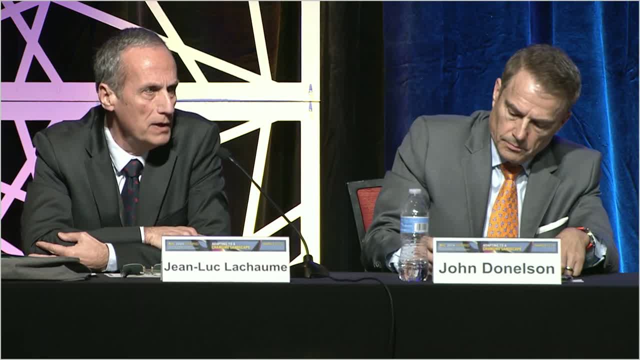 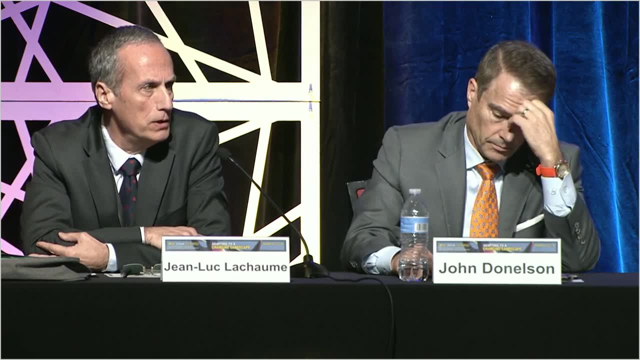 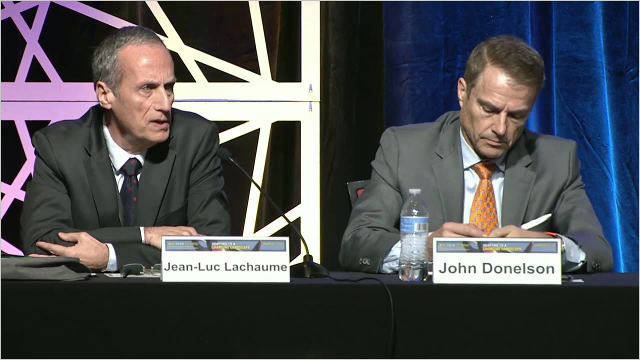 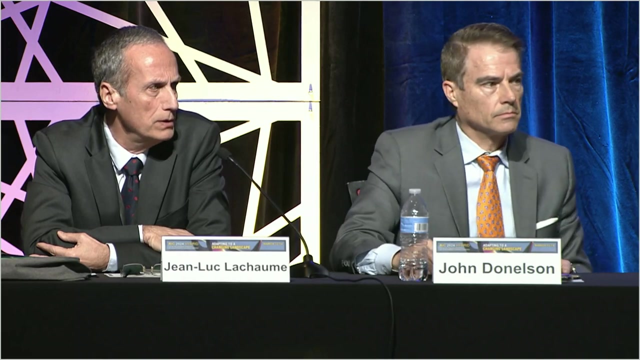 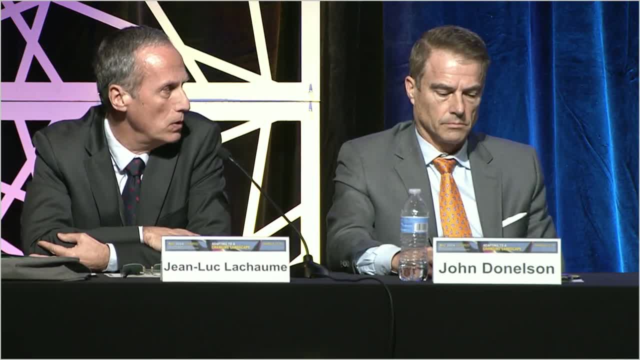 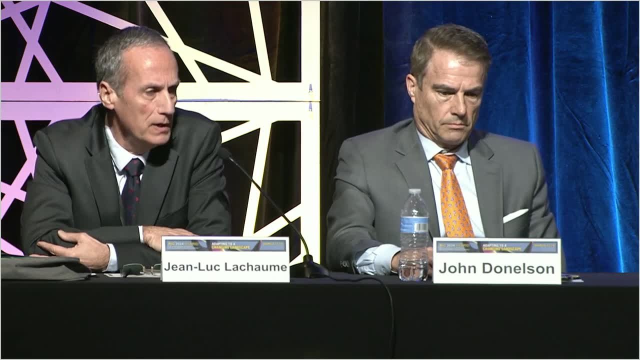 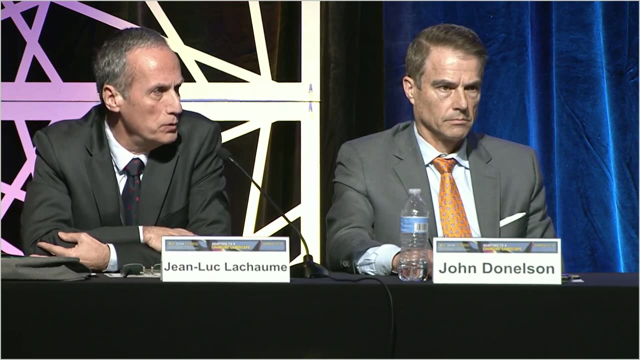 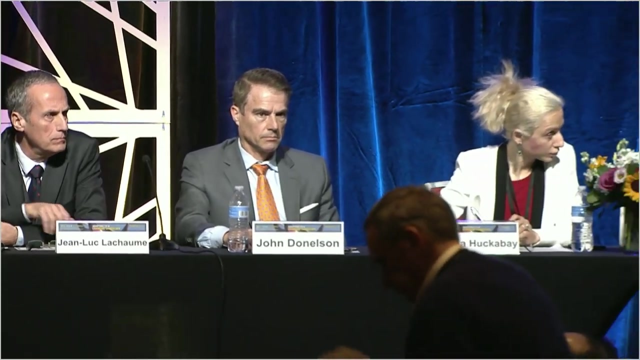 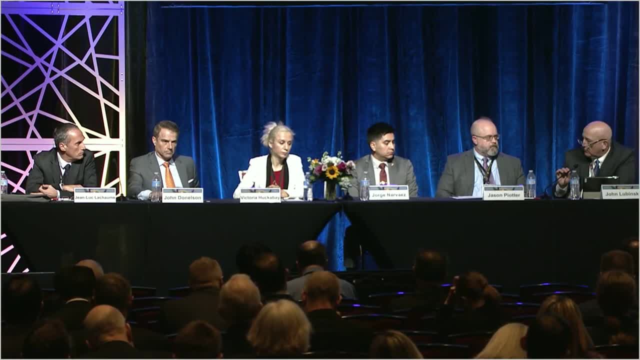 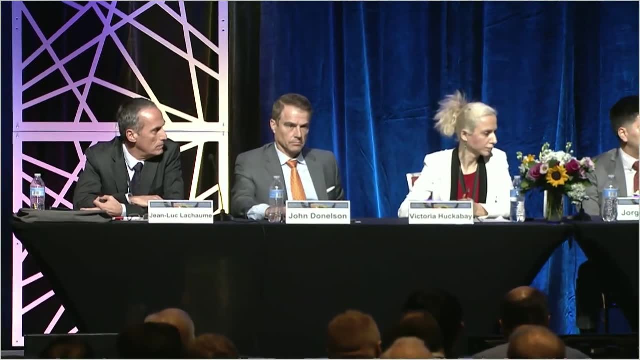 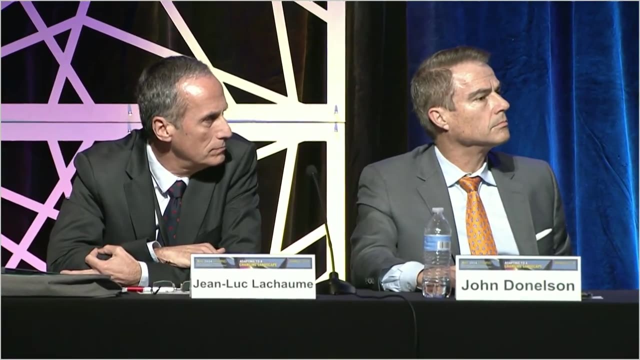 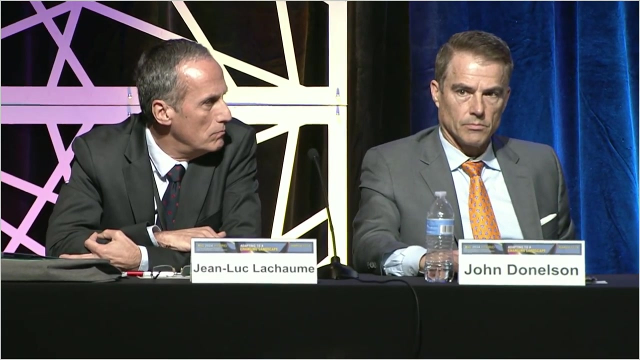 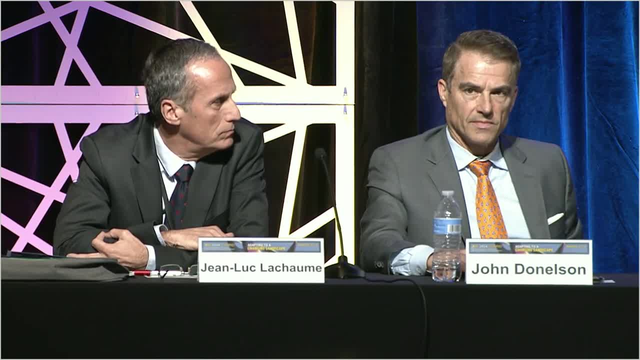 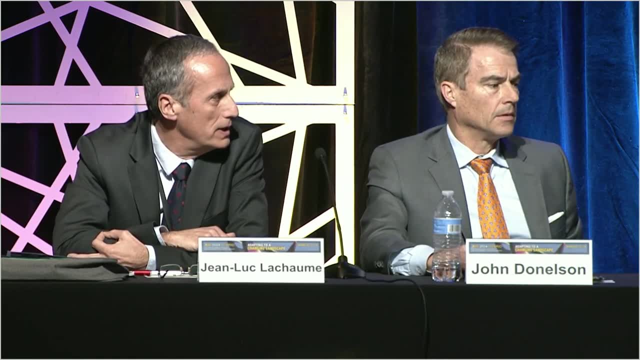 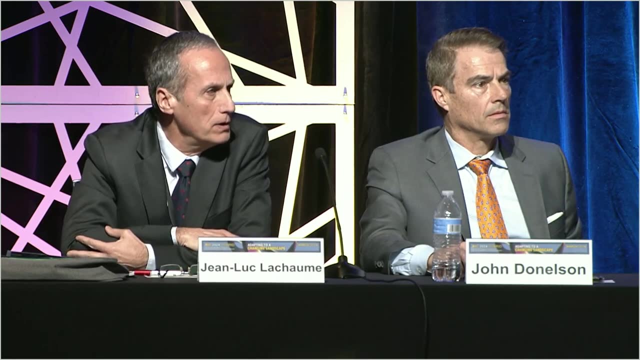 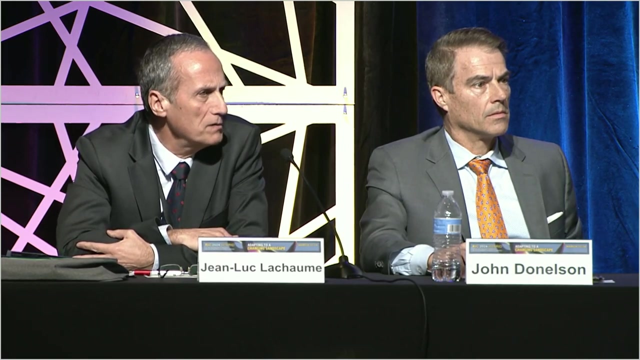 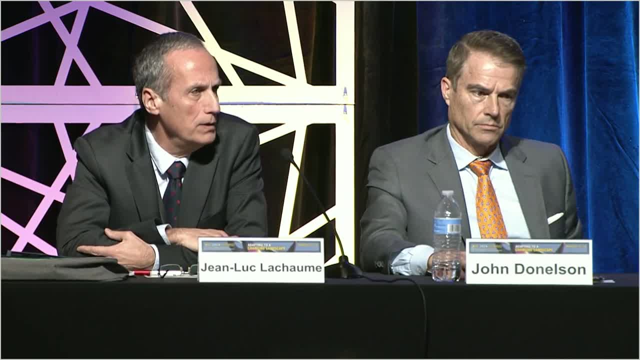 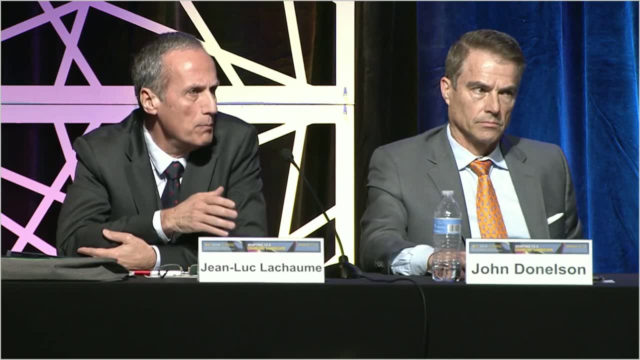 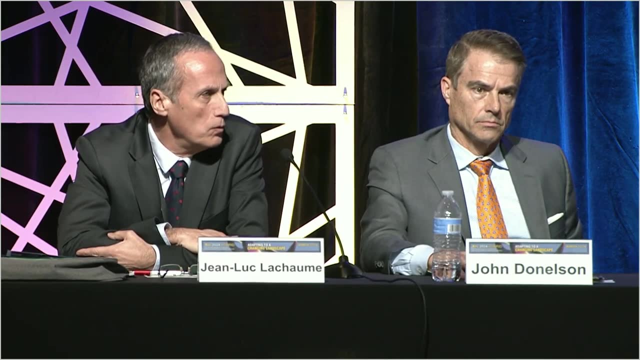 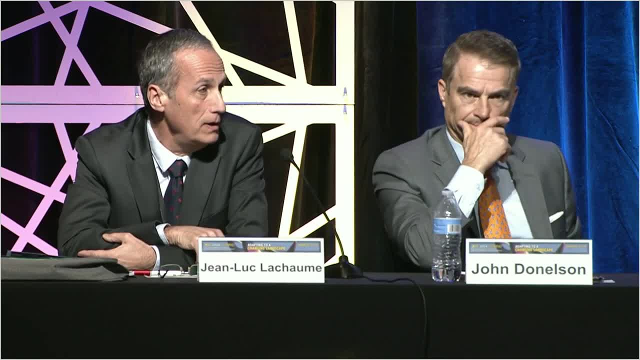 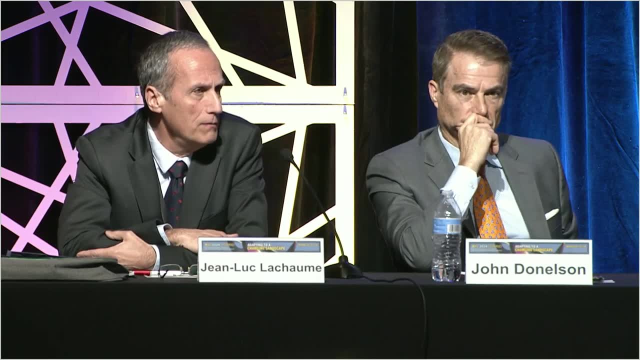 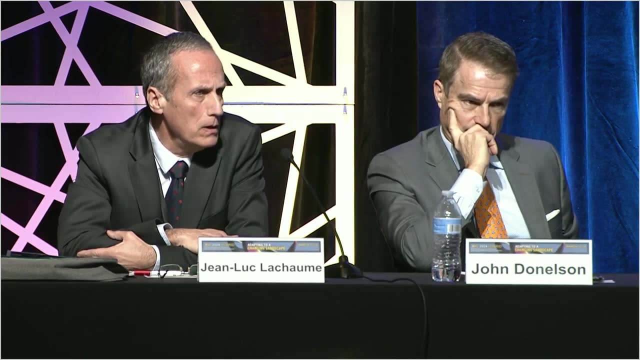 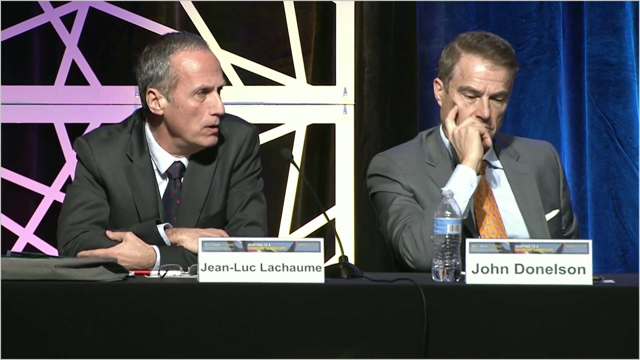 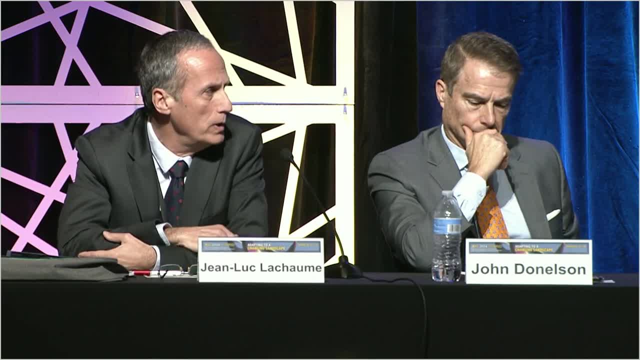 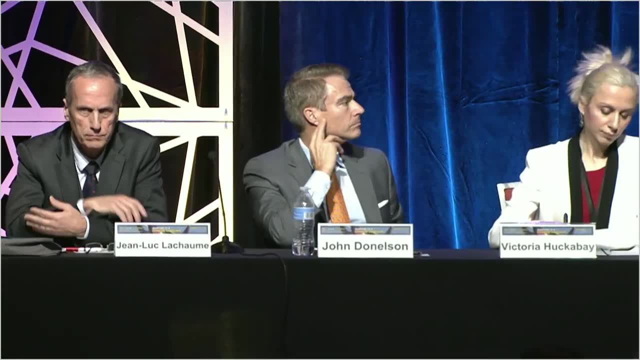 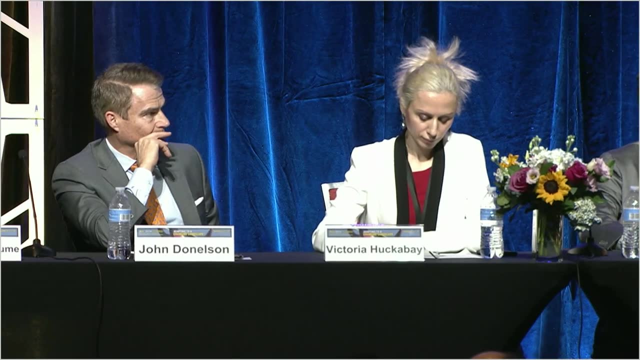 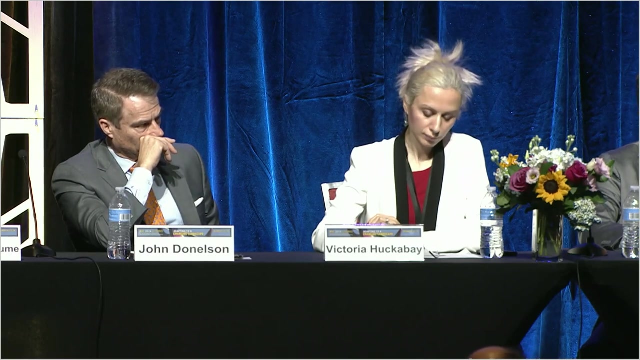 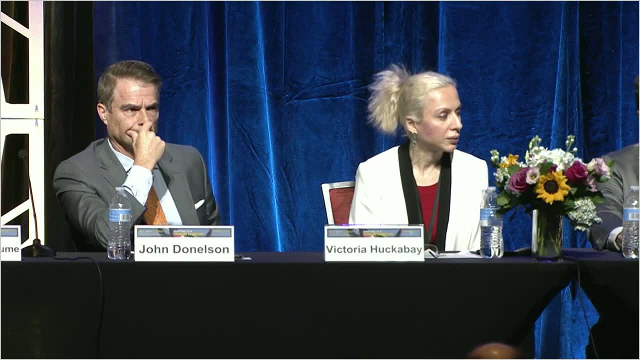 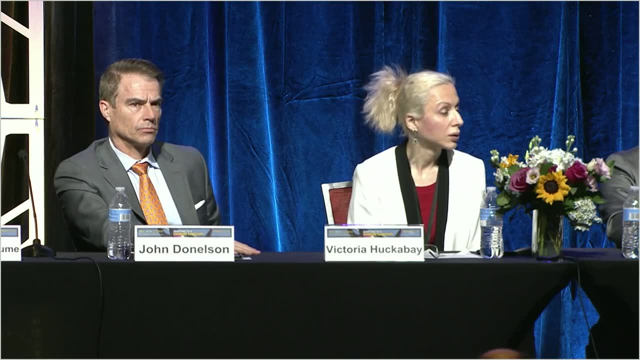 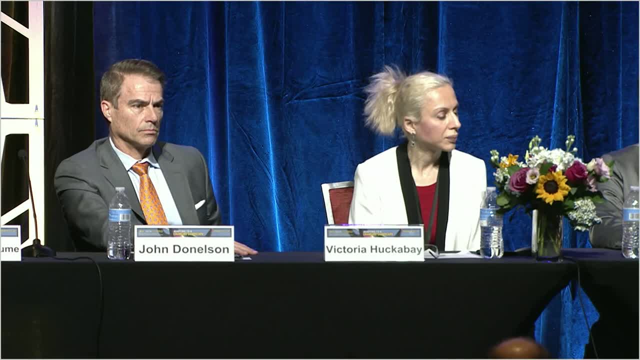 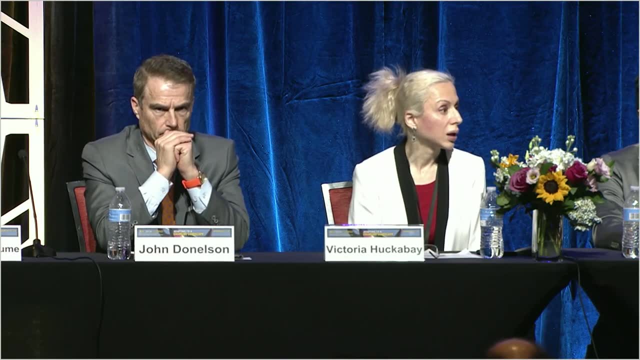 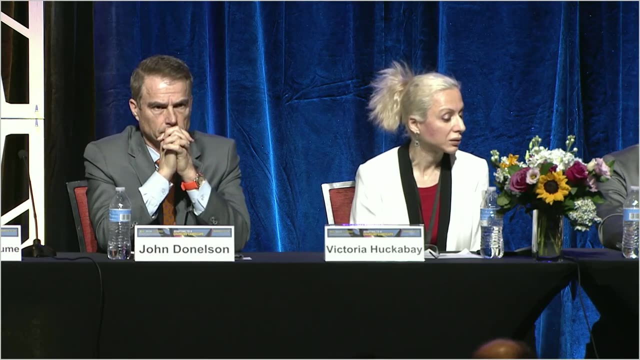 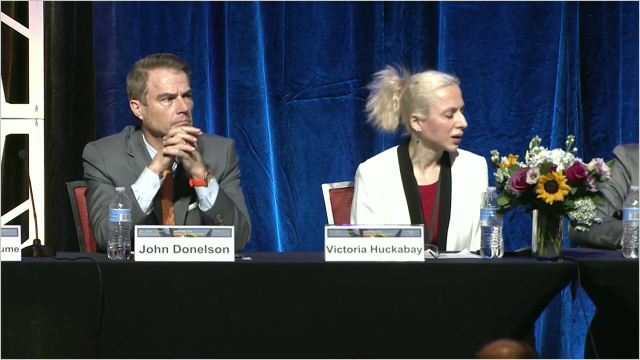 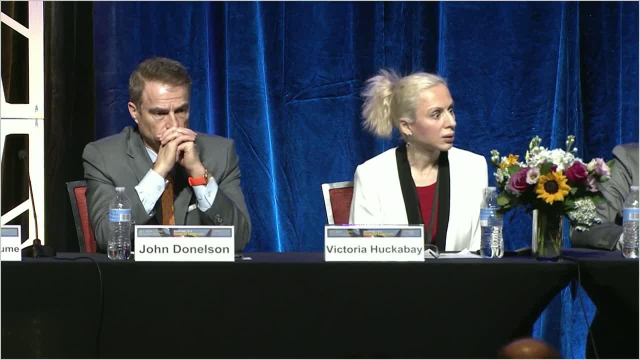 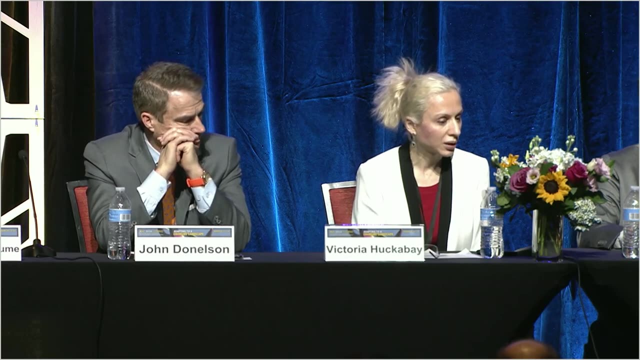 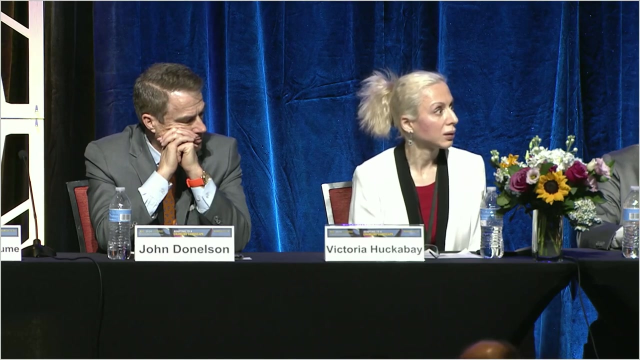 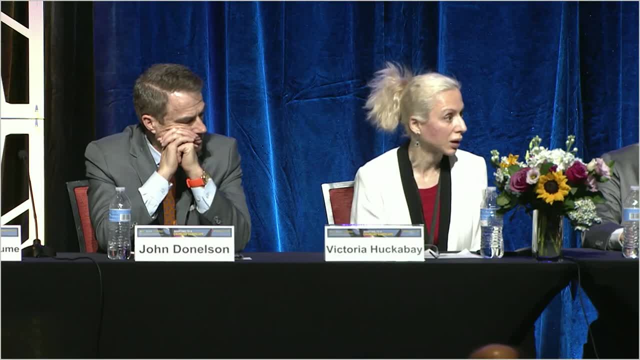 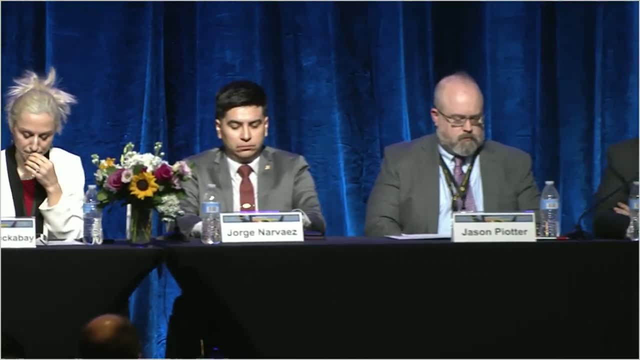 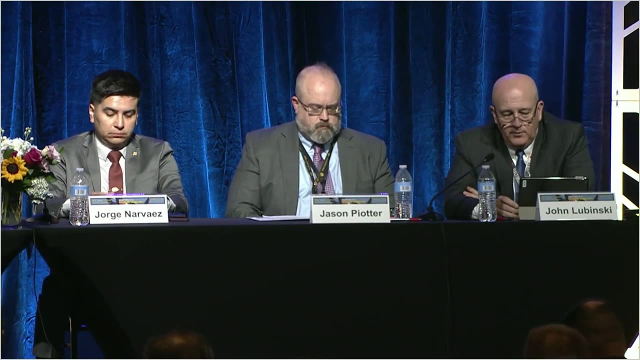 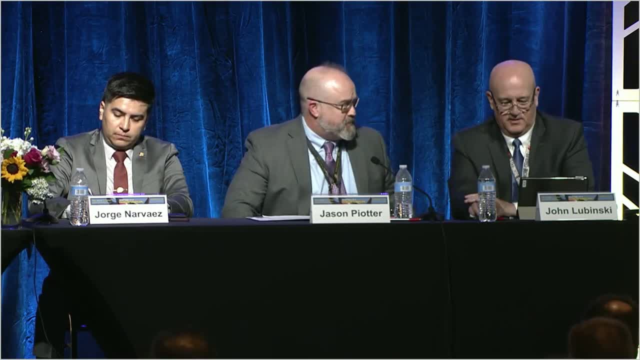 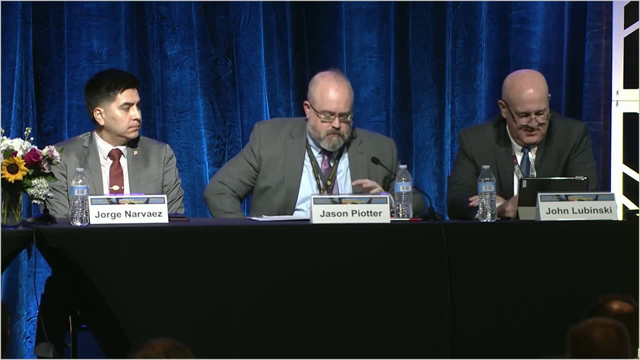 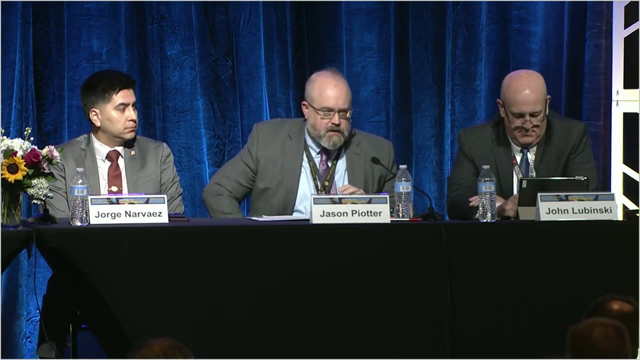 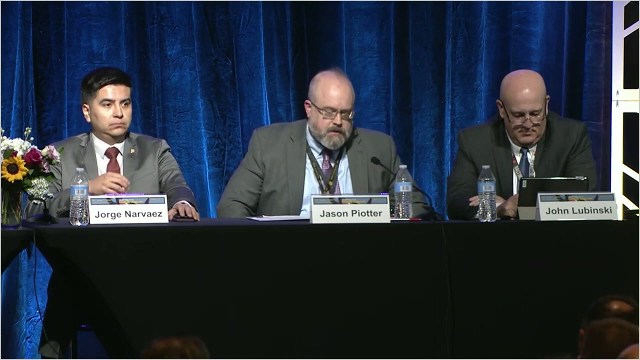 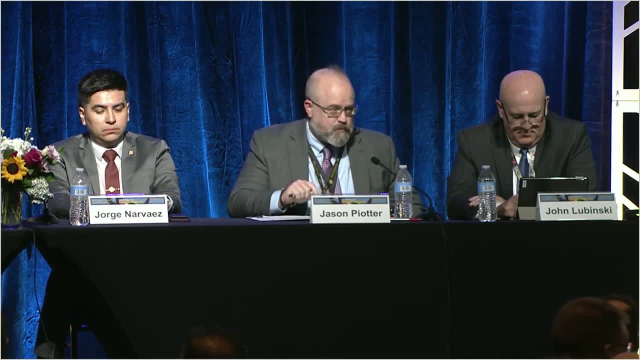 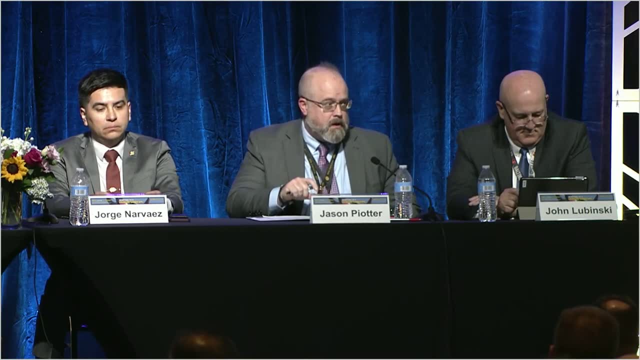 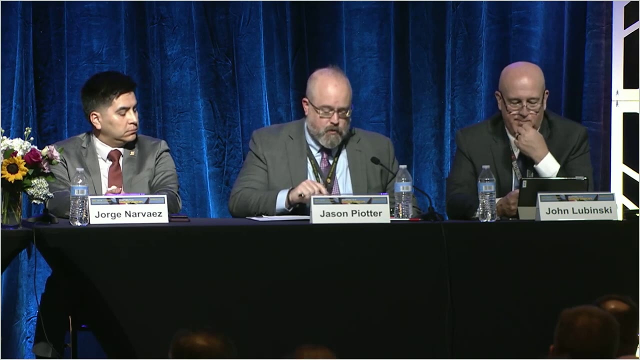 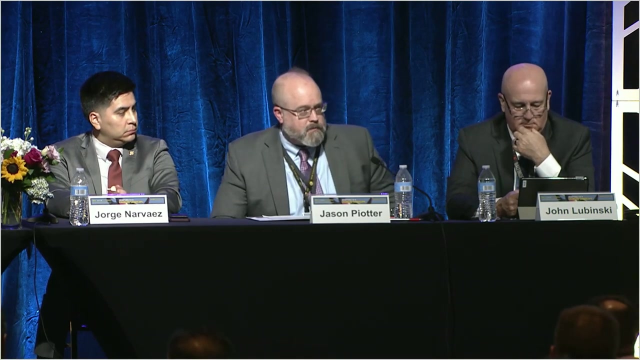 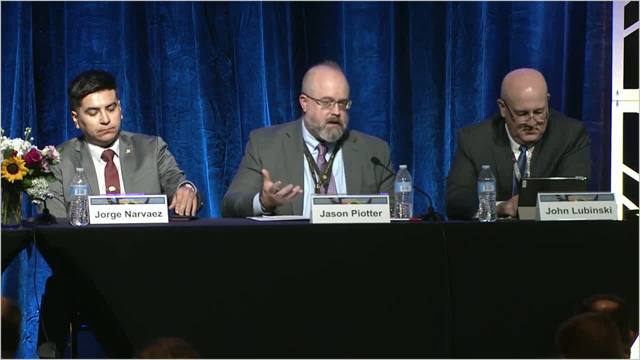 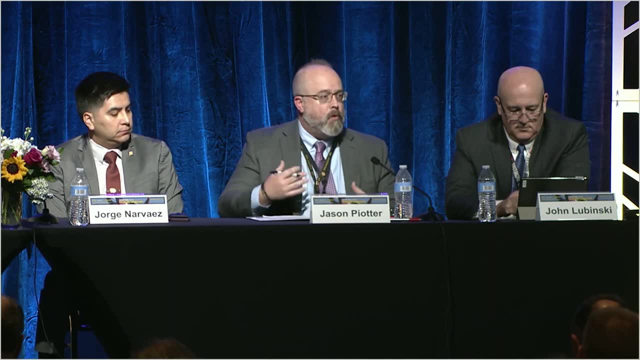 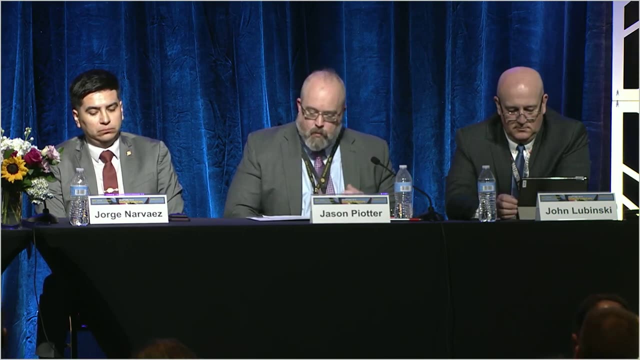 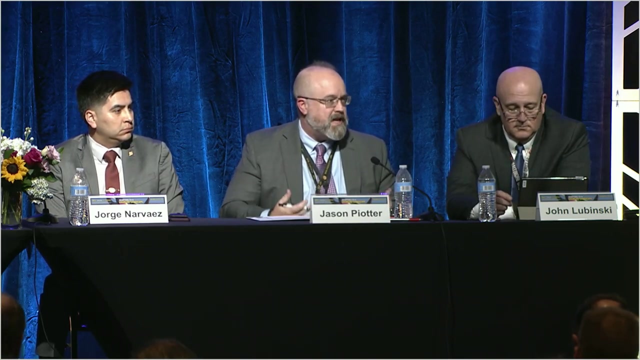 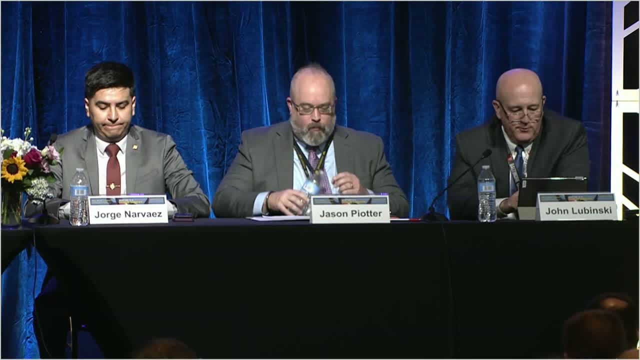 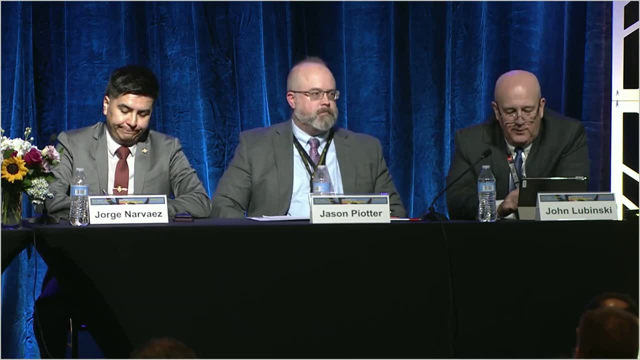 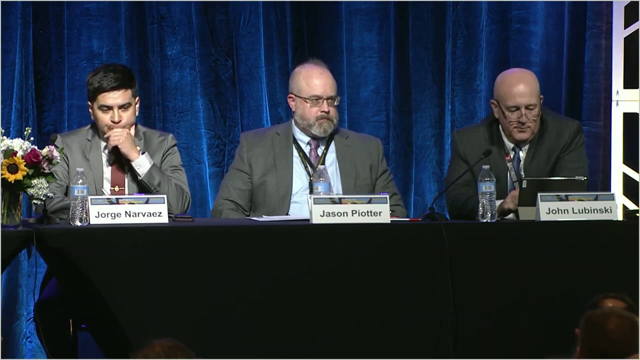 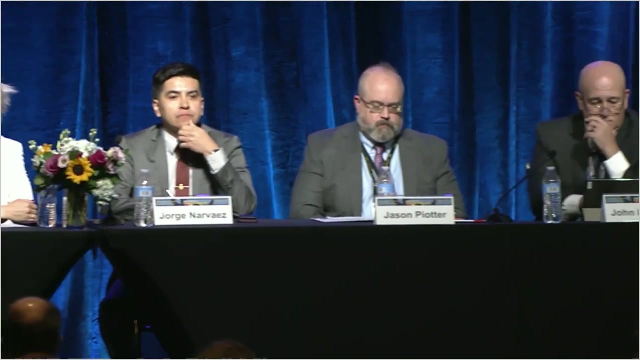 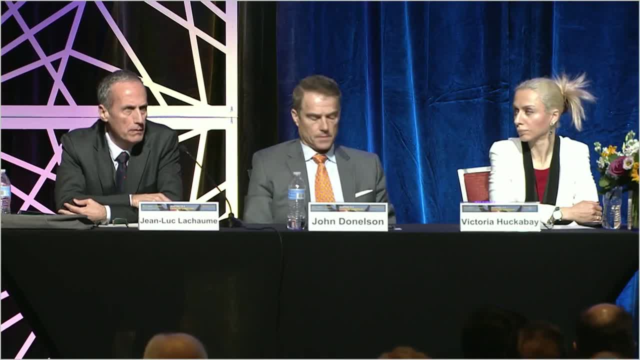 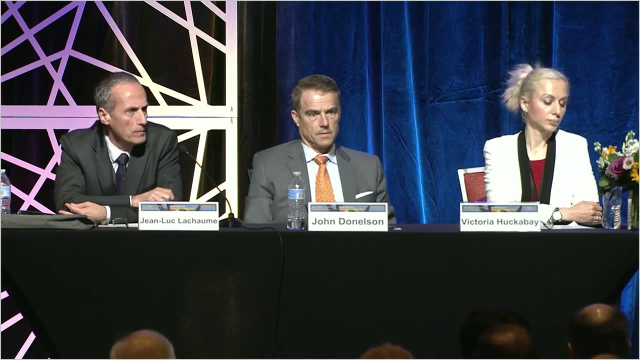 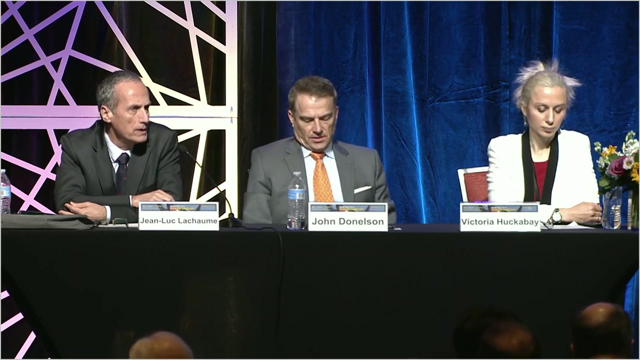 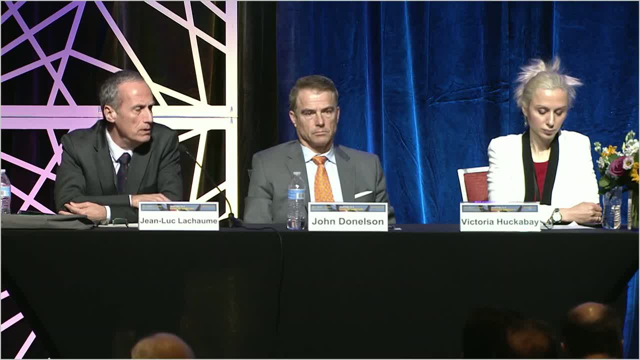 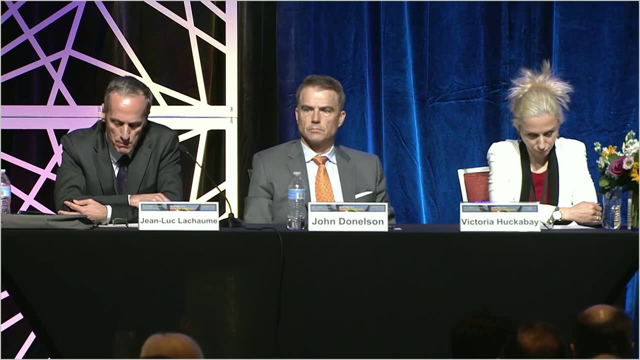 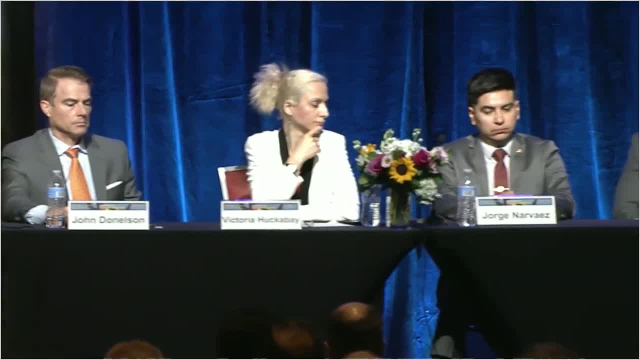 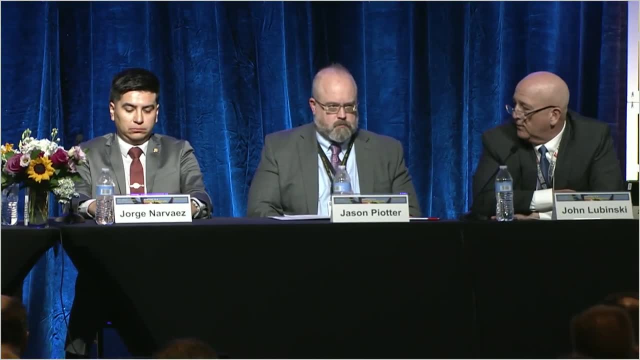 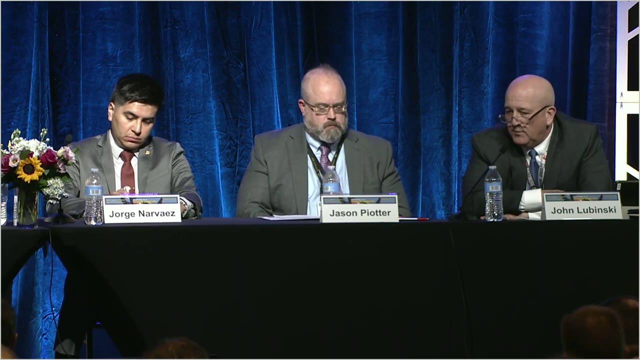 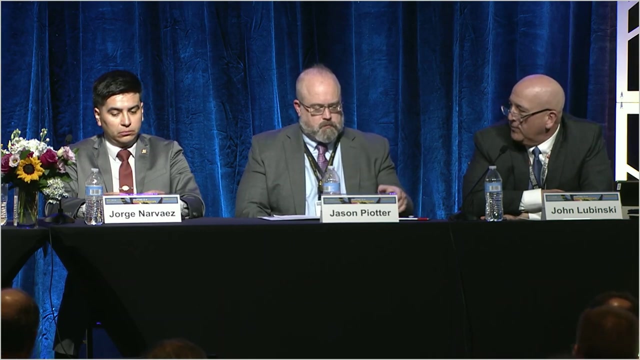 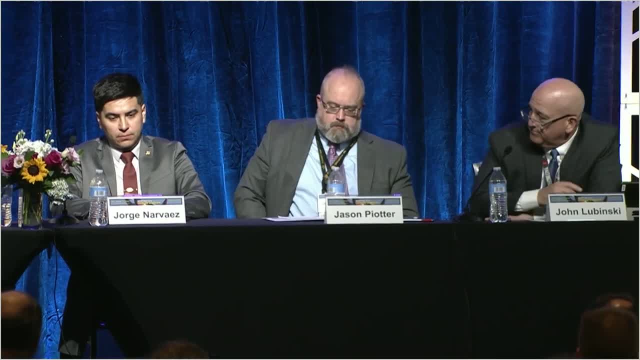 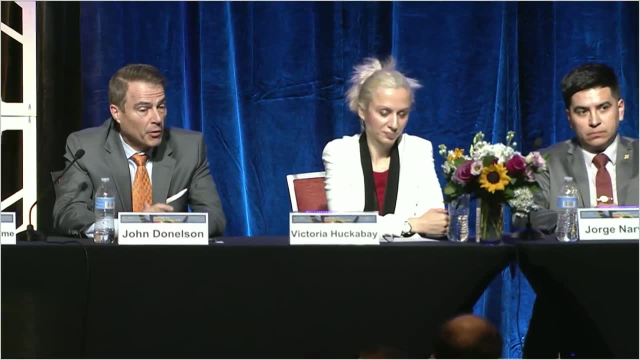 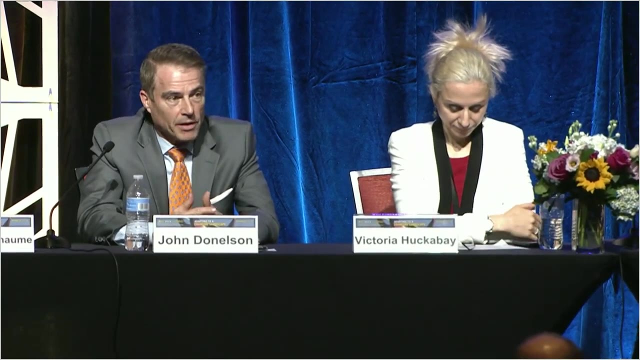 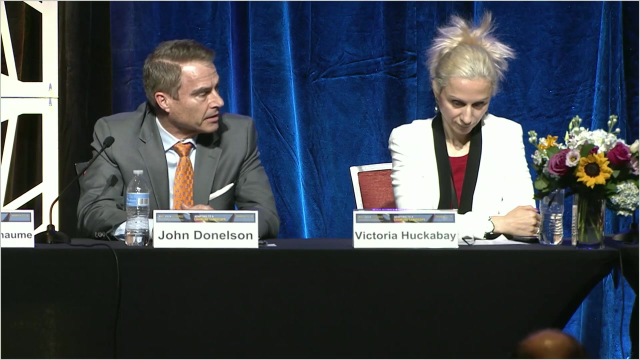 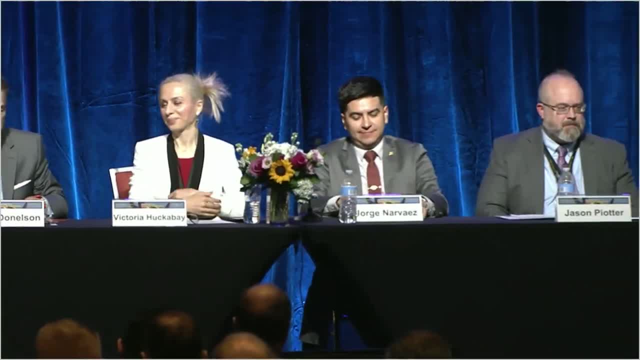 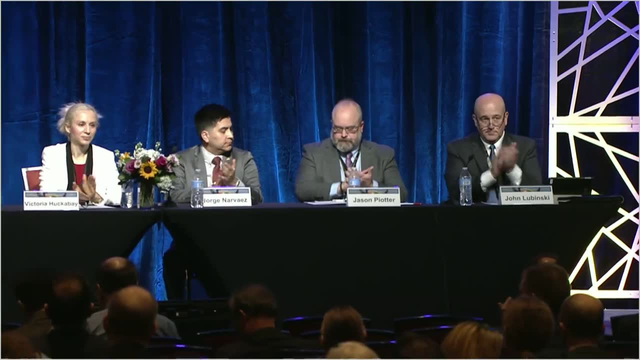 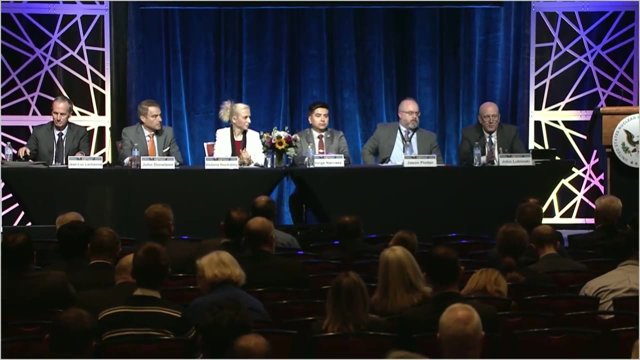 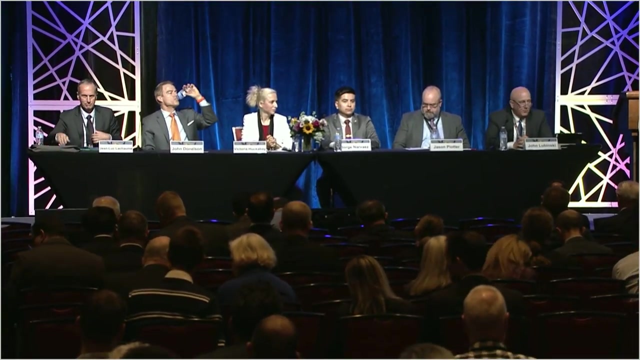